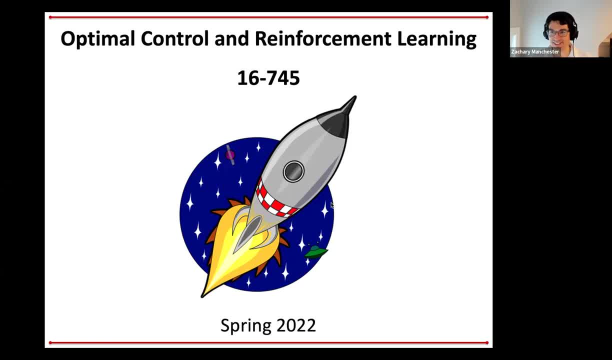 doing this from home again. So we'll see how this goes. So I guess as a just a quick logistical thing. definitely, it's kind of hard to see the. I can't see all your faces at once on the. there's too many people So it's hard to see the little hand raise thing. So 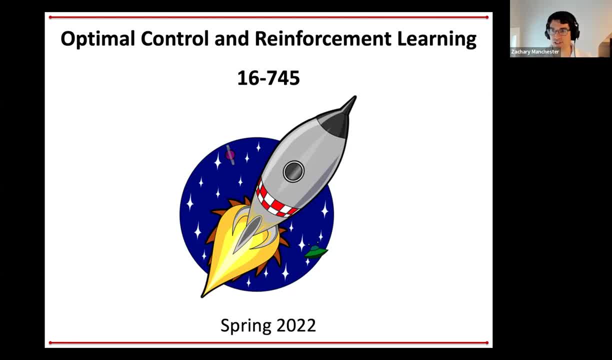 if you've got a question or something to say, just for now, just unmute and speak up, And when you do that, I'd appreciate if you turn your camera on when you're talking, just so I'm not like staring into the void and it'd be cool to see who's talking. If that becomes a problem with 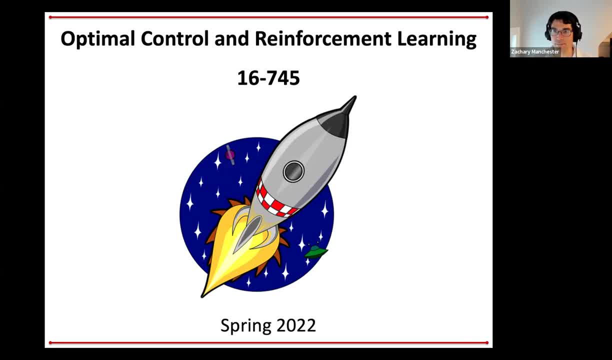 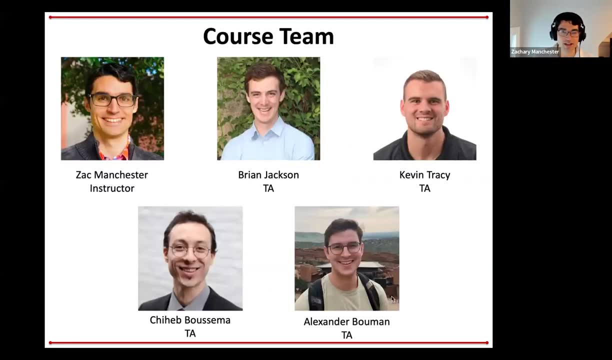 too many people trying to talk at the same time. then we'll figure something out with the hand raise thing or something like that, But for now, yeah, just unmute and then speak up, and that should be fine. A couple quick logistics things. I guess that was one. So the next step is: 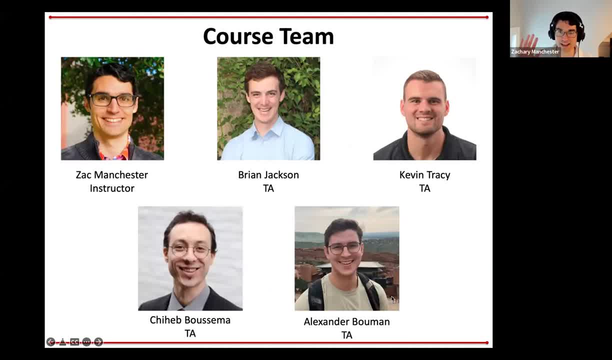 the course team we'll be dealing with this semester. So I'm Zach, You can call me Zach. I'm an assistant professor in the Robotics Institute and I lead the robotic exploration lab And our research is in optimal control. As you might expect, we do a lot of stuff with numerical 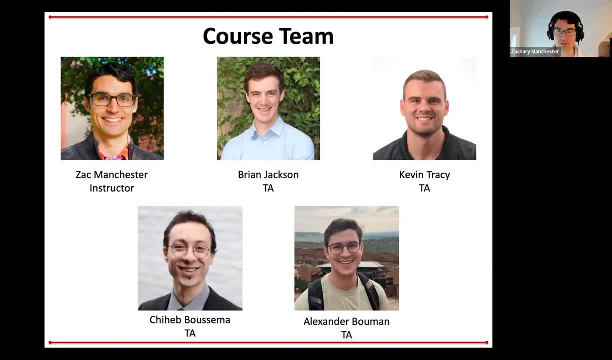 methods and kind of very applied flavor of optimal control, which is basically what you're going to get in this class. So we're it should be fun. We can talk about our research too to some extent. if you guys are curious, don't hesitate to ask myself or any of the TAs. 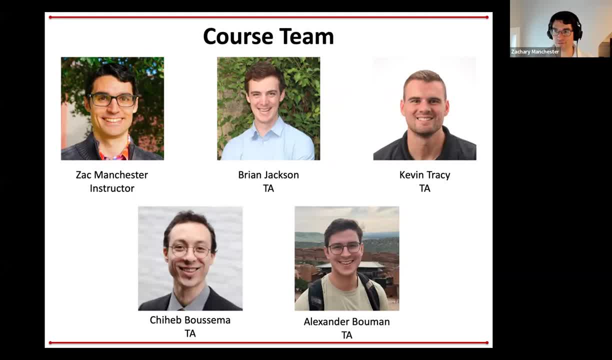 Brian Jack Jackson, one of my PhD students, who was the TA for this course last year and did an awesome job, will be kind of the lead TA this time around again. So you guys are in good hands there. And Kevin Tracy, another one of my PhD students, took the course and is TAing it this time around. 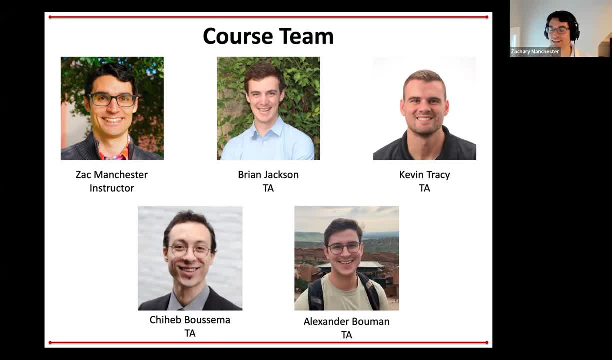 Actually, why don't you guys do a quick intro if you're thrown here? Sorry, sorry for that. Brian, you want to say hi real quick. I'll let you guys introduce yourselves instead of me talking about you, which is weird. 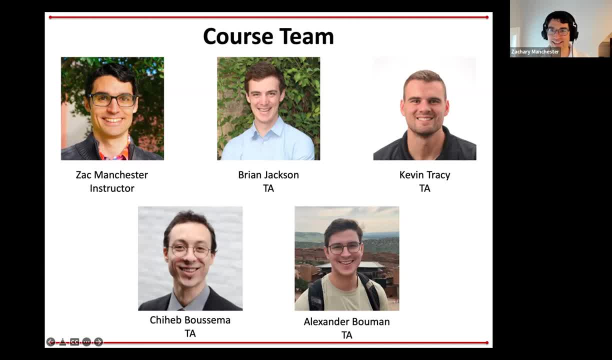 Oh, we can't hear you. How about me? Yeah, there you go, You can hear me now. Yeah, Okay, Hey, yeah, Hey guys, My name is Brian. Like Zach said, I TAed this course last year. I'm a fifth year PhD student and my research is in like applied numerical methods for optimal control. 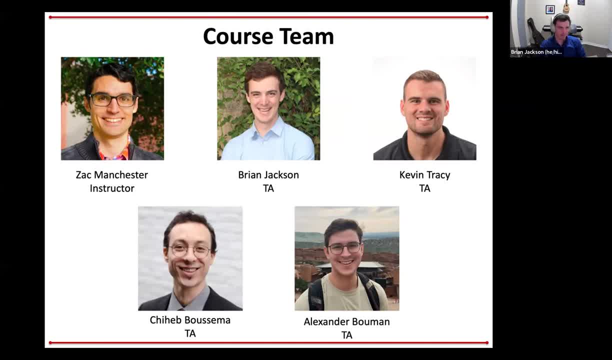 So, yeah, here to help and don't hesitate to reach out with any questions. I thought anything class related, And then Kevin's next up. Kevin, you want to say hey Sweet, Hey guys, I'm Kevin. I'm a second year PhD student. I do a lot of stuff pretty similar to Brian, optimal control for aerospace stuff. So if anyone wants to talk aerospace stuff, always let me know. 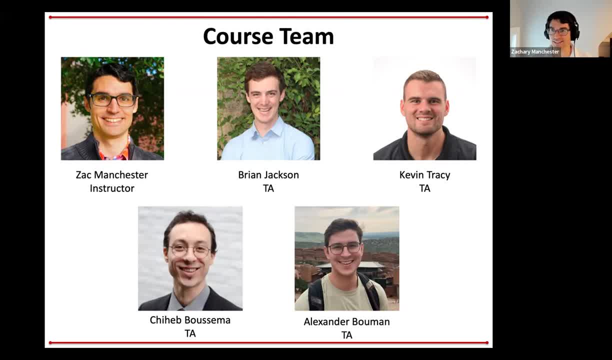 All right. And then Chihab, who also took the class last year. Is Chihab with you here? Maybe not Okay, We'll skip Chihab. And then last up, Alex, who also took the class last year and has been doing work in the lab with us. Want to say hi. 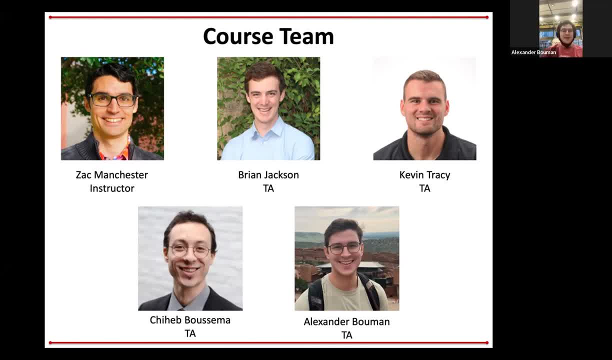 Hi everybody. Yeah, I'm a second year master's student in mechanical engineering And I work with Zach on quad motor control stuff, All right, Cool. So that's your course team for the semester, And don't hesitate to reach out to any of us anytime. 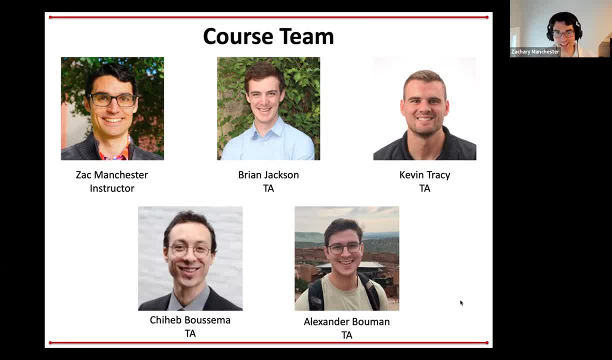 So okay, So now I'm going to kind of like lay out a little bit of kind of the state of the art in the field and some of the applications we're going to talk about later in the course. So this is sort of things you can look forward to and kind of the direction we're going to go and where we should get you to by the end of the semester. 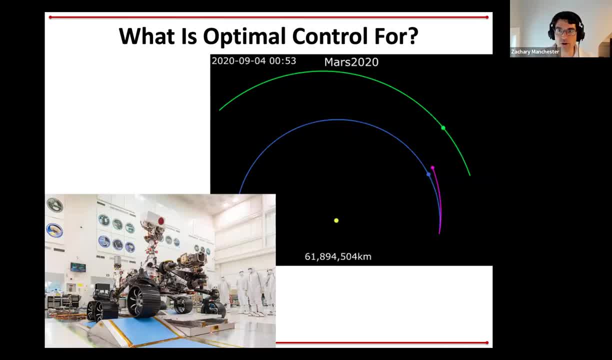 So first off, kind of what is optimal control for and what are people using it for right now? So in originally, the earliest applications For optimal control, where a lot of it was originally developed, is in the aerospace field, which my lab still works in quite a bit. 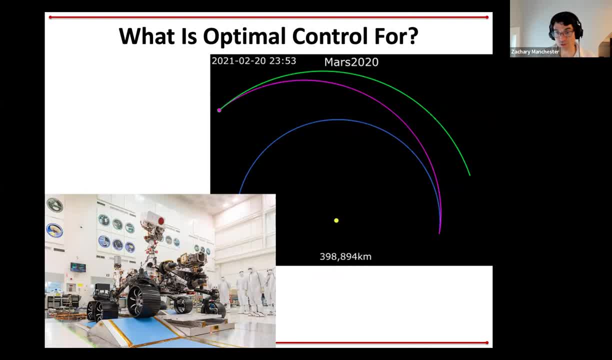 And originally this was developed for solving for rocket trajectories for launch vehicles- starting in kind of the 50s and 60s- And then for computing things like today, how do you get to Mars, for example. So, like, designing the trajectories to fly a spacecraft from the Earth to Mars is done with the sort of trajectory optimization methods that we're going to talk about in the class. 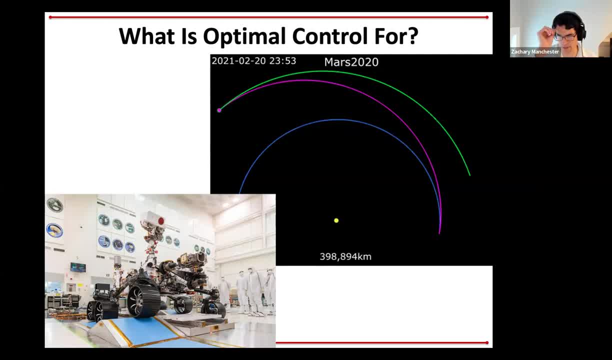 Specifically this gets done With nonlinear trajectory optimization methods. often direct co-location is kind of the method of choice for this stuff at places like JPL. So we'll talk about this a little bit And this is sort of one of the current applications and historically one of the main drivers for a lot of the developments in this field. 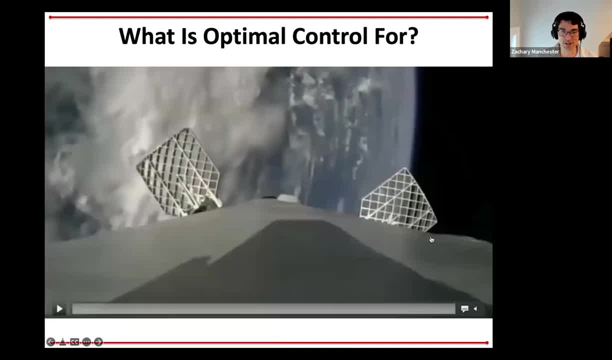 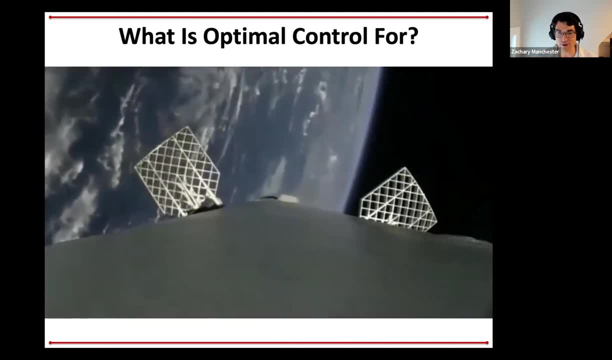 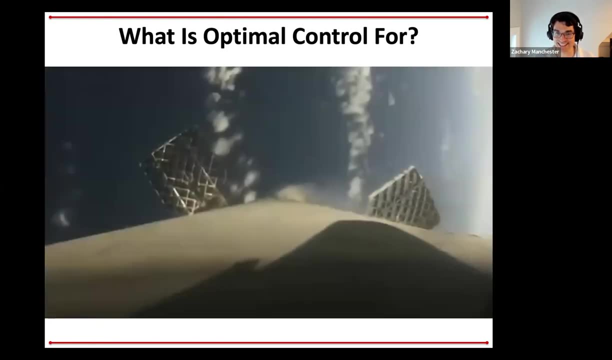 So some more sort of state of the art fun. current stuff that probably most you're aware of is SpaceX, landing rockets and more aerospace stuff. Does anyone know how this gets done? Anyone who isn't one of the TAs or isn't in my lab. 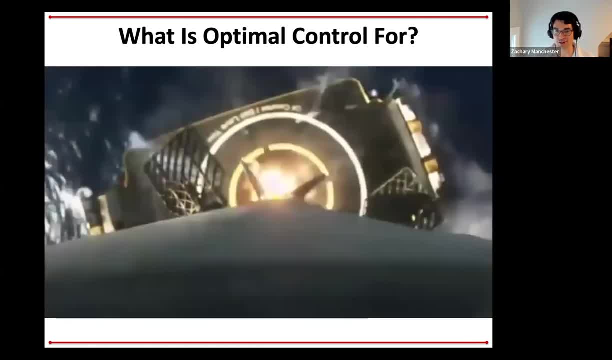 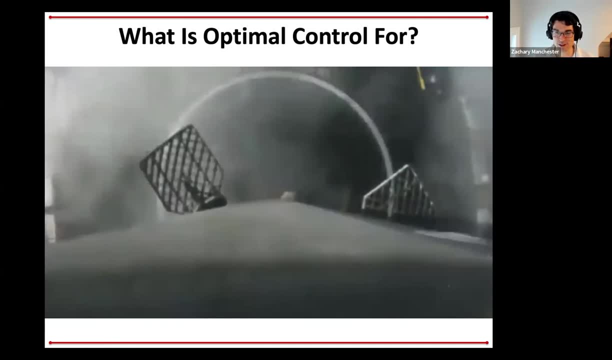 Does anyone have any thoughts of what sort of control methods are used to make this stuff happen? Land a rocket on a barge in the middle of the ocean- Pretty awesome. Has anyone followed this stuff at all? Nobody. No one has any thoughts. 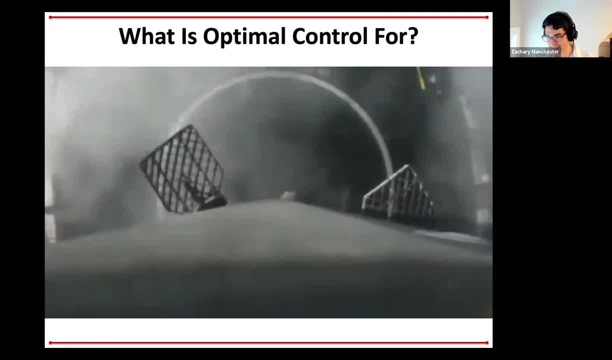 Take a guess, Someone take a guess, I'll guess. I guess that it's some sort of model predictive control. Yeah, So, as a lot of kind of the stock stuff is these days, this is convex model predictive control with a lot of kind of secret sauce and robust low level tracking control stuff. 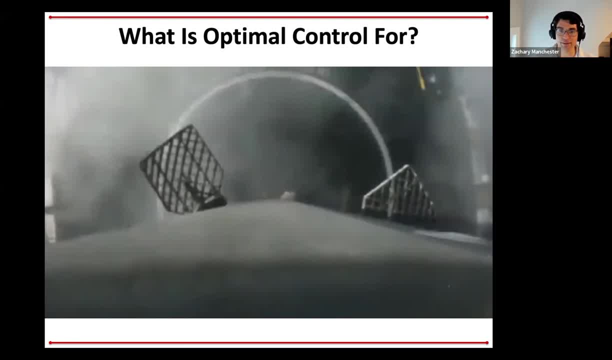 There's been actually a lot of progress in this sort of what's called the rocket soft landing problem in the last 10 or 15 years. There have been some major breakthroughs and some seminal results on how to do this with convex optimization- Basically how to like sort of reformulate this rocket landing problem as a convex optimization problem. 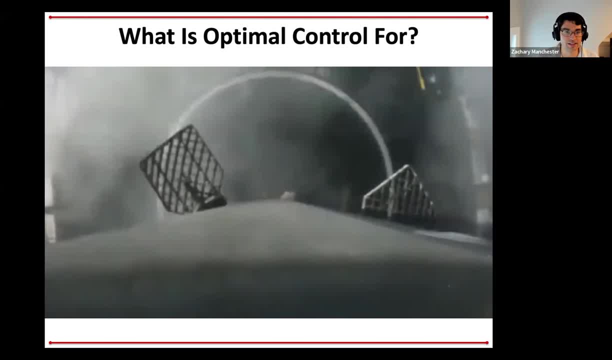 So this is how we land on Mars and things like that, which is pretty cool. Someone said graduate student descent. It is thankfully not quite that bad, All right, So that's that OK. So another kind of current hot area: autonomous driving. 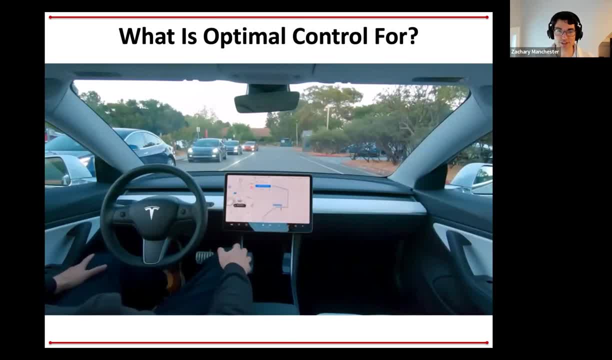 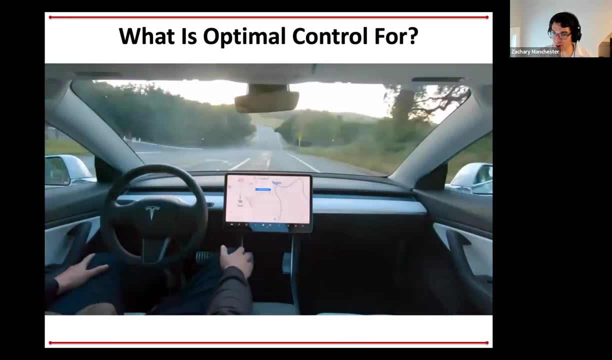 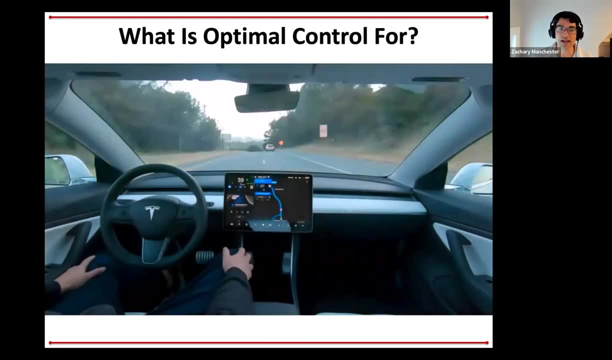 Tesla here being kind of one of the big players in this and one of the interesting examples. OK, All right, All right. So arguably the control problem here is not really the hard part. A lot of the kind of really tough challenges here are on the perception side of this problem. 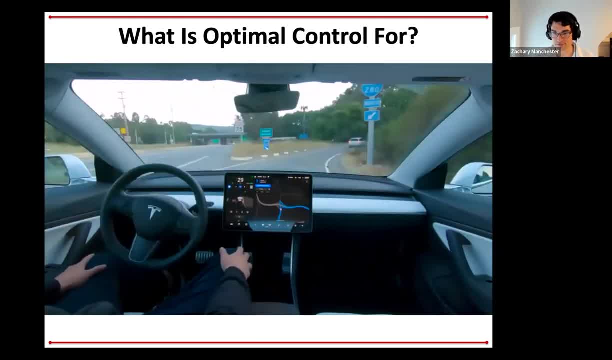 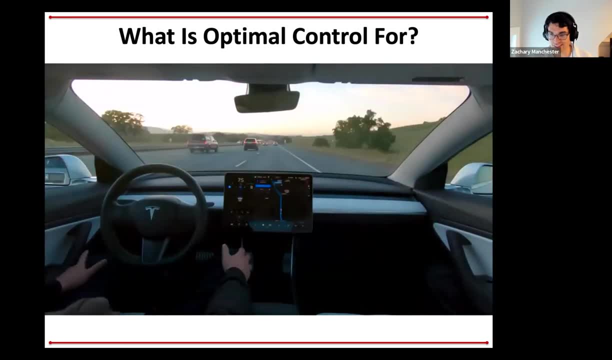 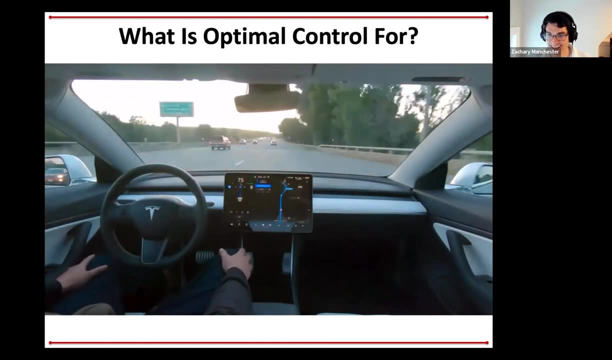 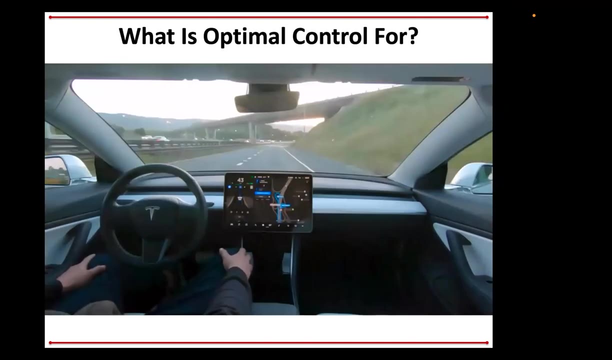 But anyone have any thoughts on how this gets done? Has anyone looked into this or did anyone work on driving stuff, on this kind of end of things, Thoughts, comments. somebody say something. Help me out. Cass Speculate- Could it be an adaptive controller? 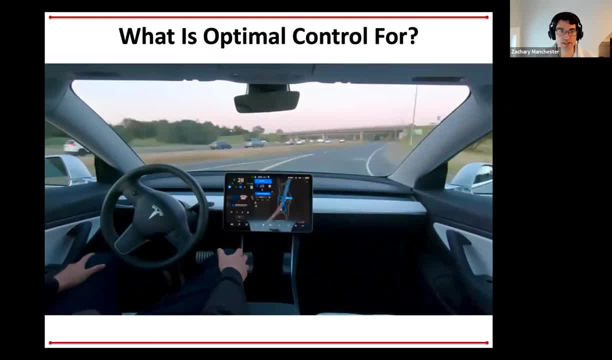 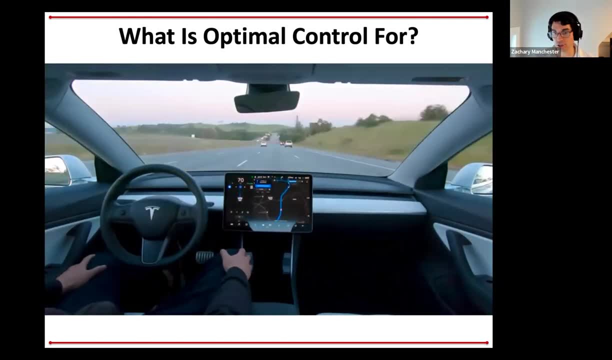 So this stuff- not so much actually, So like kind of what the standard approach here is, as again MPC for a lot of it And then often some lower level linear tracking control stuff. So here the kind of the standard approach is to use a simplified dynamics model for the car. 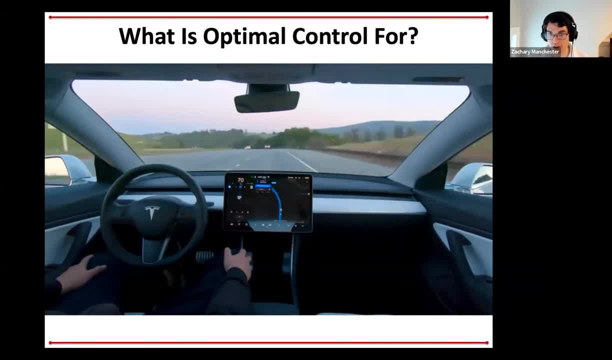 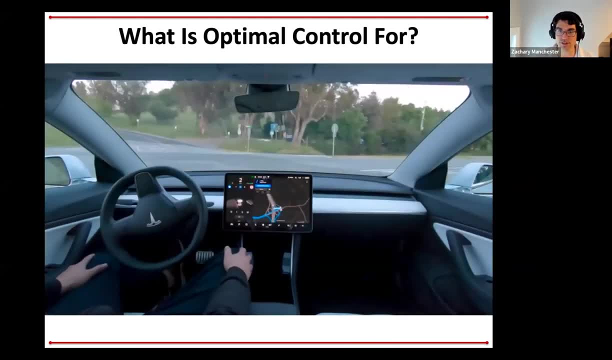 A lot of times people use what are called single track or bicycle models, And then it's kind of the standard approach. It's kind of nonlinear MPC with constraints for collisions and obstacle avoidance, and that kind of stuff is kind of the standard way of doing this. 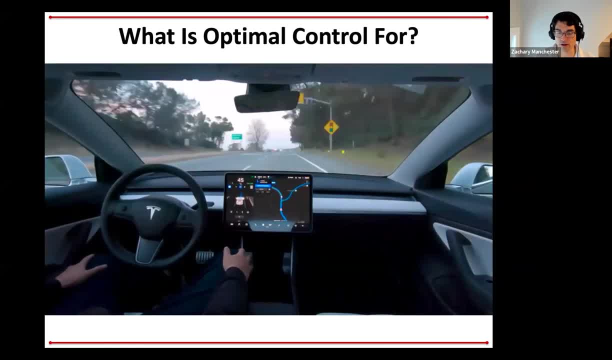 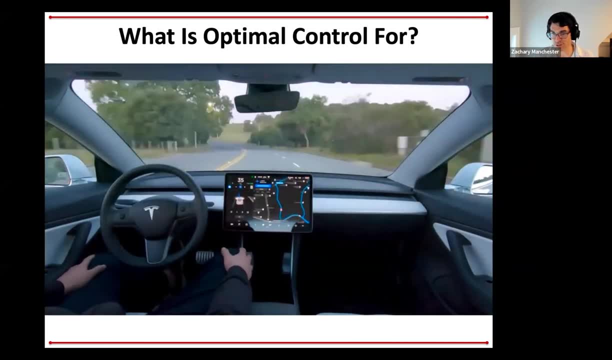 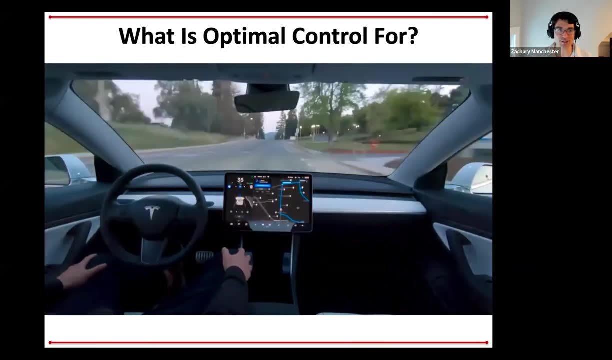 But there is some really exciting frontier research, some of which we've done in our lab, on what's called kind of game theoretic control, which is where you try to reason about the behavior of the other drivers and how your control moves might interact with them and what they might do in response to you for things like merging and passing and stuff like this, which is pretty cool. 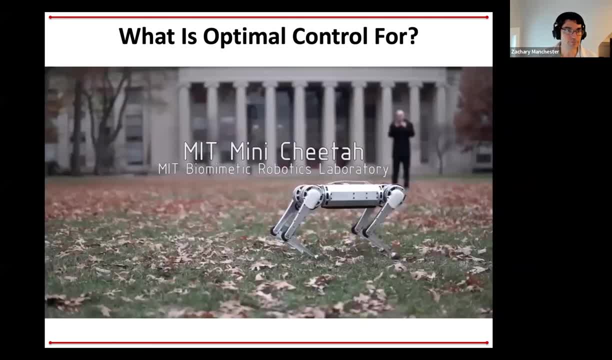 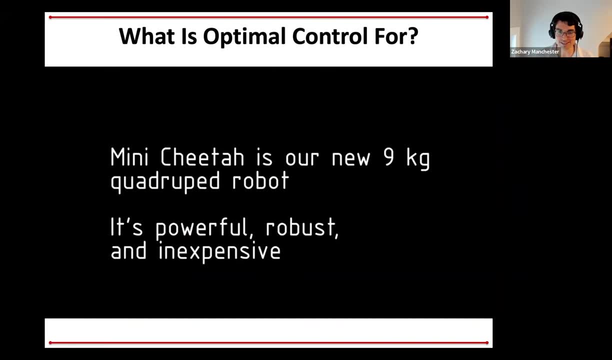 So that's kind of interesting stuff in the driving realm. Okay, so some more stuff That's sort of state of the art and cool. MIT CEATA- A lot of people know about this and have seen this, And this is one of the more exciting and more dynamic winged robots. 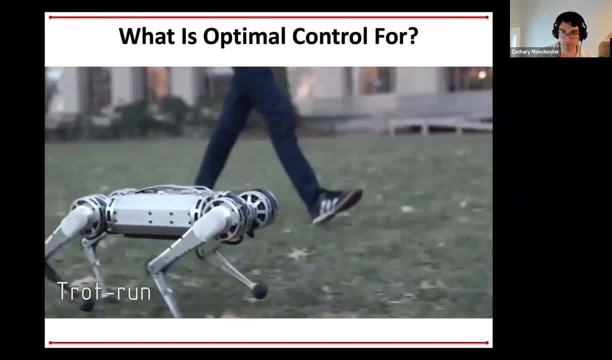 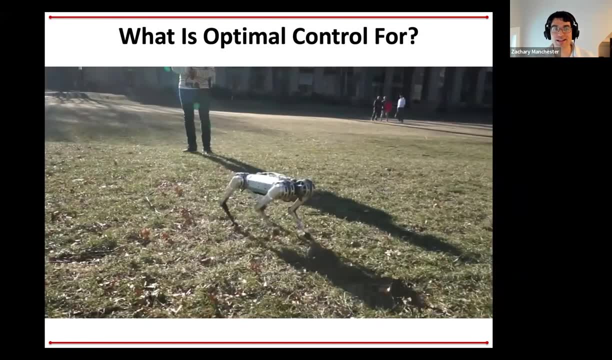 So this is once again model predictive control. A lot of tricks in here to make this into a linear model predictive control problem so that it can be solved online quickly, But some of the more state of the art stuff is actually now venturing into nonlinear Motherboard. 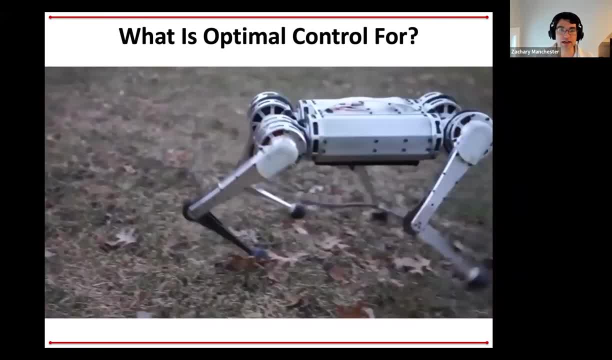 So that's kind of what we're trying to do. So some of the more state of the art stuff is actually now venturing into nonlinear MPC- Okay, linear MPC here. So this is sort of: there's a linear MPC layer at the top. 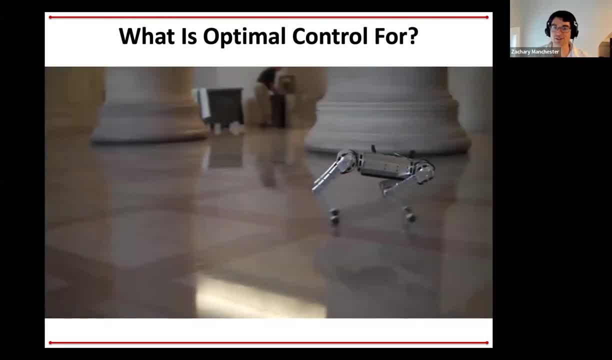 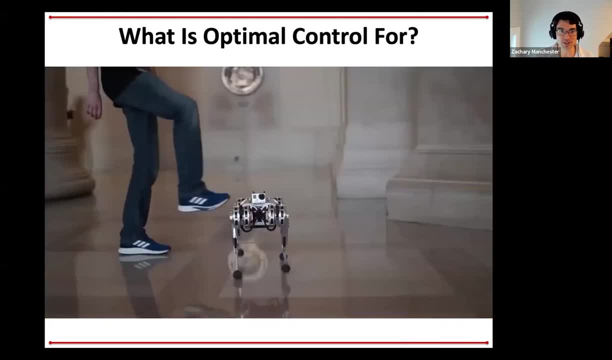 and then there's a bunch of kind of clever low-level control stuff going on so that you can treat this thing at the high level as a linear system, which it is most definitely not right. It's a super non-linear. So there's a bunch of secret sauce in there. 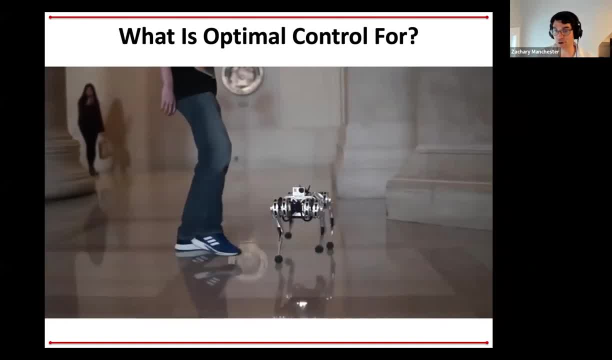 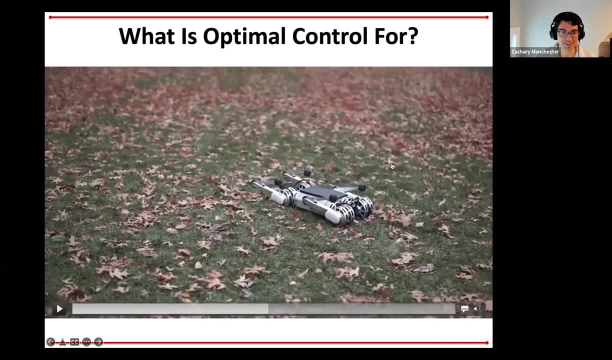 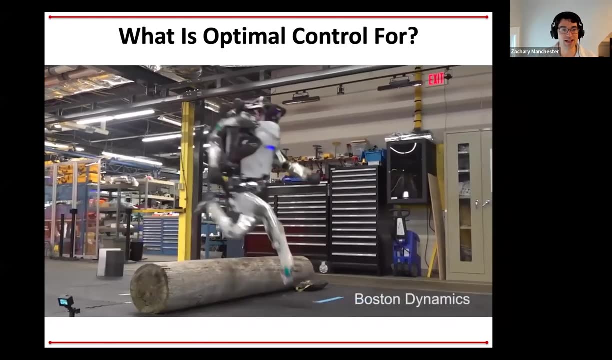 but at the highest level it is again a linear model predictive control problem or convex model predictive control problem that gets solved And sort of maybe most exciting and kind of state-of-the-art of all the stuff is- everyone's seen this stuff, Boston Dynamics. 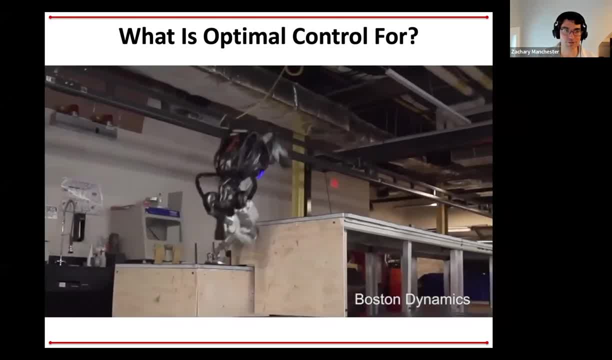 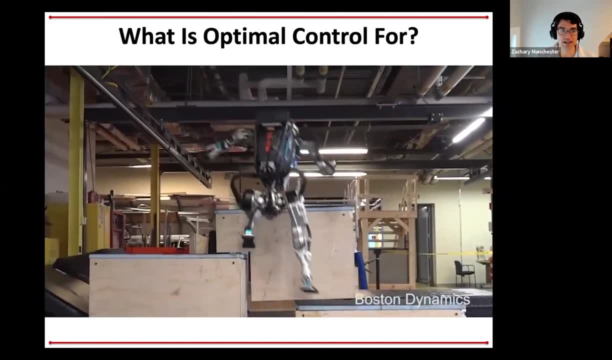 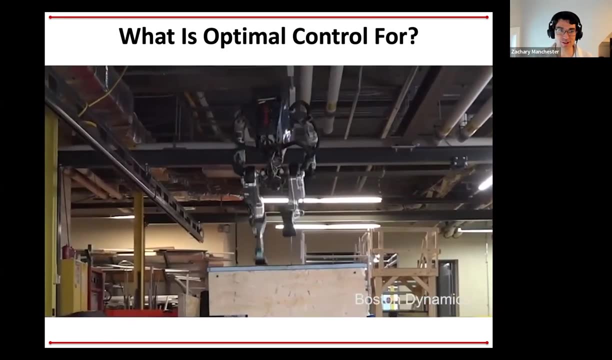 This is pretty much at the cutting edge of our field, And this stuff is just an incredible look at what they can get these robots to do. Anyone have any thoughts on what these guys are doing? This is actually pretty speculative on my part as well. 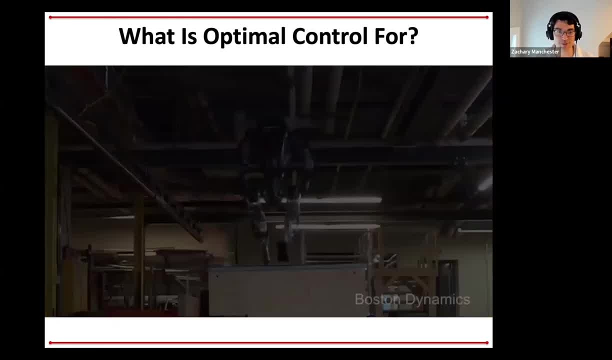 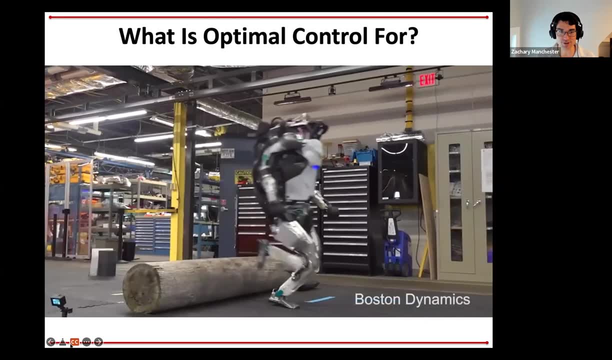 Like I had friends who worked there and like know a little bit about what they're doing And I have some good ideas but these guys don't publish and don't talk about it, So we're all guessing. Does anyone have any thoughts on what these guys are doing? 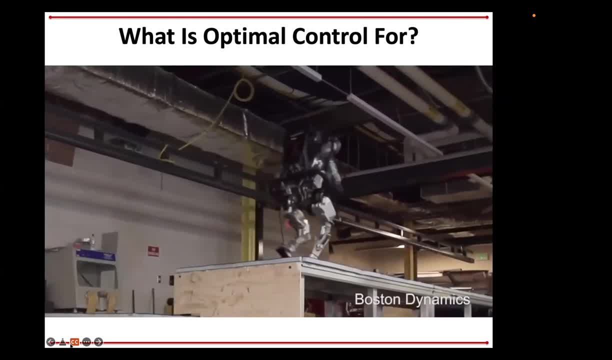 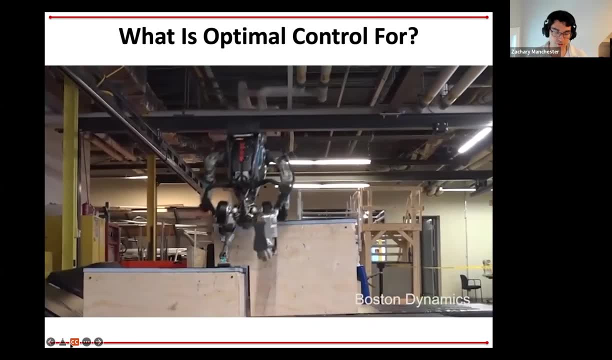 Do they do an offline trajectory optimization and then an online MPC? Yeah, so yeah, that's. you know. as far as we know, that's, and like, as far as I'll talk about, that's pretty much what's going on. 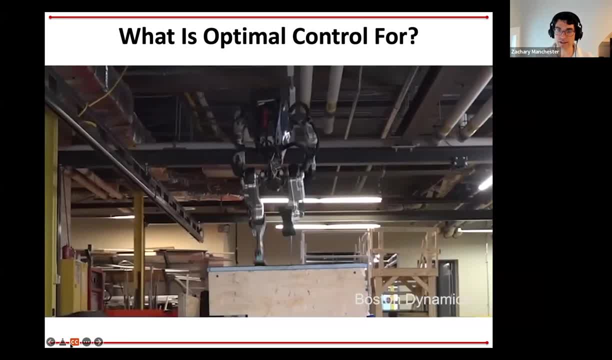 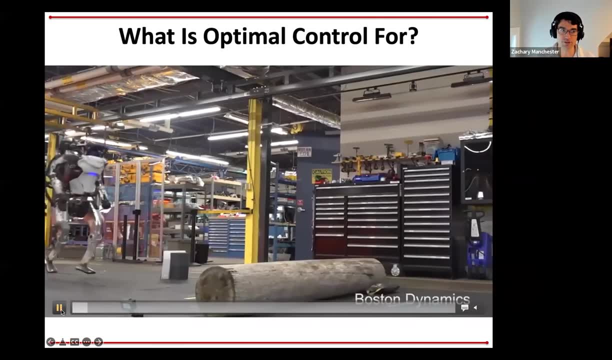 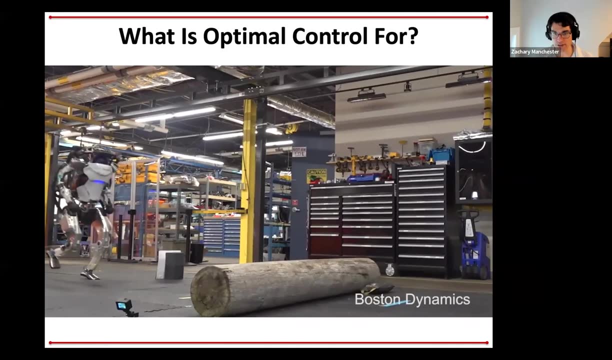 So, roughly speaking, what they're doing is an offline- you know, very slow, non-linear trajectory optimization, Step to plan these motions. So they're like with the full nonlinear dynamics of the robot, all the details in there, all the motor dynamics et cetera. 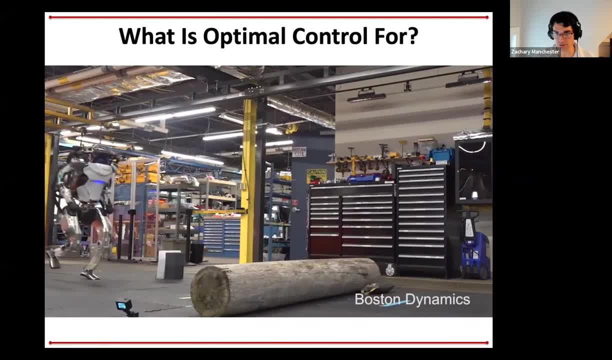 et cetera. So they're doing this like really kind of intense, high dimensional, big nonlinear optimization problem, offline to figure out how to move the robot, and then online they're doing some sort of convex model predictive control again, probably solving QPs again. 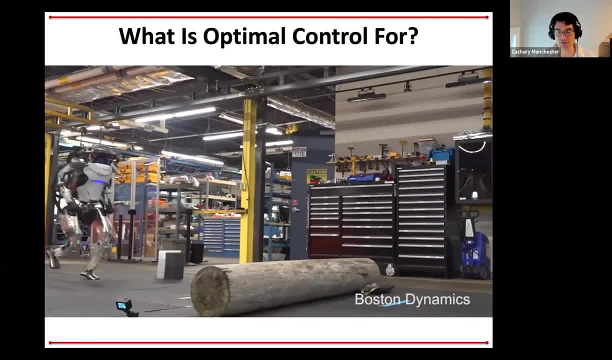 using a bunch of simplifications and linearizations to track these, these pre-computed trajectories, along with some really clever stuff where they can sort of build a library of trajectories that they've computed offline and then select from them or switch between them online, sort of like template style, and 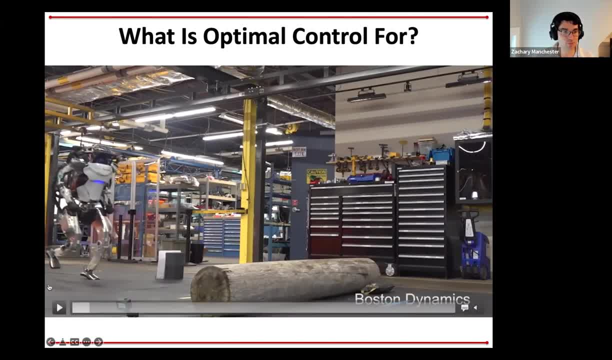 then track them in kind of interesting ways. So that's sort of what we think they're doing. So, yeah, as far as. so I see people writing this chat. It's it's. thanks for doing that. That's cool. Unfortunately, I can't see the chat with the PowerPoint on when we switch over. 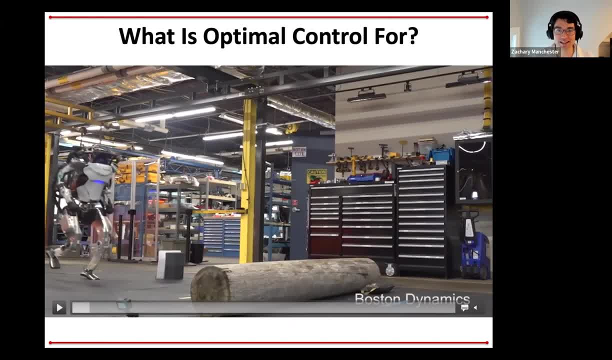 It might be easier when I stopped doing PowerPoint, But for now you have to speak up. This is a much closer to graduate student design. to whoever said that, that's kind of true, Okay, cool. So Boston, these are kind of some, you know, totally state of the art. 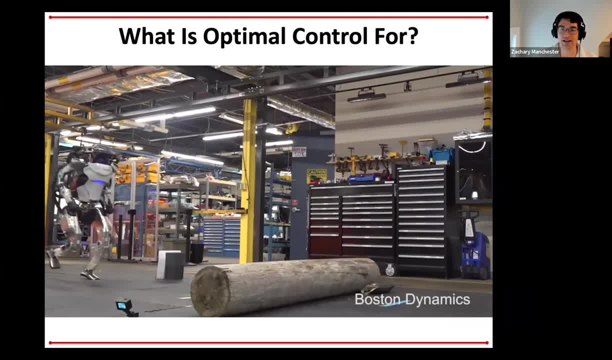 This is- and, by the way, we're going to explicitly go through most of these at the end of the class as kind of case study examples. So we'll get you pretty close, like right up to the frontier, hopefully, with some of this stuff and hopefully you can leverage it. 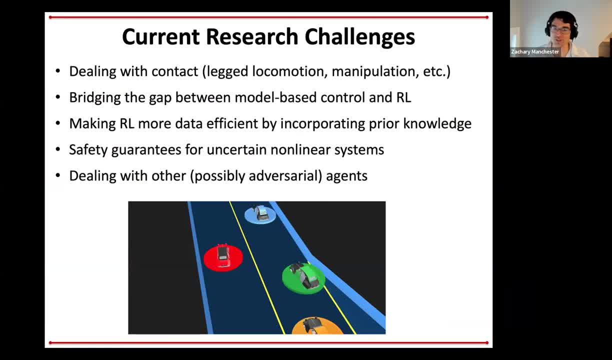 So some kind of like more forward looking current research challenges, like what are we working on In our lab And what are others working on in this field, And where are kind of the really hard problems that we still don't know how to solve? 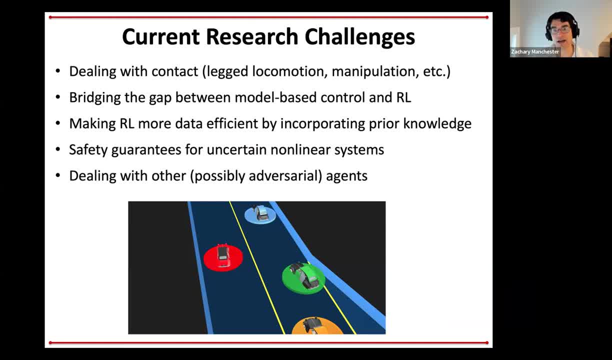 Here's a handful. So one is dealing with contact in general. So like a locomotion would be a good example of this. You saw a cheetah, You saw Atlas, and also in manipulation tasks, right Where where you're grasping, and things like this. 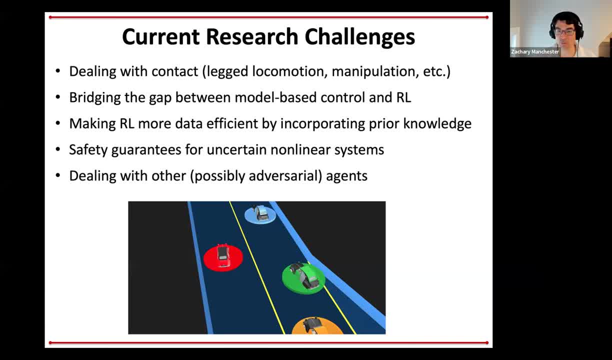 So anywhere where you make and break contact, things get really nasty and really complicated And right now pretty much every controller that deals with scenarios like that has some hacky heuristics in it to deal with what exactly goes around on around where you make and break contact. 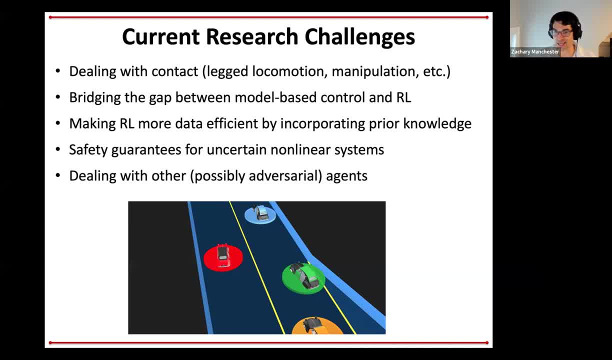 And there isn't really a good general, theoretically well grounded set of tools for dealing with contact rigorously and control theory right now. So that's a big one that we do a lot of work on in the lab. Another one is- and we'll talk more about this, but really kind of bridging the gap between model based control. 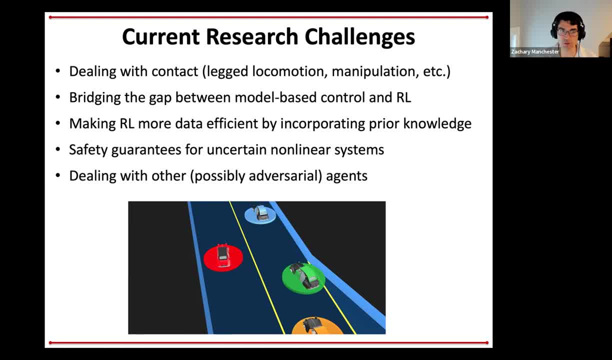 Kind of more classical stuff and reinforcement learning ideas, and then you know, kind of very related to that, making RL more data efficient by incorporating prior knowledge, AKA incorporating more model based control. So bridging the gaps between these things is kind of really interesting right now. 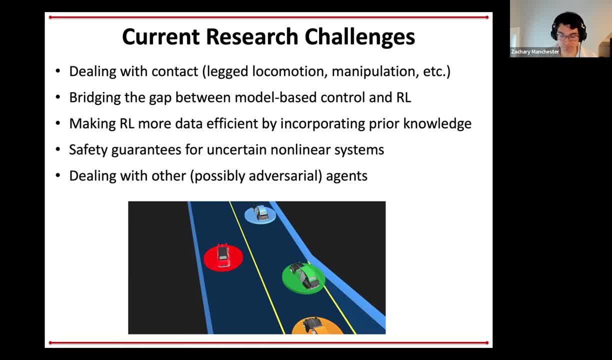 There's a lot of work going on. That's a very hot area in general. From my perspective, RL and optimal control are really the same thing. They're kind of just historically existed in different communities or different from different viewpoints or different departments. 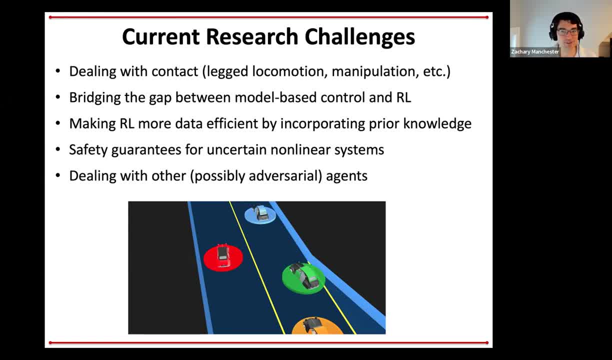 But they're really the same thing And so now they're sort of starting to come together a little bit, which is kind of cool. So a couple more one another one is safety guarantees for uncertain and or nonlinear systems. So how can you actually guarantee that your thing's not going to faceplant or blow up or crash, given we have imperfect models of the world and bad things can happen? 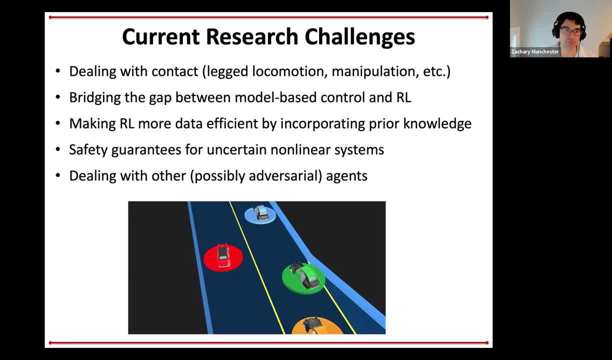 Can we give any guarantees and what sort of guarantees can we give on performance and robustness and things like that? Yeah, I think that's a great question. And then, lastly, sort of related to this driving stuff and the game theory stuff, how do we deal with other, possibly adversarial agents? 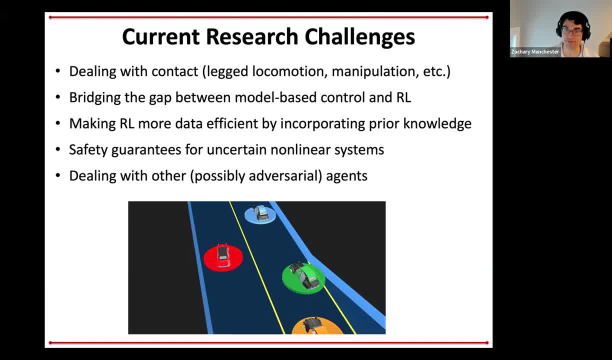 So this shows up most prominently right now in autonomous driving as a huge deal. So these are a handful of like four looking things. We're happy to talk about all this stuff. You know we work on a bunch of this stuff in the lab. 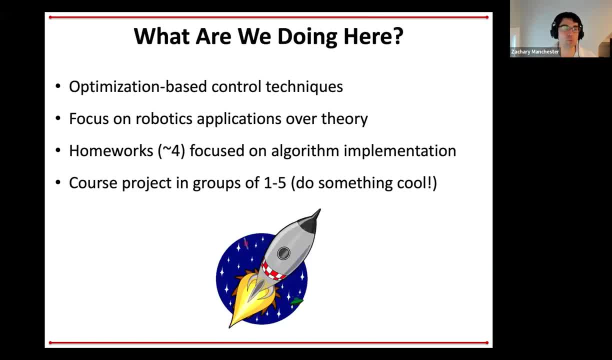 OK, so that's kind of that story. So what are we doing here in this class specifically? So number one, we're going to be focused on Optimization based control techniques, so that the title optimal control- I mean that- has a lot of sort of baggage or implications maybe attached to it. 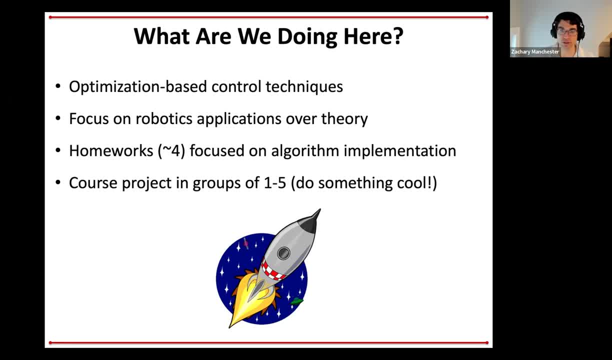 And what we mean by that is we're going to use optimization to do control And that's sort of a very broad set of tools and ideas. we're going to focus on very heavily on applications- robotics, applications in particular- over theory. So this isn't really going to be a course where we are like proving theorems or deriving the. 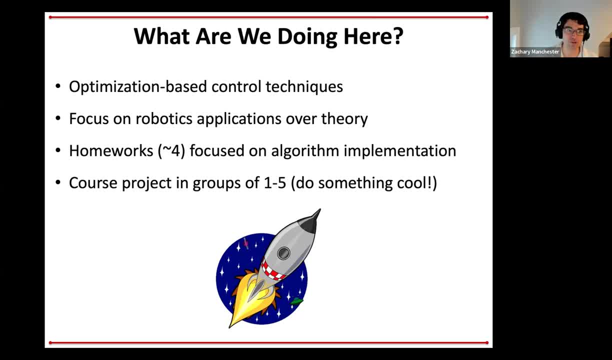 You know, patriarchal minimum principle or things like that. We're mostly going to be focusing on coding up algorithms and really doing it with an eye towards, hopefully, you guys being able to take this stuff and go apply it in your own research or in your own careers after this. 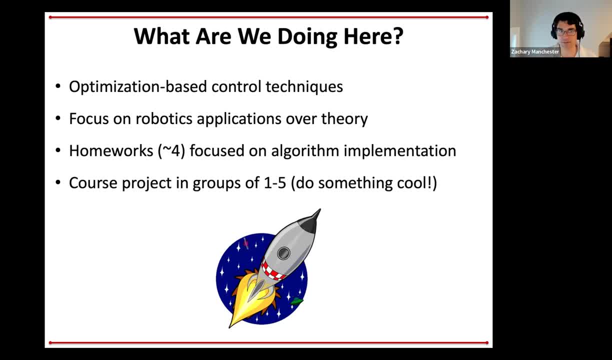 We're going to have four kind of major homeworks over the course of the semester. They'll be again. they'll be coding assignments focused on implementing algorithms, trying stuff out, that kind of thing. So there'll be sort of Jupyter notebook based things and do on GitHub and this kind of stuff. 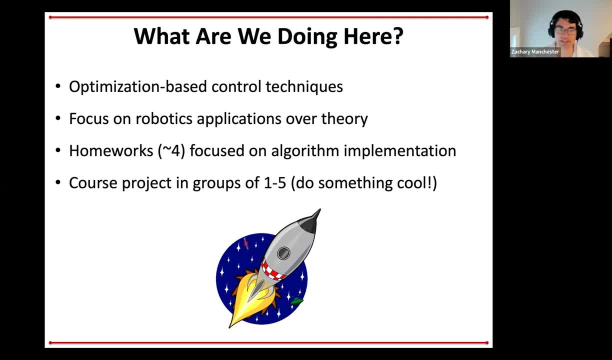 And then, lastly, we're going to have a course project that you guys are going to work on in groups, normally groups of one to five, I think I would. I think it's a better idea if you do this with somebody else. so if you're, if you're inclined to do by yourself, I mean that's okay. if you really want to do, if you have something from your research that you want to do here, that's, that's cool. 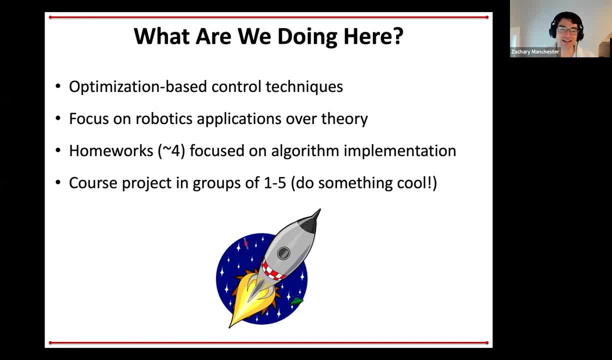 But I think you'll have a better time doing that. I think you'll have a better time doing it with a friend or two, and the idea here is to do something cool, do something interesting that interests you. hopefully, if you're- if you're a graduate student, you can do something that's sort of directly related to your research and hopefully get a kickstart, sort of jumpstart, on a conference paper or something like that, and do something that's just totally relevant there. 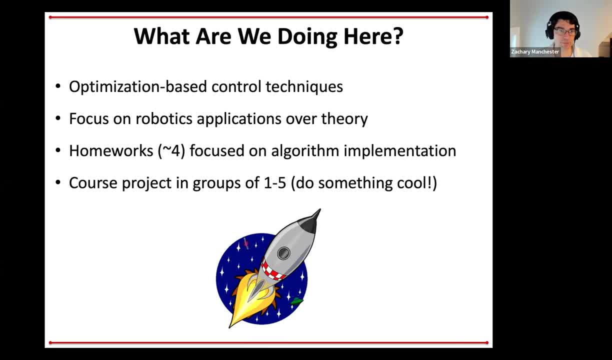 We don't want you to like spin your wheels on something you know random here. do something that matters to you, do something cool, Okay. and I should say, as I said, disclaimer out the gate. this is definitely more of an optimal control class. it's definitely from an optimal control viewpoint as opposed to a reinforcement learning viewpoint. 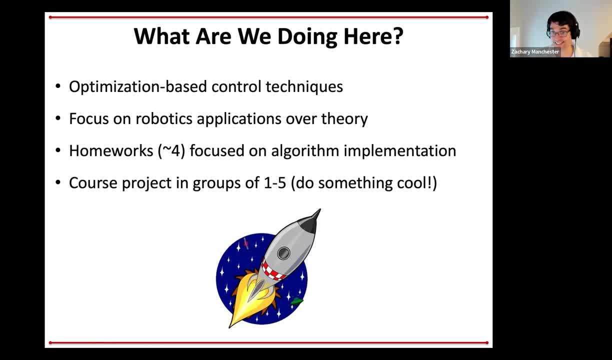 As I kind of alluded to before, from my perspective these are really the same thing and it's really just a matter of perspective and viewpoint. and, like a lot of times, did you use a polynomial or a neural net in your function? approximation is really what separates these things, so we're going to kind of try to look at this from a uniform viewpoint. mostly deal with 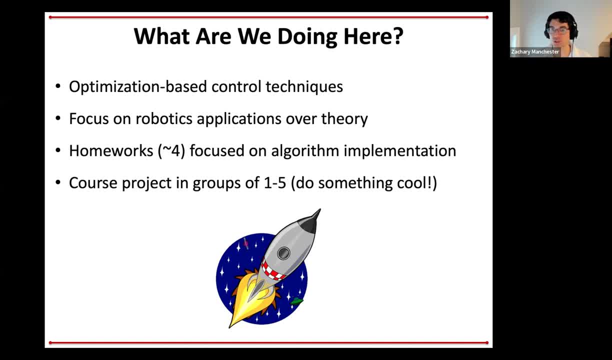 model based stuff. but we'll also talk a bunch about what you do when you don't have good models, how you can use data driven techniques and sort of, where all the connections are between optimal control and RL and they're really kind of, you know, it's a continuum and they're really kind of the same space generally. so hopefully we'll set you up with kind of a good baseline set of tools here and techniques and sort of knowledge base that you can use and apply in any of these settings. 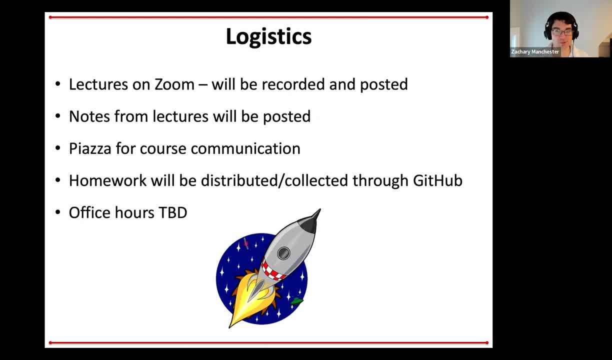 Okay, so logistical stuff. Lectures are on Zoom, as you all know, for now, because you're here, we hopefully will be back in person in a couple weeks, TBD. so more on that I guess in the next couple weeks, and I will record and post the lectures. this is getting recorded right now. 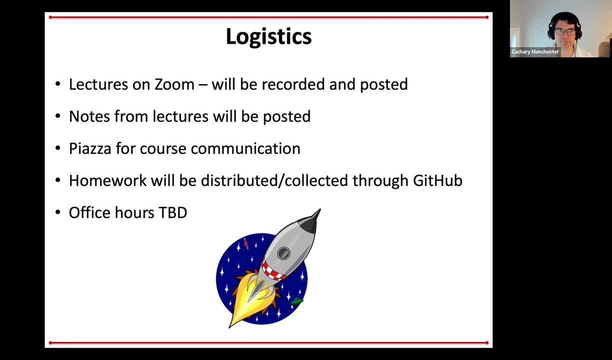 I'll post them on YouTube in a playlist, and even when we go in person, I'll still record and post lectures. So let's see, I'll also post my notes. I'm going to write on a tablet and those I'll PDF them and upload them to GitHub. I'll also do a lot of Jupyter notebooks. 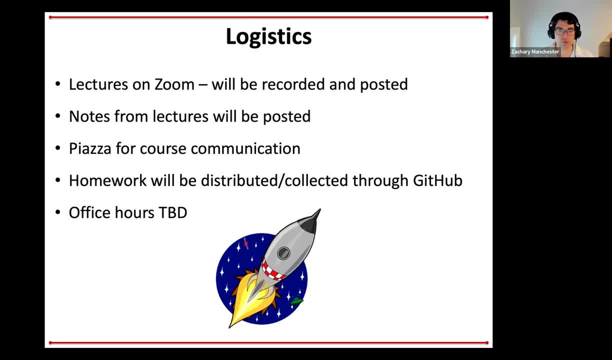 and kind of demos in class where we play around with the code live. hopefully it works most of the time and so I'll post those Jupyter notebooks along with my handwritten notes. We're going to use Piazza for like kind of course communication, real time Q&A etc. Hopefully all the course communication we can kind of just do with Piazza. 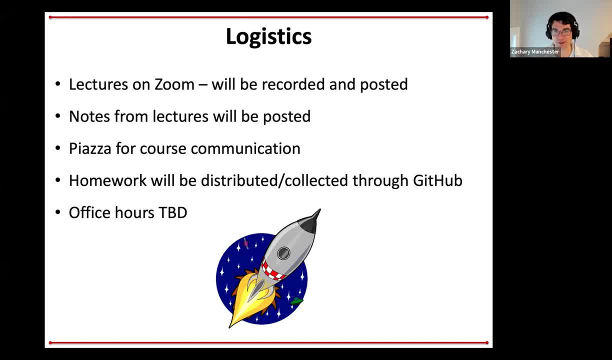 and avoid email, And I really don't want to use Canvas. I'm probably going to use it just for posting grades, but we're not going to like collect assignments on there or do any sort of communication really through Canvas at all. So definitely get on the Piazza site. We're going to use that for pretty much everything. We're going to use GitHub to collect assignments. I think that's about it. 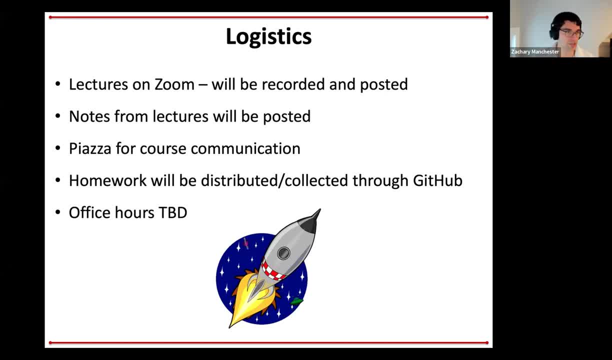 Yeah, so GitHub. we're going to use GitHub extensively, so I need a GitHub account. I'm going to send out some kind of poll for office hours. So those are TBD. They'll be on Zoom for now and we'll see in a couple weeks, but we'll kind of dynamically adjust as we go for this stuff And don't hesitate to reach out if you, you know, need to talk anytime. We're pretty flexible and there's a bunch of us, Okay. so 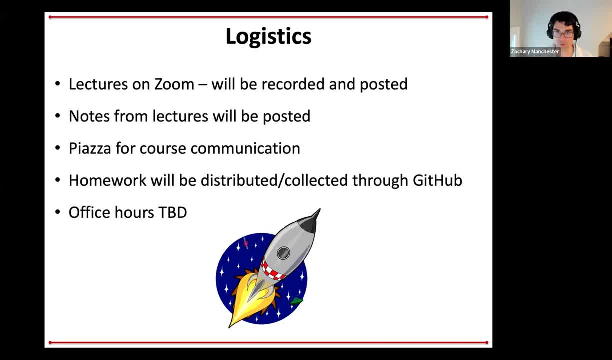 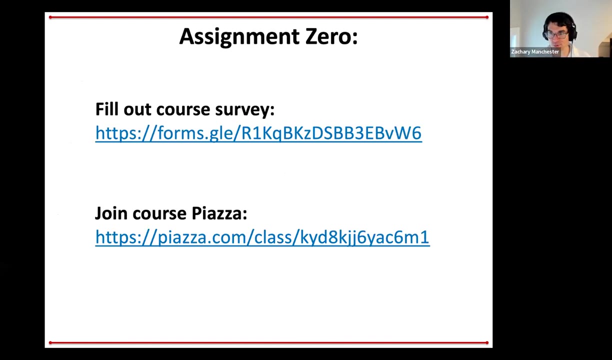 any questions about any of this stuff, any of this logistic stuff, And just unmute and speak up if you've got any questions. Anything I've talked about so far- Questions- concerns comments, thoughts. Okay, so onward then. So we have two kind of like two things for you guys: assignment zero, we'll call it So. first is there's a course, survey, Google form- that's just me asking questions about like. 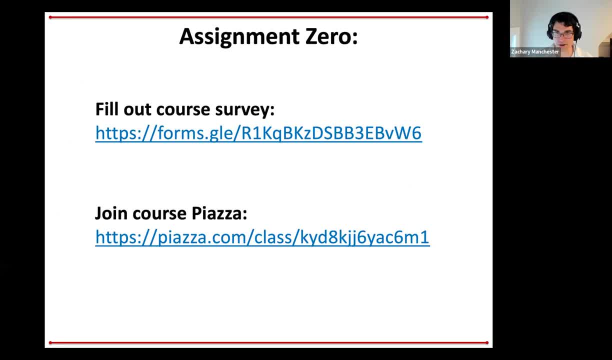 courses you've taken before, kind of background things to try to gauge where everyone's at and hopefully target the content a little bit, and stuff like that. And then we're the Piazza site. we're going to use GitHub for that, which we need everybody to join. So there's the links. This will all get posted. 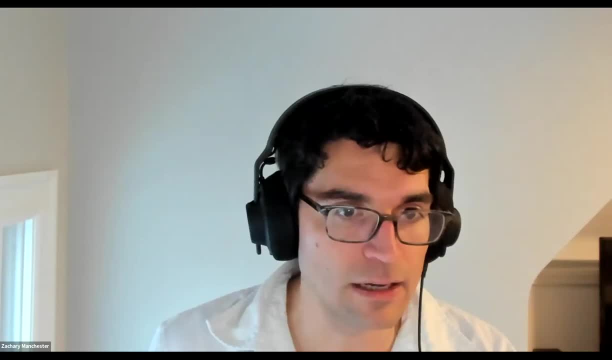 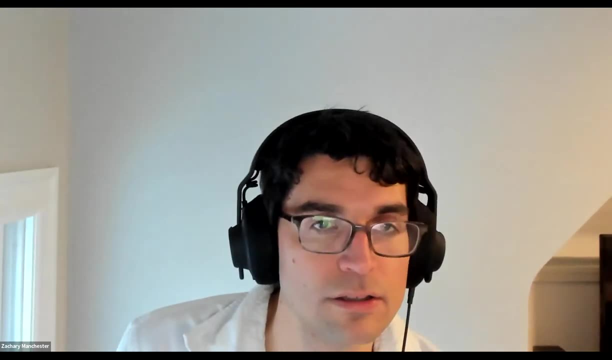 I can probably put these in the chat as well. I'm going to stop sharing my screen for a sec And then I'm actually just going to pull up the Piazza site and we can look at some stuff there. Okay, so let's try this. 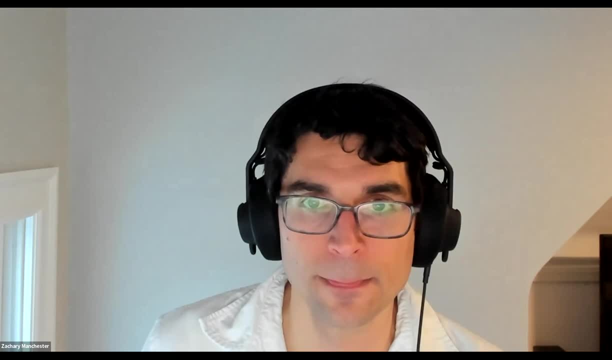 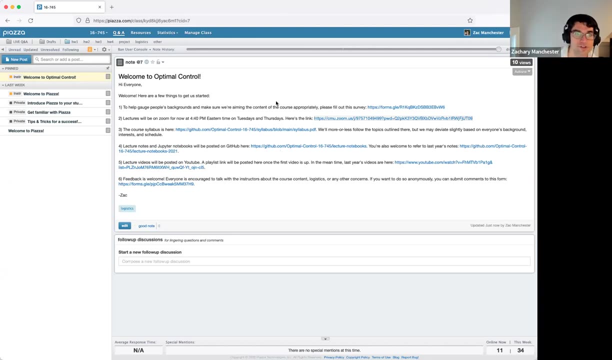 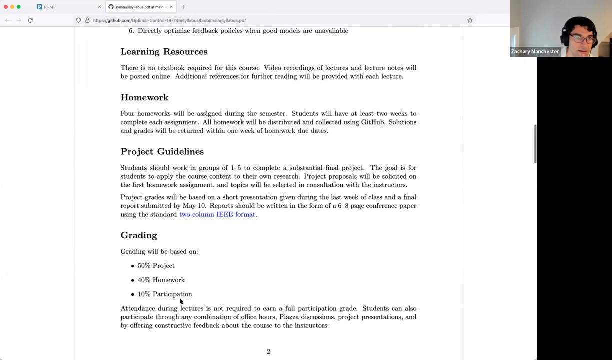 So a couple more things. Okay. so here's the Piazza site And then right on the front page, here's kind of the survey link, the Zoom link, the syllabus, which we can take a quick look at, Just kind of go through see if anyone has any questions on this. So really, what we're going to look at here. so grading it's going to basically be half projects and then sort of 40% homework, meaning each homework is worth 10%. 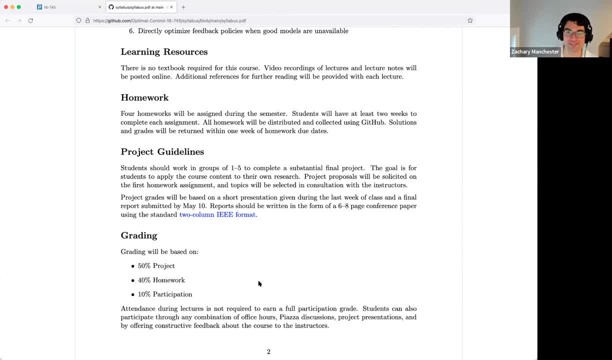 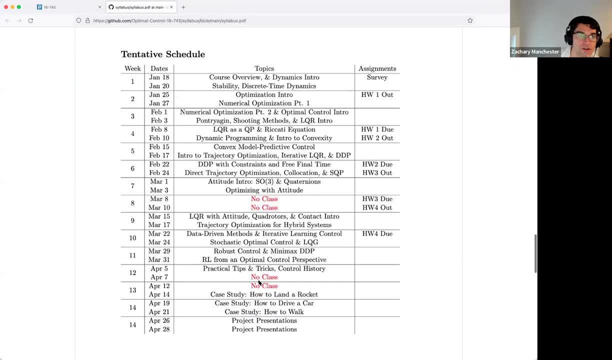 And then 10% participation, which is really like giving me wiggle room to bump people in the event that things are on the edge, stuff like that. Okay, so here's kind of what we're going to talk about. So today we're going to get. after we're done with all this upfront stuff, we're going to get into dynamics, And this is just kind of 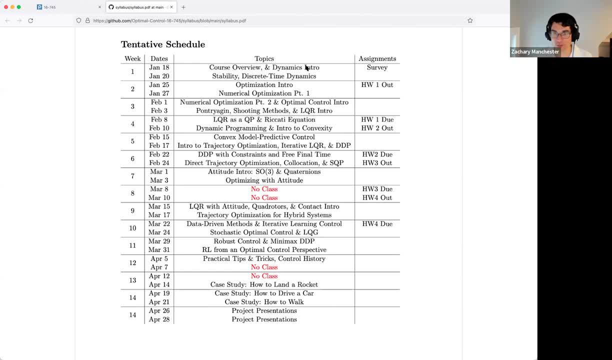 background on dynamic systems that you need to be able to do control and hopefully that's mostly review. Next time we'll talk a bit more about stability and discrete time dynamics, which is how we get these into a computer. Then we're going to have a few. 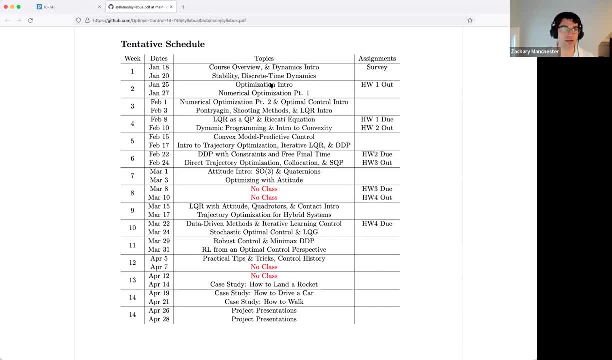 Then we're going to have a few lectures on just optimization in general, So kind of intro to optimization, and then a bunch of stuff about numerical optimization, how you actually solve these optimization problems with a computer, getting into how we deal with constraints, things like that, And then we'll get into sort of optimal control, which is kind of a special case of optimization in general. 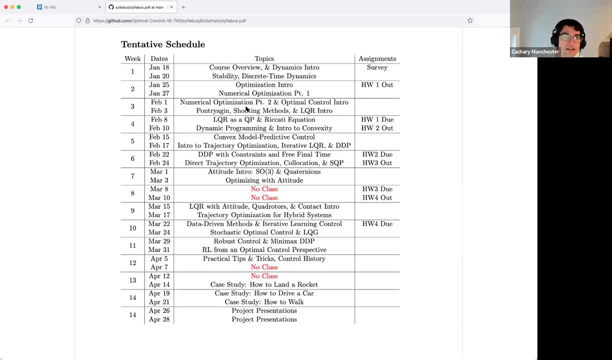 Some classic stuff, the Pontryagin minimum principle, shooting methods, LQR, sort of bread-and-butter stuff, kind of equations, dynamic programming. Then we're going to get into a sort of convex model, predictive control, a bunch of which is used all over the place right now. It's kind of 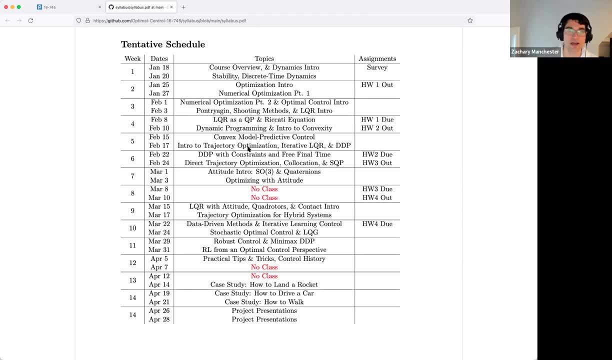 one of the standard things to do. Then we're going to get into sort of nonlinear trajectory optimization- how you solve those problems, a bunch more tweaks on top of that. setup, direct methods, so co-location methods, things like that. Then we're going to talk about how to apply these methods specifically. 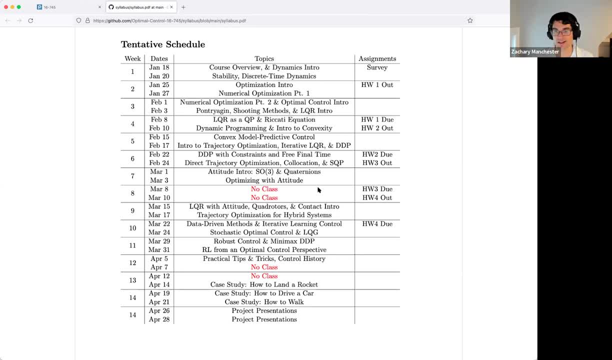 to systems that have 3D rotation, which shows up all over the place in robotics. Anytime you have a non-fixed-base system, so legged robots that can rotate around all the way or do flips- aerial vehicles, drones, spacecraft, underwater vehicles, right? So anything that's not bolted to the world like anything other than a classic manipulator arm. 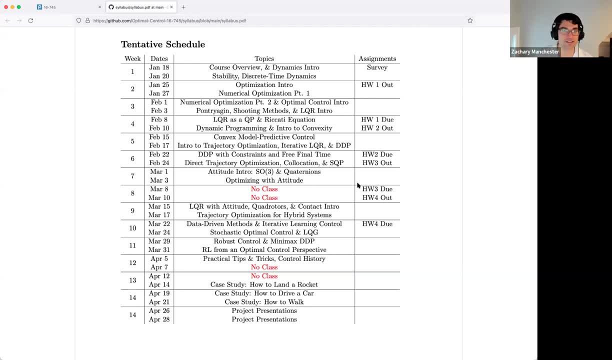 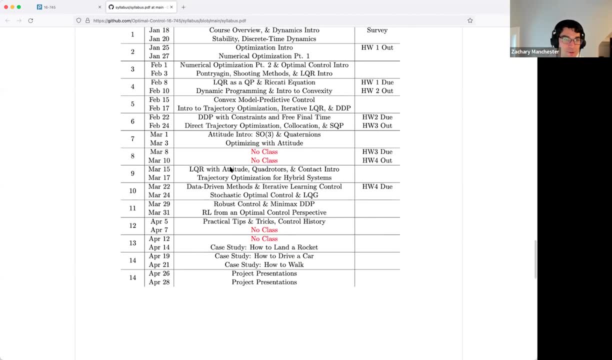 So we're going to talk a bunch about that stuff because it shows up in practice a ton And it's sort of a pet peeve of mine. People kind of do it the wrong way a lot, So we'll teach you how to do it the right way. So we'll do a bunch of that stuff. Then we're going to get into some more robotic-specific things. So we'll talk about contact systems that make and break contact a la you know, legged robots and manipulators. 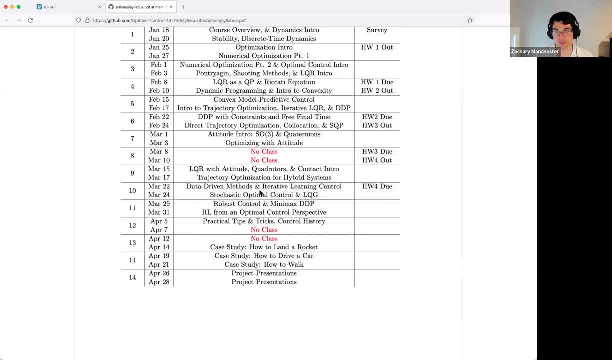 How you do trajectory optimization for those systems. so how you do kind of the cheetah Boston Dynamics stuff. Then we'll talk a bit about data-driven methods and what to do when you don't have super good models. Then we'll talk about stochastic optimal control. so noisy sensors, things like this, And the LQG problem, which is a special case, which is kind of one of the classic bread and butter results in all of optimal control. 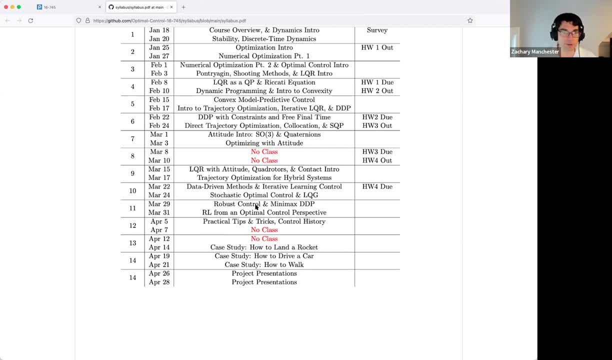 So this is basically LQR plus a Kalman filter. Then we'll talk a little bit about robust control. so what if you have uncertainties on your model and some methods for solving those problems? Then we'll do a little bit of a quick whirlwind tour of RL, hopefully. 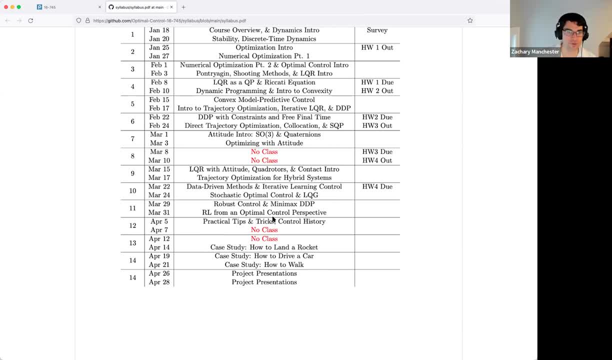 Kind of with the same perspective and notation and stuff from the rest of the course. We'll do some- I mean this stuff's RL as well- but this is sort of kind of maybe a broader survey of stuff. We did this last year and I think it was a good thing to have so kind of a practical tips and tricks session that shares a bunch of random things that. 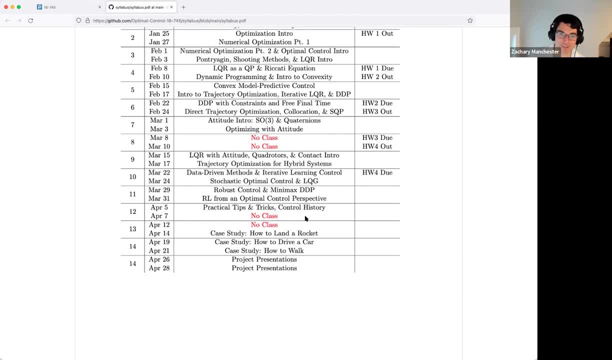 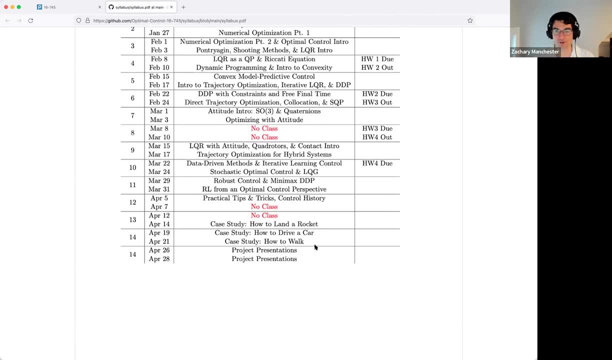 you should know about, but that aren't necessarily theory things that are taught in most courses. And then last year we did these case studies, which I think were pretty cool. I'm open to adding more of these or having different ones, but last year we did the rocket landing problem. 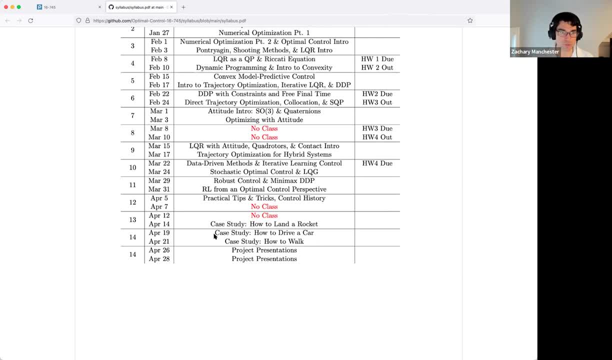 And then we did a bunch of stuff about driving and how the car stuff works, and then a bunch of stuff about walking systems and how kind of the quadruped humanoid stuff works. And then the last week is going to be for project presentation, so we'll kind of have you guys do lightning talks. 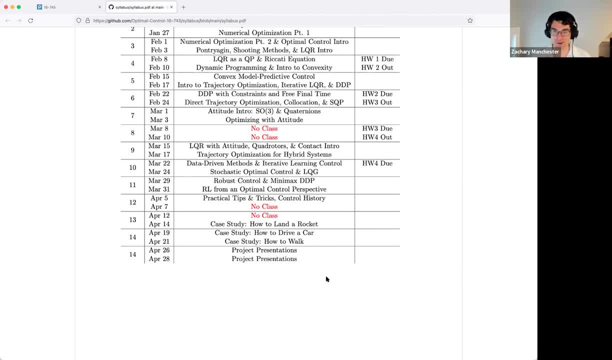 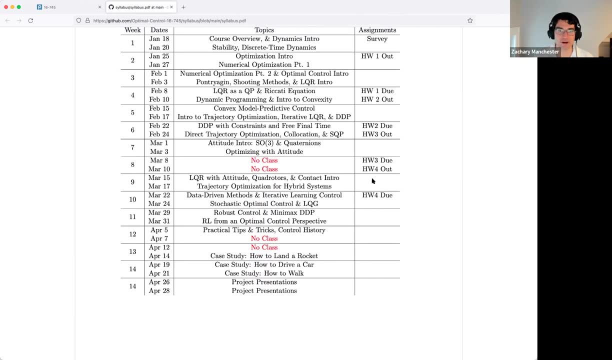 for the last couple lectures and hopefully that hopefully we can have some Q&A. You know it'll be fun, So that's kind of the idea. The homeworks here- these will probably get spread out a little bit more, but it's kind of just generic for right now. 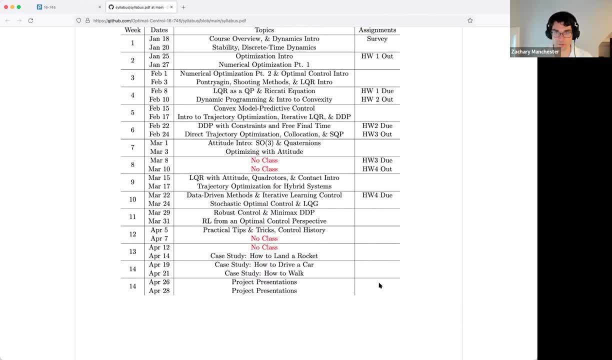 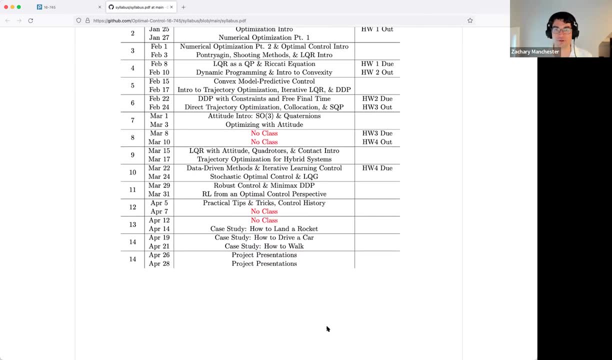 And then I'm leaving kind of a good few weeks at the end for you guys to really kind of dig into the projects. that's the intent at least, And the projects will be due, like as late as I can do it, kind of at the end of finals time or whatever, just a few days before the 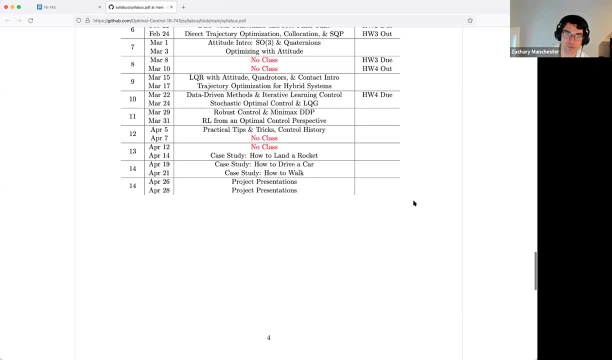 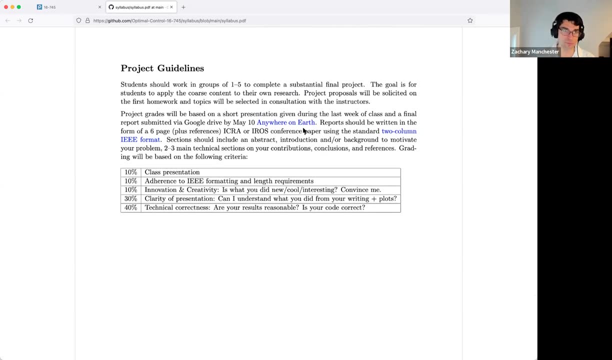 deadline for me to hand in the grades. so I'll give you guys as much time as possible there. So you'll have a bunch of time after the presentation slots to keep working on the project. And on that note you guys can all go read this. but just to give you a heads up for the project, you'll have to do this kind of lightning talk thing a couple minutes. 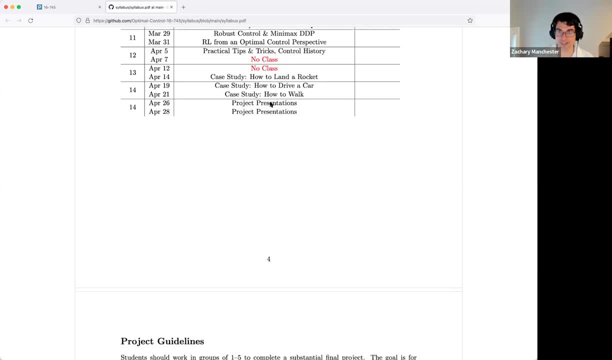 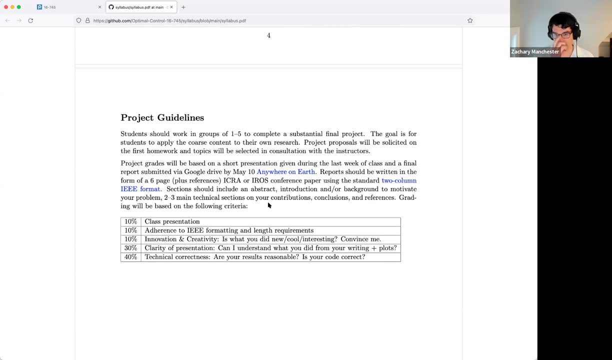 the last week. We won't expect you to have your full report done at that point. you'll have another couple weeks over the finals and everything to write it up. but the the idea there is to basically make it look like a conference paper, so we're going to have you do kind of a standard ICRA-IRAS. 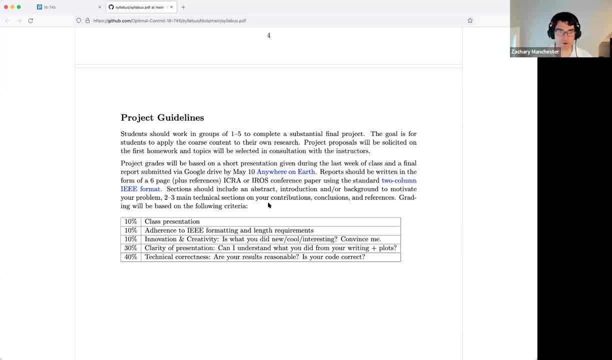 conference paper format. so it's a six-page, two-column lead format, kind of the standard thing, And so that's kind of the level we're looking for. here is roughly six pages and you know, kind of at the level of something you know that you could turn into a conference paper hopefully. 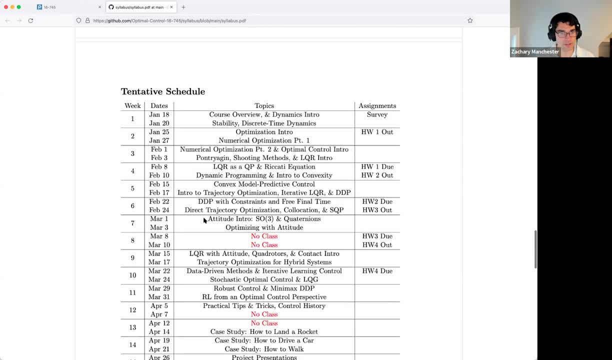 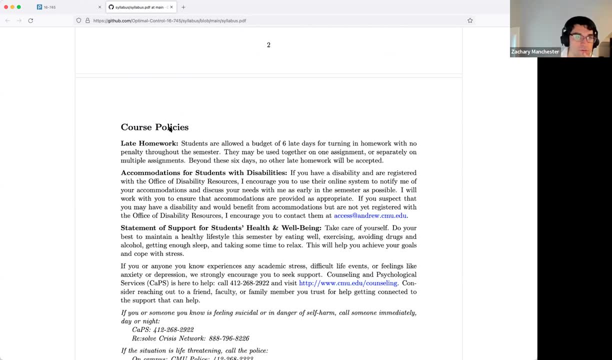 Okay, so that's, I think, kind of all the important highlights of what we're going to do in the class. Any questions about any of this stuff? Oh yeah, there's some other stuff to talk about. Okay, so late homework policy. so I'm going to just give you a budget of late days. 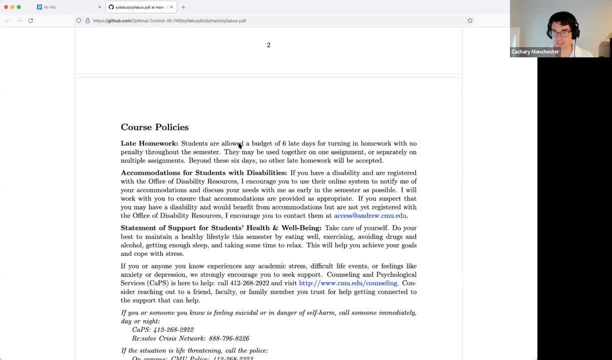 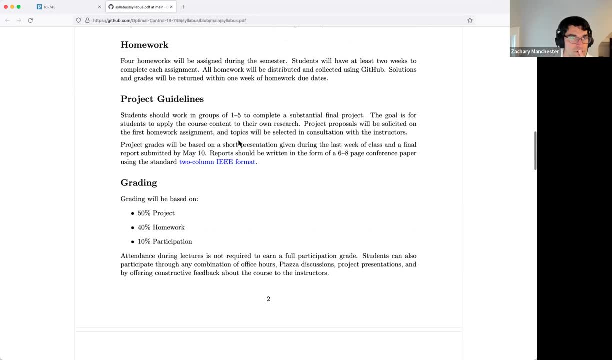 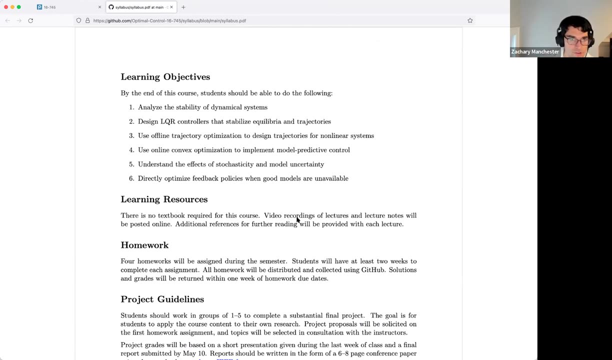 We did six last time and that worked out okay. so you just have six late days you can use on any of the homeworks in any combination you want. Is there any other important things? I think that should be it, So we already talked about this. No textbook, but I'm going to post videos, notes. all that stuff will be posted. 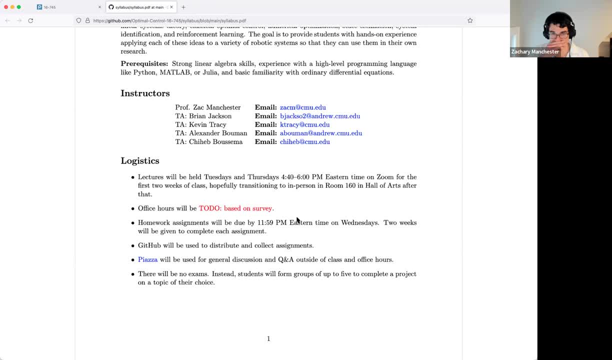 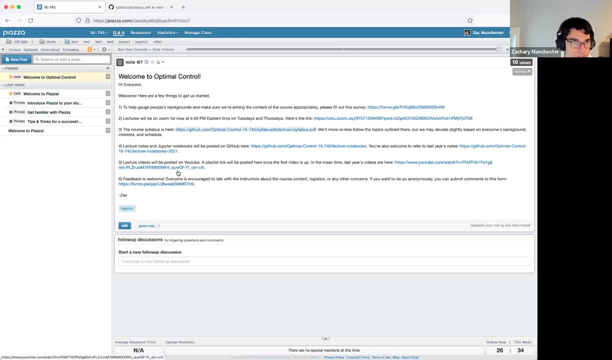 Yeah, anybody have anything before. we kind of- I think that's it for that for sure. Okay, so we'll do those. lecture notes will be on the next slide. Yeah, so that's going to be on the next slide. Okay, so we're going to do those. lecture notes will be on the next slide. 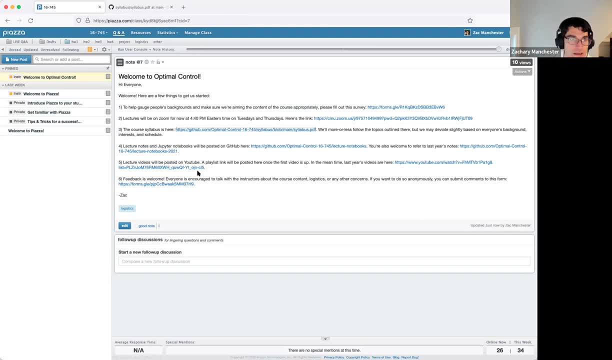 I'm going to put links, links. I think I'll put the link on GitHub. here's links last year's are up there too. If you want to look at last year's, I'm going to make a YouTube playlist with all the videos you can see last year's. 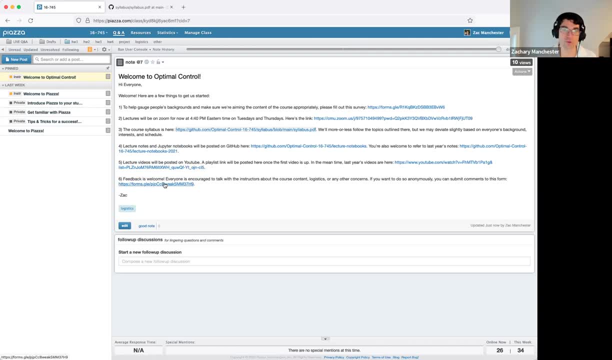 And then the last thing is we have this Google form. So, first off, yeah, We're not perfect. I make mistakes all the time. We can always make this better. So, especially with weird remote kind of logistics, It's kind of weird. So if anybody has any feedback, I always want to hear it. 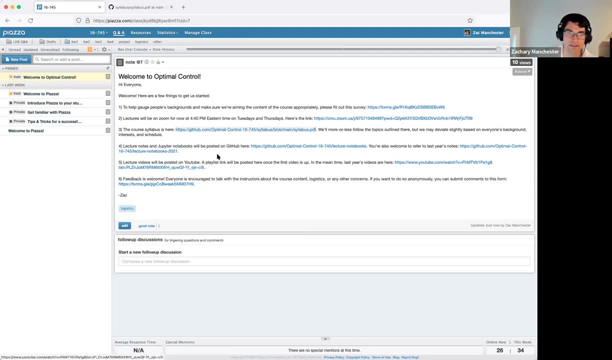 Talk to me. talk to the TAs anytime about anything. content logistics: Talk to me. talk to the TAs anytime about anything. content logistics concerns whatever you got. yeah, don't be afraid to speak up and then, if you don't want to, sort of 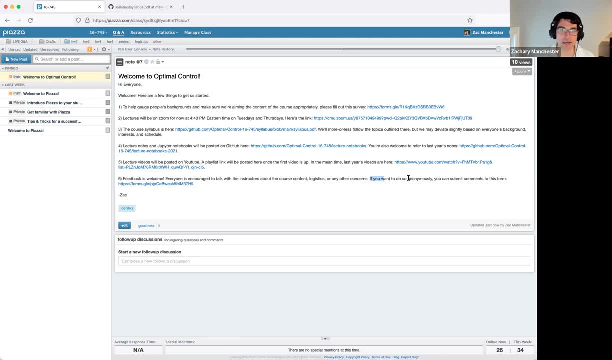 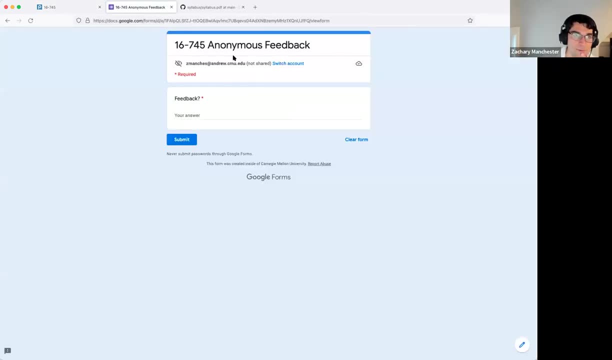 like talk face-to-face or Zoom or whatever. you can also do so anonymously. We have this Google form which does not record your email address, not shared. I promise it's anonymous and I just get a like totally anonymous email from this whenever you submit something with whatever you. 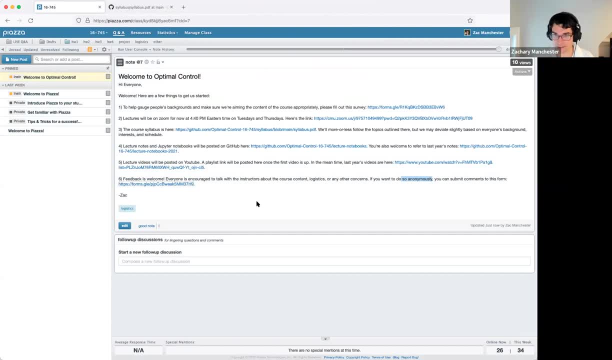 sent. so yeah, I think that's it. so anyone has any questions, feel free to speak up while I switch over to actual stuff. Yeah, I have a question. Yeah, Are the homeworks auto-graded on GitHub? So we have some, we have an auto-grader thing and we actually we try to be nice to you. 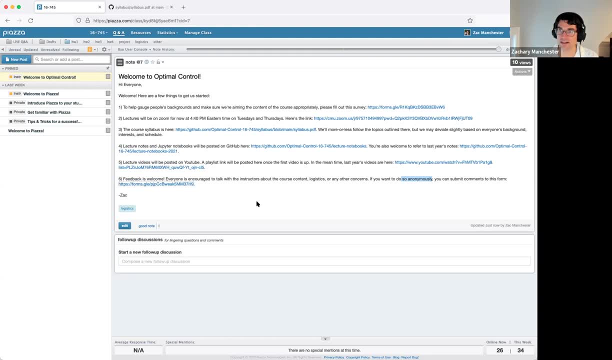 guys and we actually post sort of like along with the assignments. we'll post sort of unit tests that will evaluate your answers, so you can check your answers before you turn it in so that you'll know if you got it right. essentially so, there'll be like a set of tests that you can run yourself. 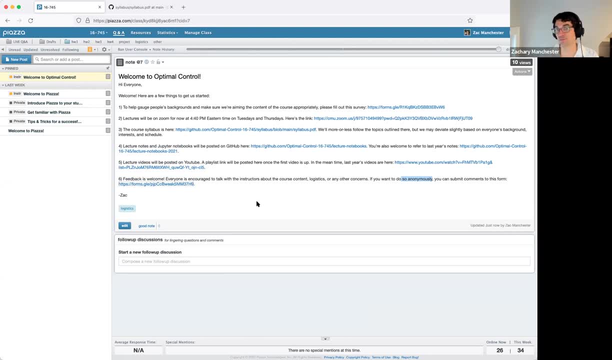 before you submit and then when you submit, we'll run a different set of tests on it just to verify. but yeah, so there will be like some auto-grading stuff. If you don't pass the test, we'll actually go look at it, you know, by hand and stuff like that and for the grading. but yeah, 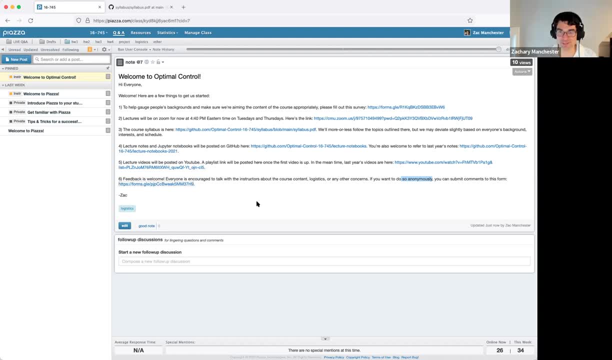 you should. I mean, basically, it's set up something like that and then you can do some like, if you just put the time in, like you'll know if you did it right, if you, you know, give yourself enough time, you should be able to go through it. you know, make sure you're passing. 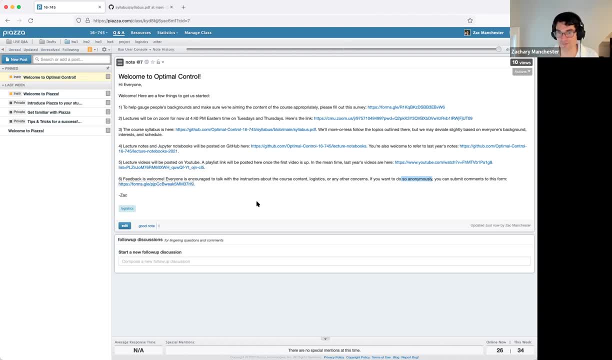 the test. if you're not passing the test, come talk to us in office hours and figure it out right. so I definitely I want you guys to succeed. we're not trying to trick you or anything like that, and as long as you kind of like put the time in, there's no reason you shouldn't be able to get. 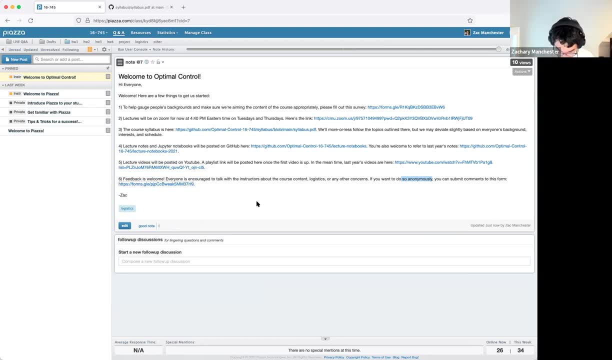 perfect scores on the homeworks. Cool thanks, Yeah, I have a quick question. Yeah, Are there any readings for the class Or like text or anything we should refer to? So there's, there's a bunch of optimal control textbooks. I can put post some of those as references, as sort of general references. 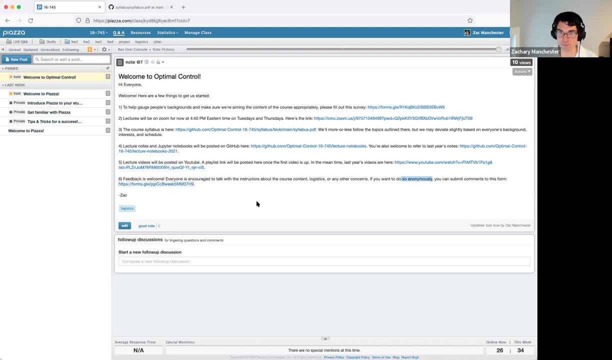 I'd say like I'm kind of taking a bit of a non-standard path through this. that's a lot more sort of like computational, you know, implementation focused, and there aren't really a ton of good books on that. A lot of stuff we're going to do, but there are definitely some good general. 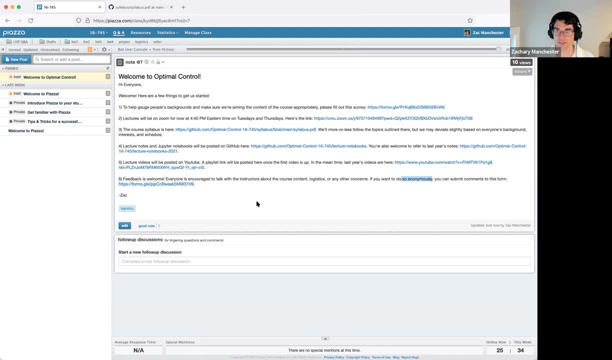 references and I can definitely like post some material And try to like, along with the lecture notes from each week, I can like definitely post some references to check out, to sort of like go deeper and look for more. So that's a good one. 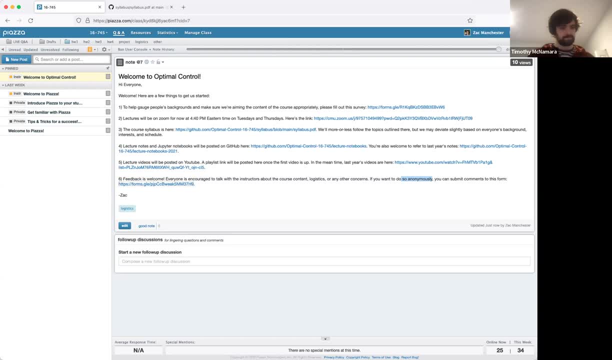 I will take that as an action. Cool thanks, Okay, yeah, For the quick question for the homeworks: what programming languages? Oh yeah, that's a very good one. So, Brian, would you mind taking that one real quick and we'll use your stuff from. 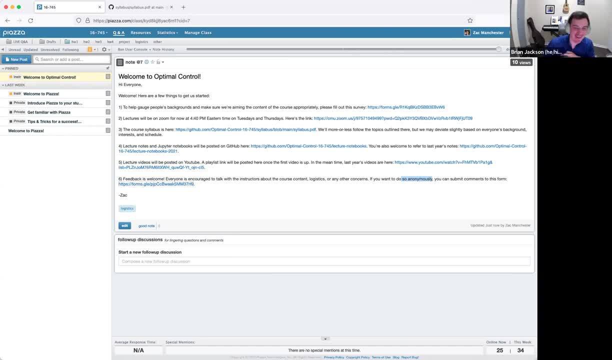 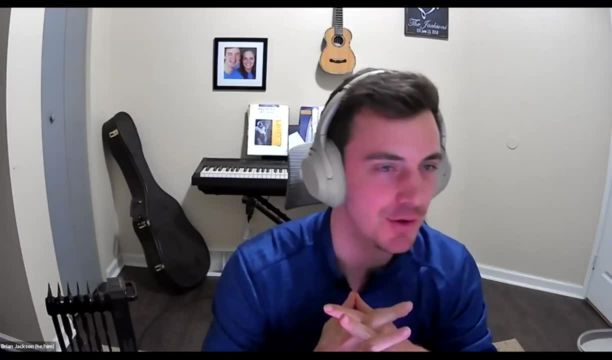 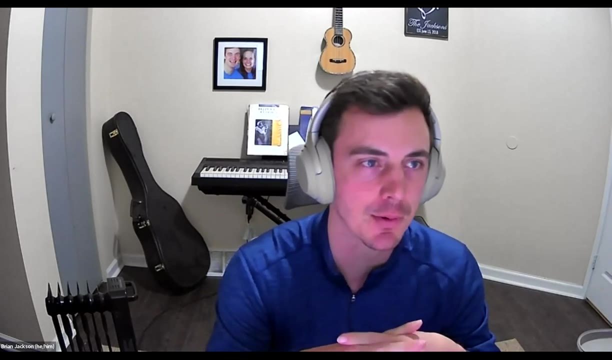 last time, Sure. So yeah, we'll be using Julia in this class. For those of you who haven't used Julia, which is probably a good number of you, it's very similar to MATLAB and it's very easy to pick up If you're coming from either MATLAB or Python. 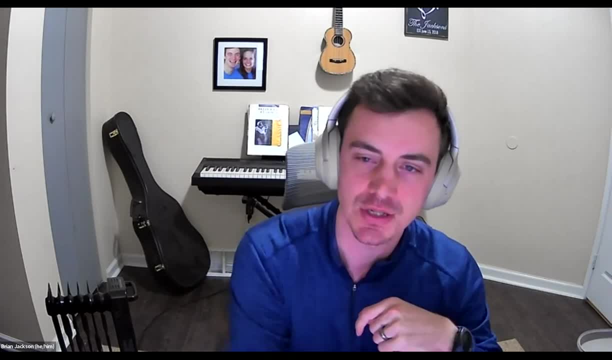 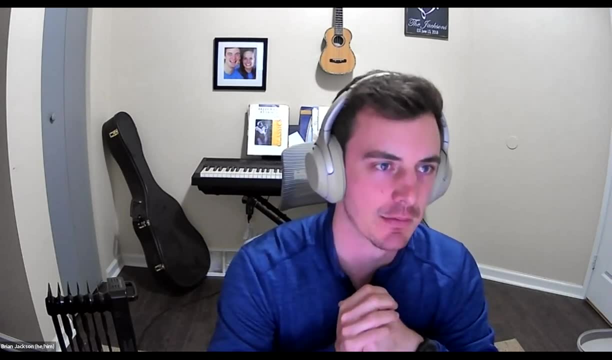 really don't worry about it too much, It should be fine. So I'll post a bunch of content to help you guys kind of transition from either one of those languages and get ramped up pretty quickly. So that gives you a little bit of a sense of where you're coming from. So if you're 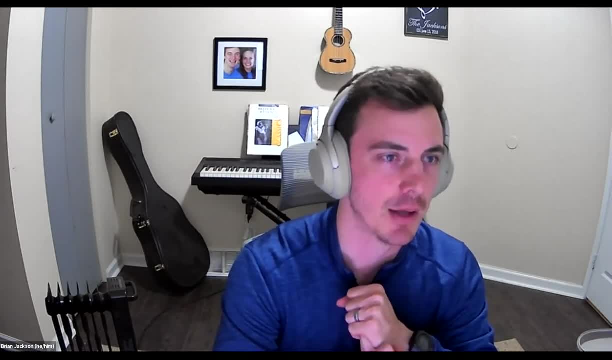 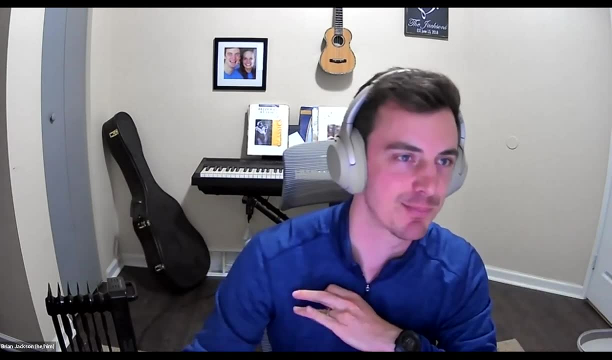 interested in learning a little bit more about how to use Julia. I'm sure you'll be able to do so, So I'll post all that on Piazza in the next couple days. And, like, I've been using Julia for a while since, like pre-version 1.0.. So like, if you. 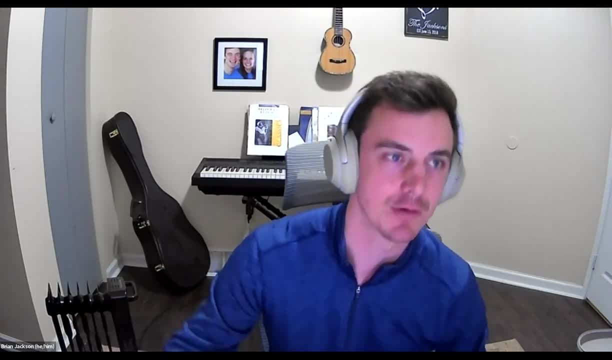 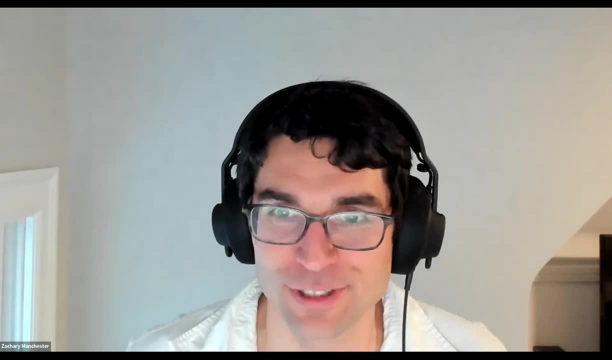 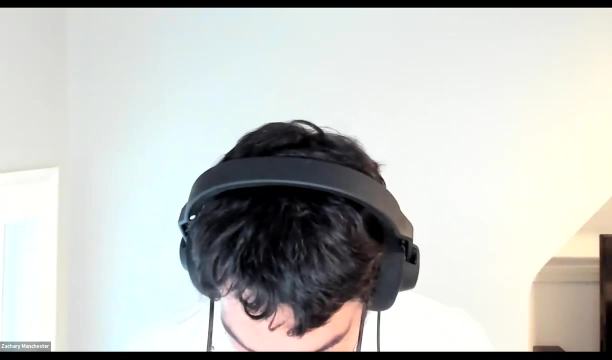 have any questions whatsoever like Julia related, please hit me up. All right, thanks, Brian. Brian is definitely our resident Julia expert. He's sort of definitely better than me, But yeah, it's. I mean, I came from MATLAB and for a long time I basically copy and pasted my MATLAB code into Julia and fixed the handful of errors that would come up. So it's ridiculously similar to MATLAB. at least you know the easy stuff, So it shouldn't be too steep of a learning curve. If you've done MATLAB, it's super easy. If you've done Python, it's pretty. easy. still There's a few more differences between. it's a lot closer to MATLAB than Python, but like it's really not bad. So as long as you've had experience in one of those or both of those, you'll be totally. 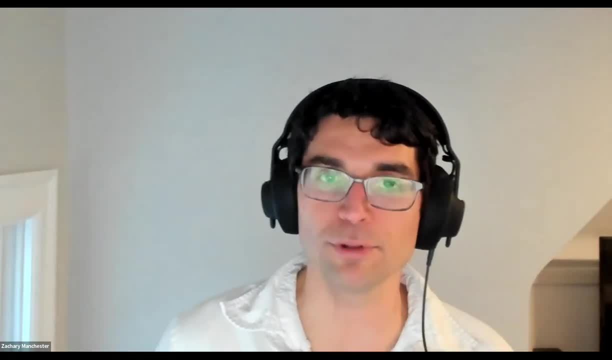 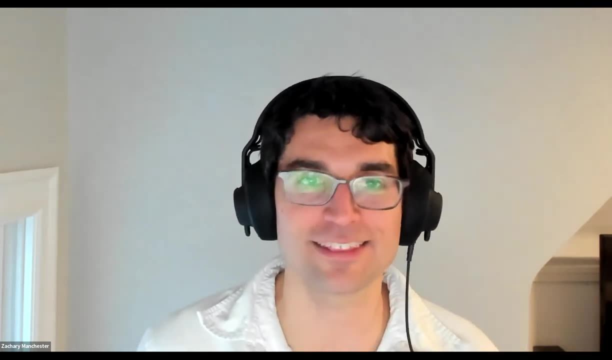 fine and it should be pretty easy to pick up And we're going to give you a lot of template, code and stuff like this with the homeworks, so it'll be kind of fill in the blanks. So, as long as you know how to do like array math, matrix math, using like MATLAB or Mumpai, it shouldn't. 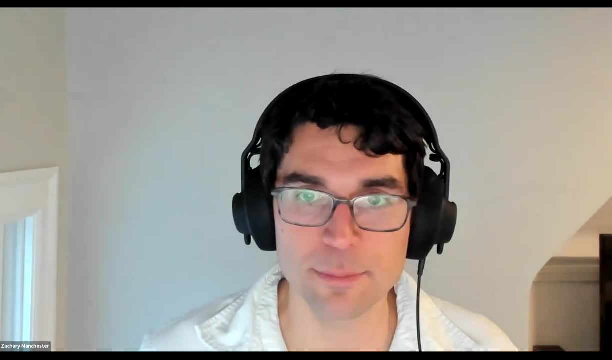 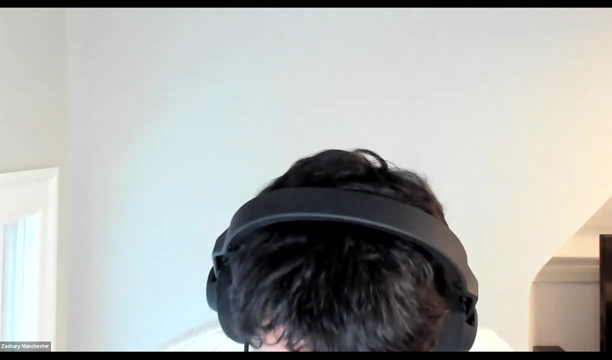 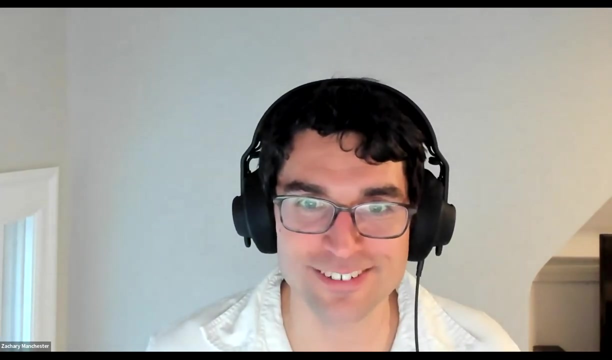 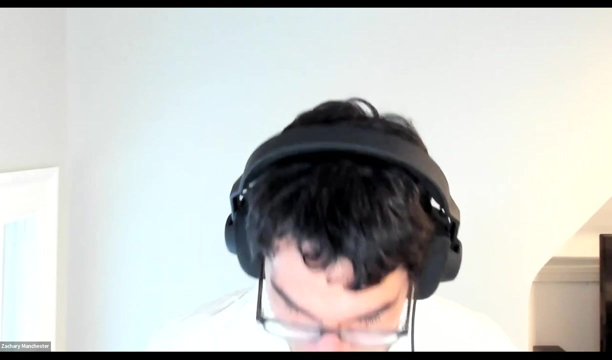 really be a problem. Okay, anybody else? All right? cool, So I'm now attempting to make my tablet work. This is a perennial challenge. It is always harder. the first time I haven't done this in a while, so here we go. Share screen start. 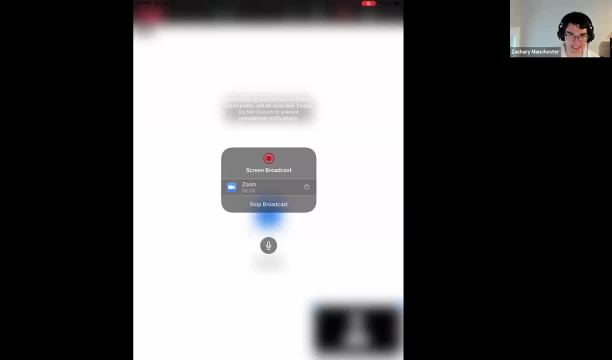 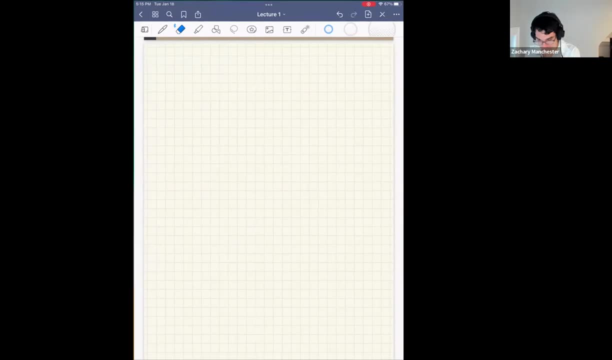 All right, I think it's working. Ah, cool, Hooray, We're in business, all right. So, and like I said, yeah, It's really going to be a lot of fun doing this, So it's going to be kind of a challenge. 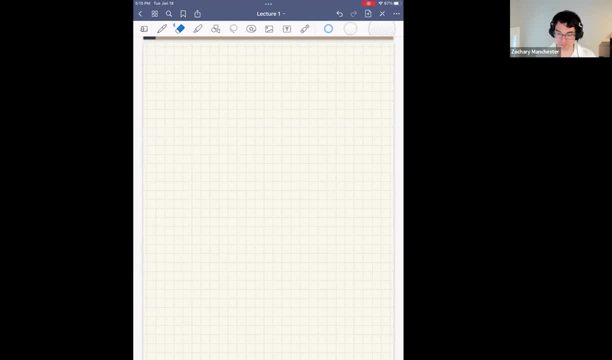 said: yeah, if you have questions while I'm doing this, just speak out, because I'm like off my own little world here looking down at things and I can't see the chat super easily, Okay, so what we're going to talk about today is kind of 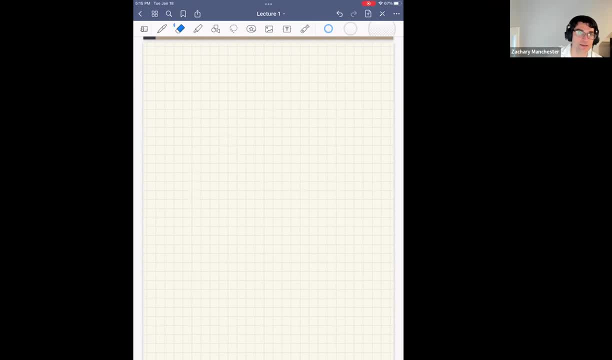 dynamics, I would say, I guess, continuous time dynamics, in particular, of controlled systems. So hopefully this is a review for most of you guys and you've all done some of this before. If you haven't definitely speak up, talk to us and we should be able to get you up to speed. 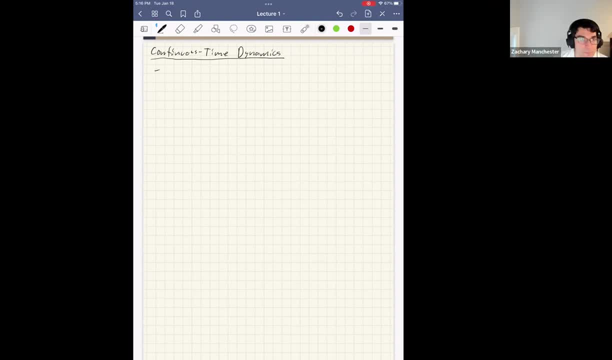 Okay, so the most general slash generic form for a smooth dynamical system is the general form. It is the following: So we have a first order vector differential equation that looks like this: So x here is generically called the state and this is a vector in Rn. 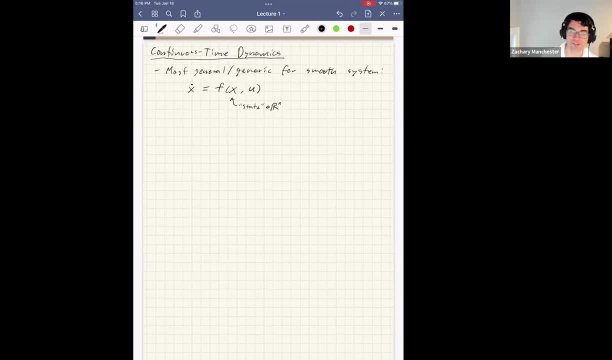 Usually it's a vector in Rn. Usually it's a vector in Rn, Although we usually make this assumption that it's a vector in Rn, but it's often not. In fact, most of the time in robotics it's not, but we still kind of assume this in a lot of cases. 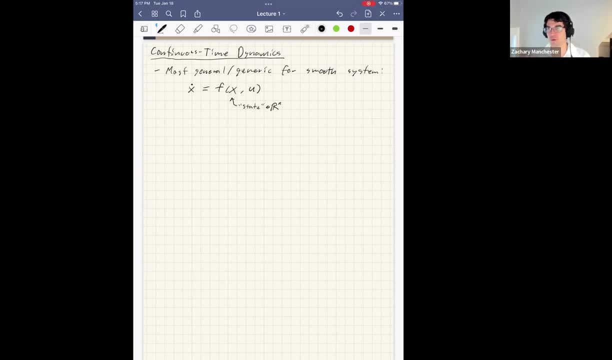 So that sort of positions, velocities, everything you need to describe where your system is and how fast it's going. So for most robots this would be like maybe the center of mass position and velocity, plus all the joint angles and the joint angle velocities, that kind of thing. 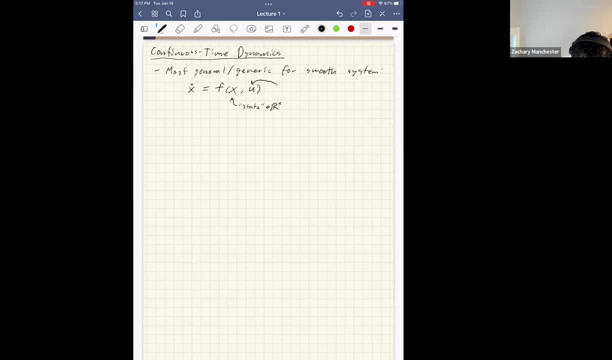 So that's state The? u here is called the input, And again, this is a vector, usually in a different dimension from. so we say Rn for this guy And this in our most robotic systems this would be like your joint torques. 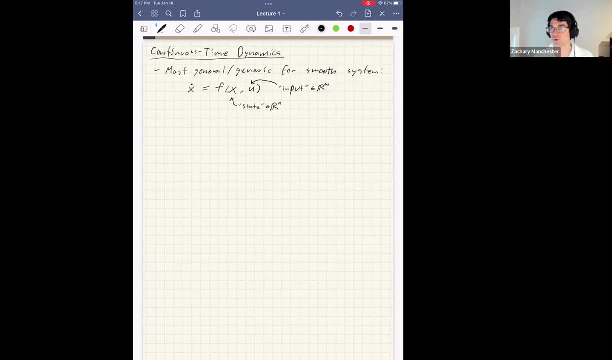 for example, on an arm or on a humanoid For a quadrotor. this is like the thrust from your propellers or the motor currents. if you want to go lower level, For, say, for a rocket, this would be, for example, a rocket. 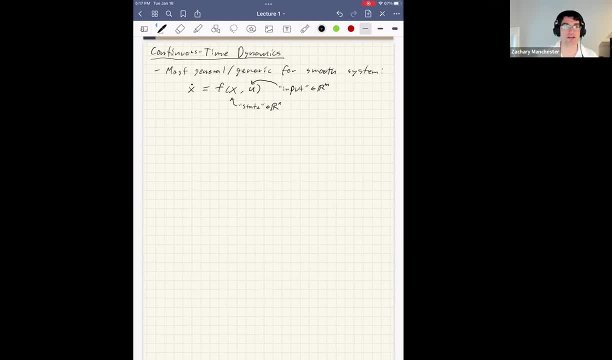 This would be like the thrust and the gimbal angle for the engines, This kind of stuff, right? So this is the stuff you have control over on your control system. And then x, dot, is actually obviously the derivative of your state. And then this thing, f, this f function, we call this function the dynamics. 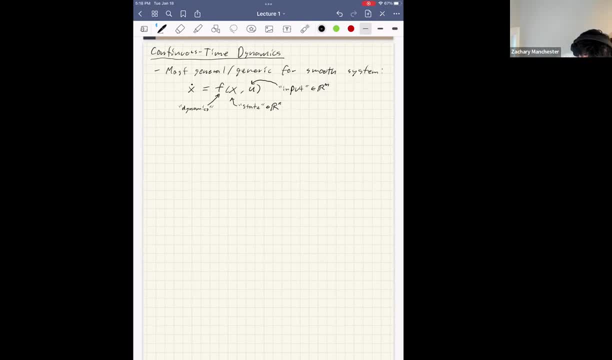 Right, okay, so that's. I think what we'll do is save both that. So for any smooth system, we can always write it in this form. This is super, super generic, but for a mechanical system, so most robotic systems. 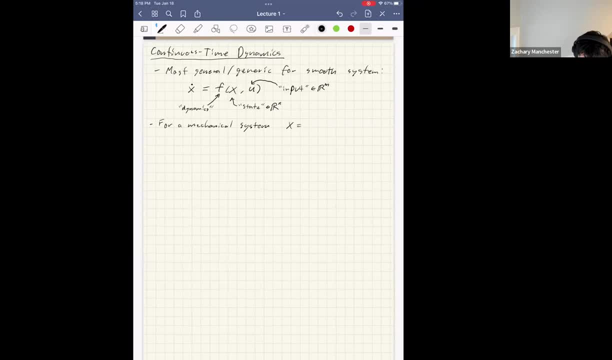 this looks: the state vector will look like what we call the configuration. So this is kind of position and or joint angles. We call that q and then the velocities v. So this guy is called configuration, This guy's and in particular this configuration q is not always. 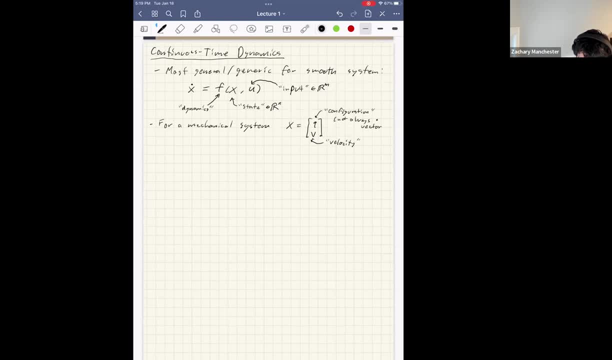 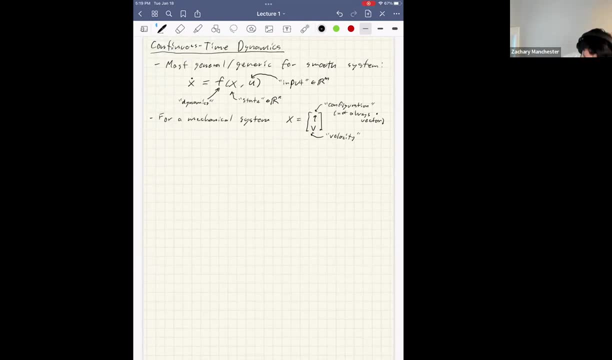 a vector. That's going to be important later, but v is always a vector. Okay, any questions about that? Okay, so we're now going to do everyone's favorite dynamical system: the pendulum. So I mean, I'm sure everybody's seen a pendulum before, so this is hopefully a super review. 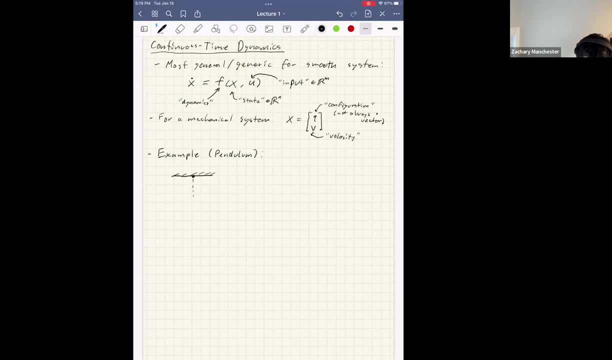 So this guy, we're going to do the classic thing. We've got, you know, some a mass m over here on the end of it. We've got the length l here, and then we've got an angle theta. 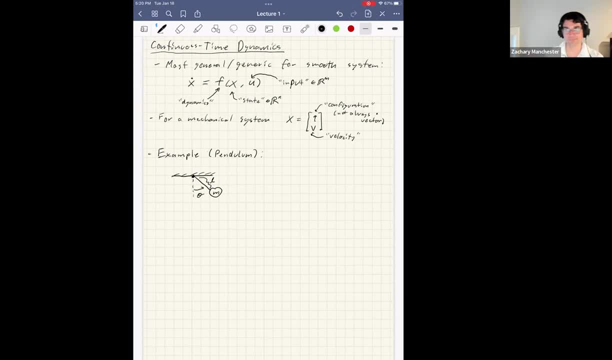 defined like this And if you do kind of your standard, f equals Ma, TORQ balance or Euler-Lagrange equation, however you want to do it, you get dynamics that look like this: m? l squared theta, double dot plus m g l sine theta. 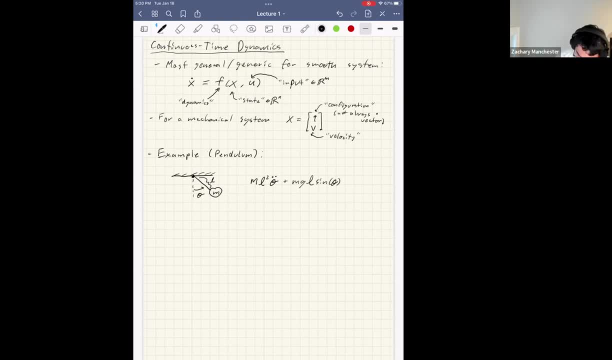 And we're going to assume, since we're in the controls class, that we have a control torque here, that we have an input, that we can actually do something to the pendulum. So we'll say equals tau. So we assume we have a torque about the base. 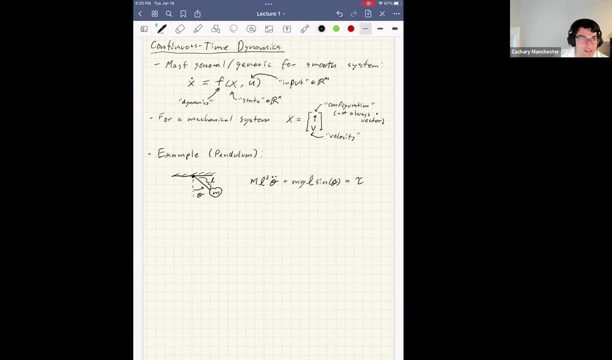 of the pendulum, the same angle, theta right there, And this torque is going to be. we're going to treat this as our control input u. So those are our dynamics And here. so, looking at our generic form of dynamics, there we're going to put this into that generic form. 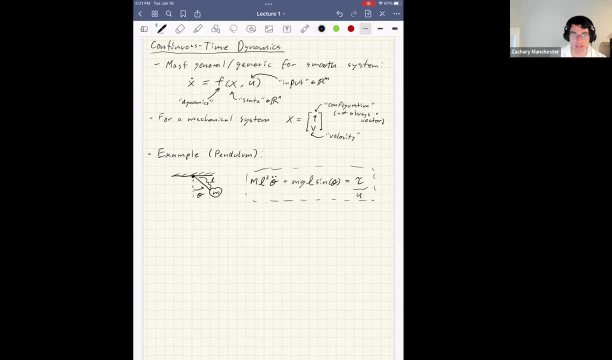 So to do that we need to define our configuration and our velocity and stack it up in that standard form. So here our configuration, q is just theta, the angle, And our velocity, v is going to be theta dot, And if we put this together we get: 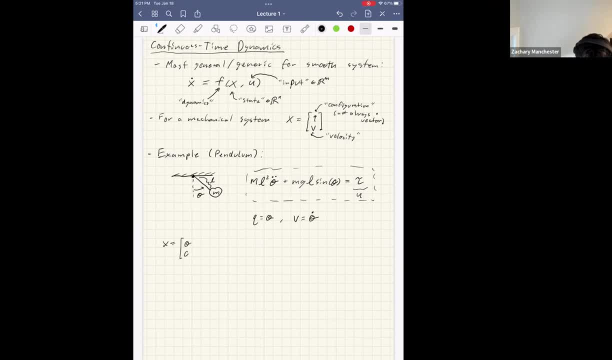 x equals theta, theta dot, And then our dynamics is going to be x dot, which here is equal to theta dot. theta double dot is equal to, So obviously theta dot. we've already got that in the state vector, So that's super easy. 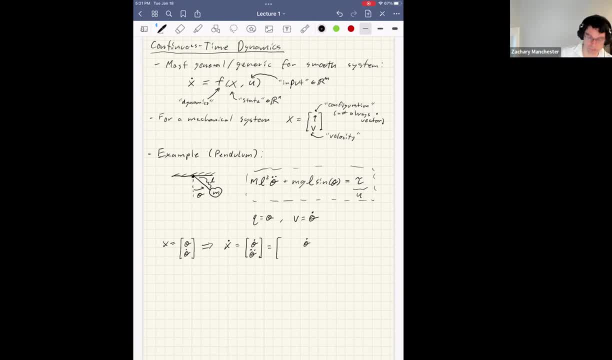 That's just theta dot And then theta double dot. we're just going to solve this equation in the box for theta double dot and kind of move things over. So we're going to get minus g over l sine theta, plus 1 over m, l squared u. 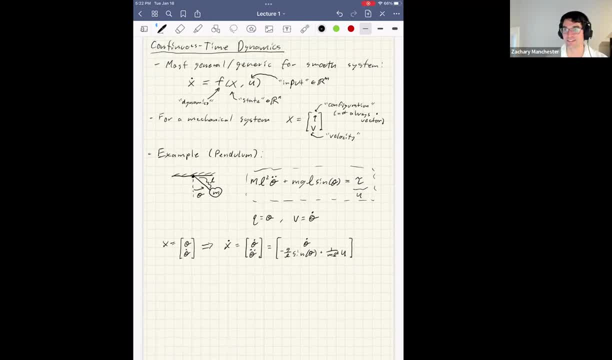 OK, any questions about that? So that's pretty straightforward. Everyone's seen this before. I'm hoping Here's the fun bonus question. So we said this whole thing about configuration is not always being vectors. Does anyone know what the configuration space actually? 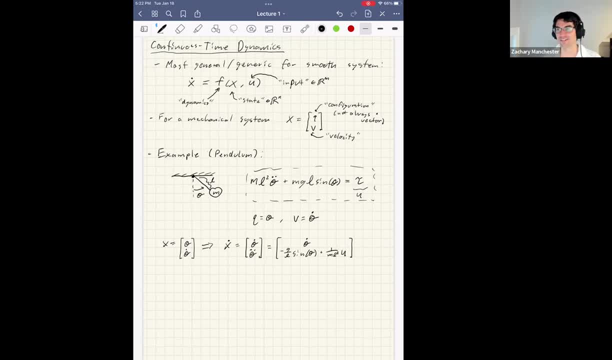 is for the pendulum. It's not r or rm. Does anyone know- Don't ask question, Depending on how you're- if you're saying there's a ceiling or not. it's sort of, I believe, s1.. Yeah. 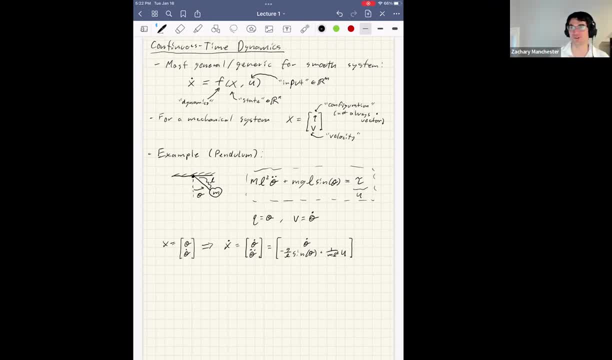 Just the circle Circle, Excellent. Yeah, so it's a circle, right? I mean, this is very intuitive stuff, But geometrically it's not the real line, right? And in particular it's topologically different from the real line because it wraps around. 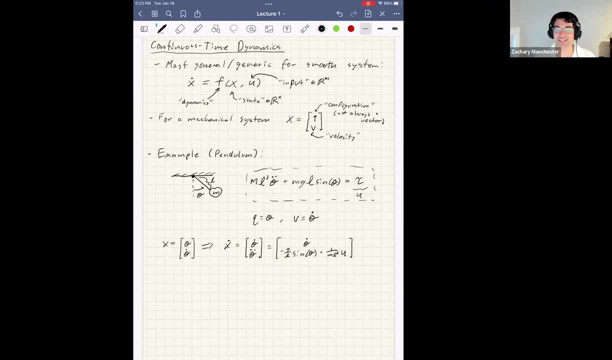 on itself, right. So this is actually kind of interesting. It's a compact manifold as in it wraps around. It doesn't go out to infinity, like the real line would. So actually here the q is not a vector, It's actually an element of this. 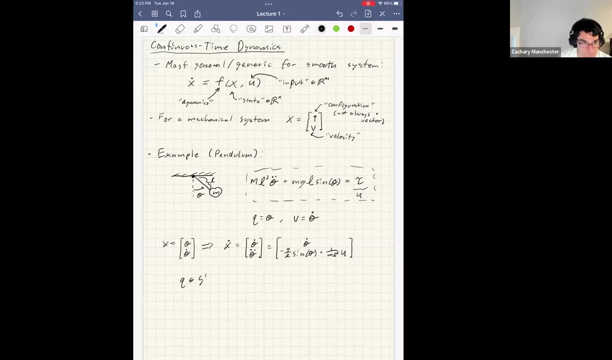 That's one circle And on that, what's the state space then? So we have the configuration space or configuration manifold. is the circle? What's the state space when I have both configuration and velocity? It's a torus, Yeah. 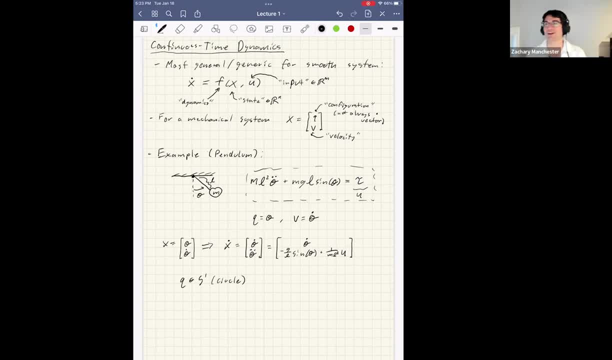 So why is that? Why is it a torus? Oh no, sorry, It's not. I'm sorry, That's wrong. Sorry, I wasn't listening. So it's not a torus, So remember. OK, so the configuration is a circle. 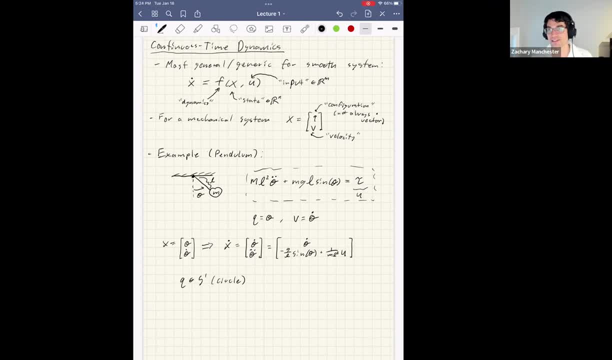 The velocities here are not an angle. The velocities are a vector in Rn, So in particular here they're just R, right. So think about circle. The velocity vector is tangent to the circle right. So it's this tangent line at any point on the circle. 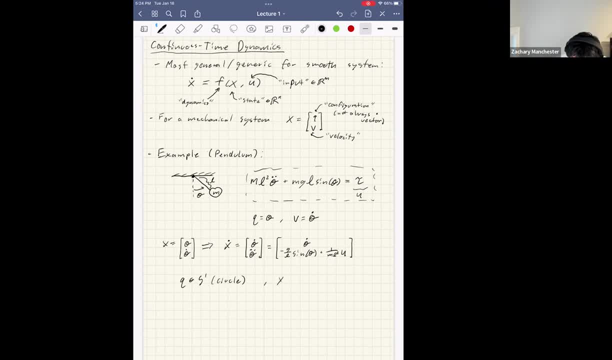 So actually that can be a vector. So if you look at the state space, here is actually S1 cross R. It's the circle, And then at every point on the circle the velocity is just R. So topologically, if you think about that geometrically, 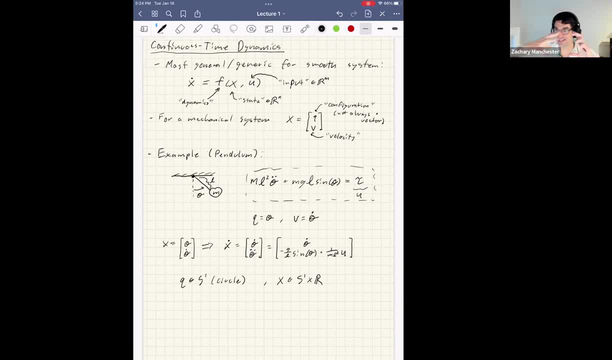 what that actually is is a cylinder. It's sort of a circle, And then at every point on the circle you get the real line. So you have two coordinates and that's the cylinder. All right, There's just fun facts that often don't get talked about. 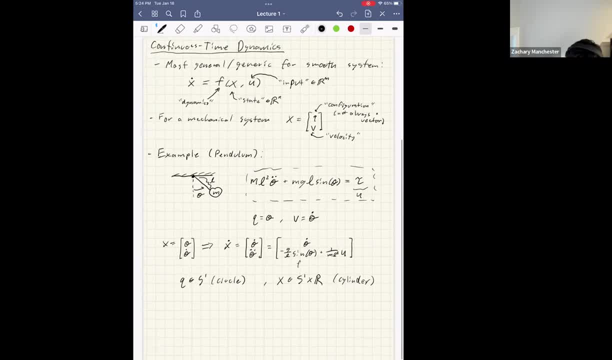 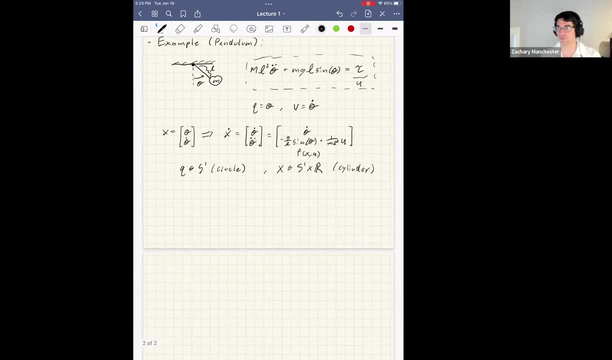 But they're, I think, interesting. OK, And yeah, this guy's next to you here. OK, cool, That was a fun little aside, But yeah, this shows up all over the place. So the torus- someone talked about that. 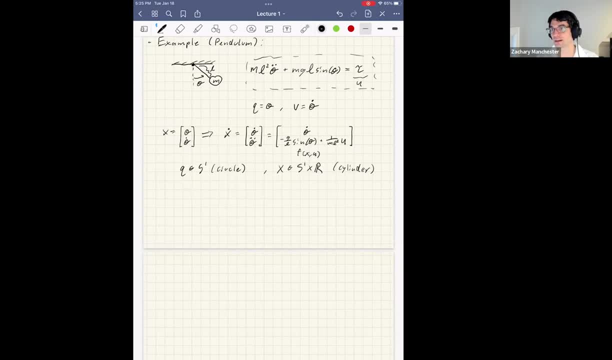 was torus is actually the configuration, not state configuration manifold for the double pendulum right, Because there you've got S1 cross S1. So you have two circles right, The first link and then the second link, And that, if you imagine, you have. 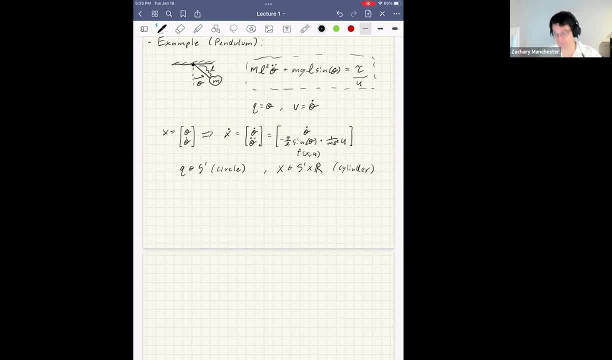 the circle and then every point on that circle you have another circle that makes a torus. OK, cool. So moving on then. enough random distractions from me, All right, So now we're going to talk about a slightly more sort of specific class of system or restricted class of system. 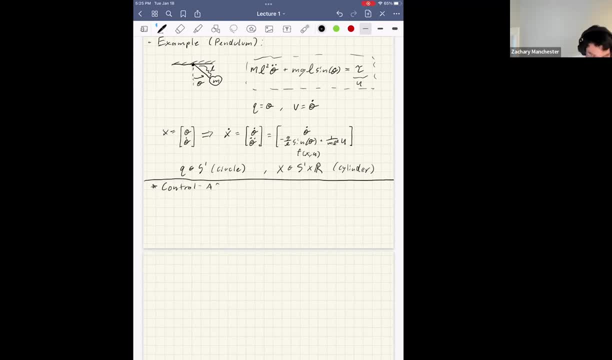 called control affine. OK, So these look like the following: x dot equals- we're going to call it f0 of x, which, importantly, this is only a function of the state plus what should we call this? We'll call this d of x times u. 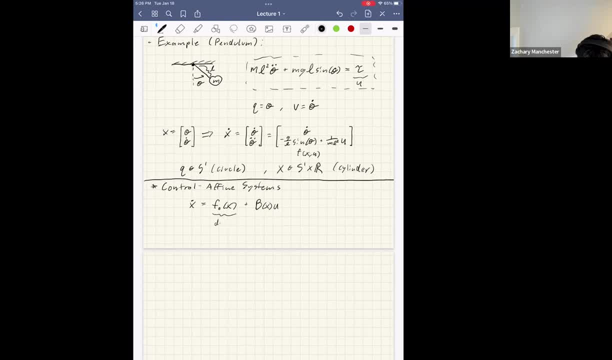 So this f0, we call the drift, And then this is called the input Jacobian, And then this guy is called the input Jacobian. So we call this control affine, because in the control input u this is affine. right, It can be totally nonlinear in the state. 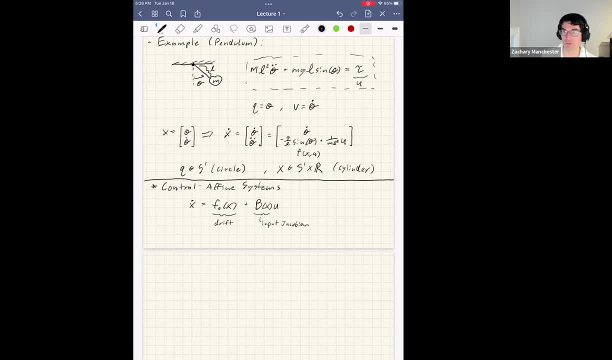 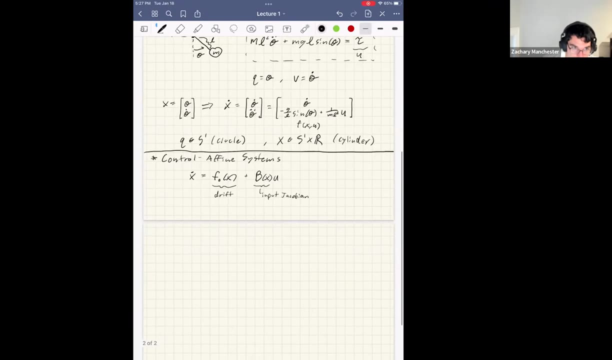 So f0 of x can be totally nonlinear, b of x can be totally nonlinear, But b is a matrix, right, And that multiplies u In terms of just u. this thing is control, affine, And the interesting thing about this: 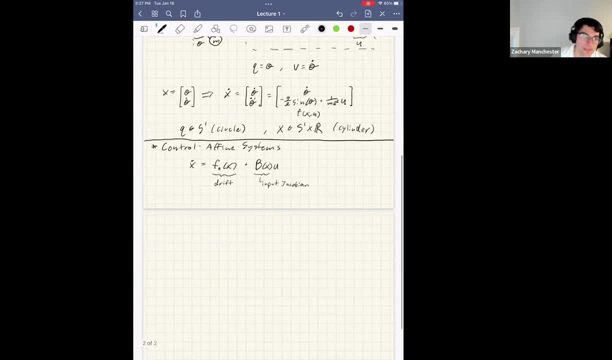 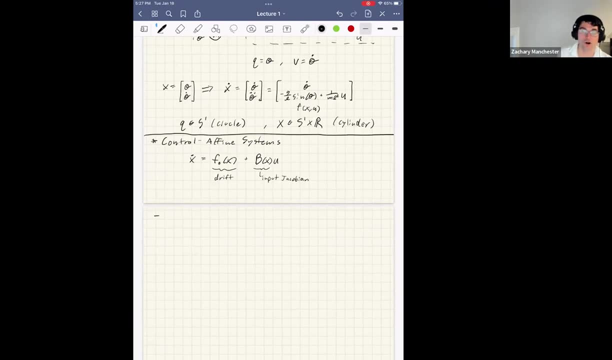 so this has a lot more structure than the first problem, right, And it turns out that most systems can be written this way. In particular, all mechanical systems can be written this way And I would say actually, I think, any smooth system. 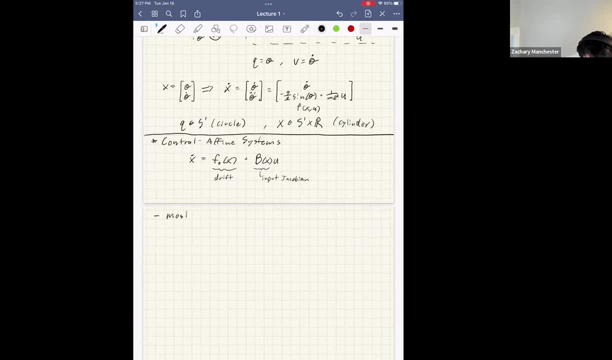 basically you can write this way And this has some important control implications. So you're going to know, if I have a system that doesn't look like this, there's a trick for rewriting it in this form, So like if I have sort of weird nonlinear coupling. 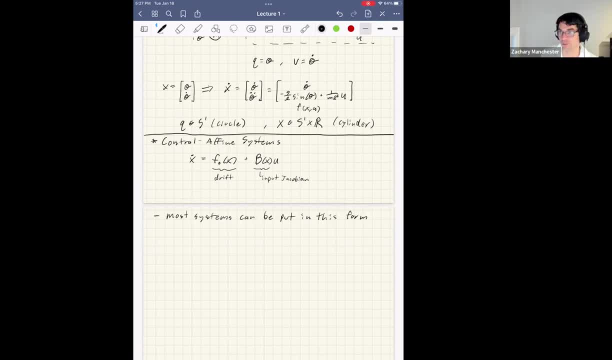 between an x and u. there's a trick, mathematical trick, at least right Right- where I basically introduce new states that correspond to my original u And then I make my new control input the derivative of whatever u was before, And if I do that it becomes control affine. 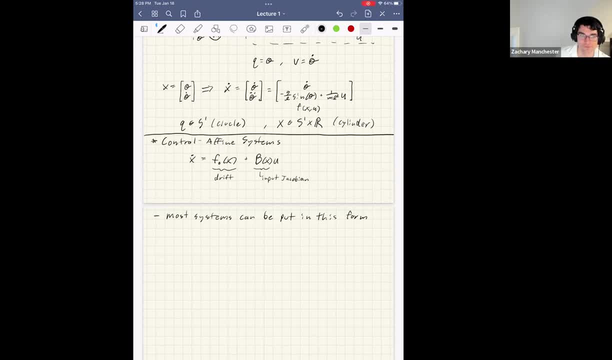 So there's always mathematical tricks you can play to put- not control- affine systems into this form, as long as they're smooth and differentiable, and all that good stuff. So if we do this to our pendulum, here's what that looks like. So I'll put my pendulum in this form. 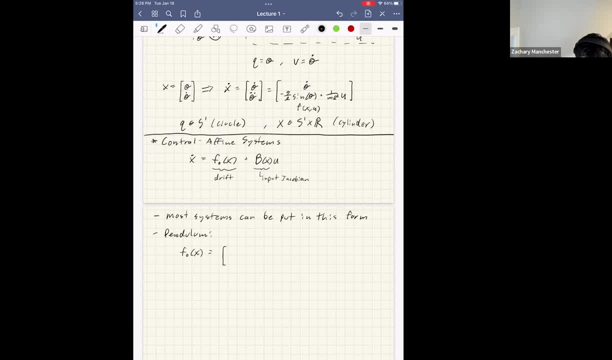 f0. then is going to be theta dot up here, no problem. And then the g over l sine theta term, And then this b of x guy is going to be 0. And then 1 over ml, squared Down here. so it's whatever was multiplying with u up top there. 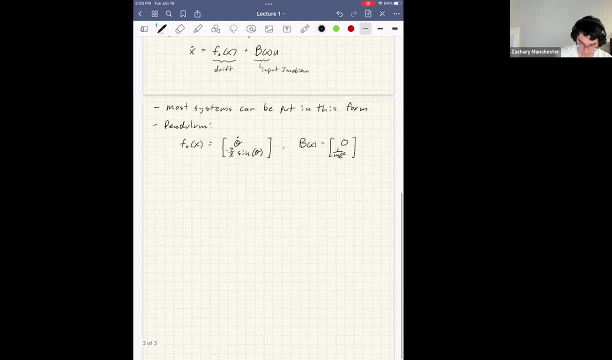 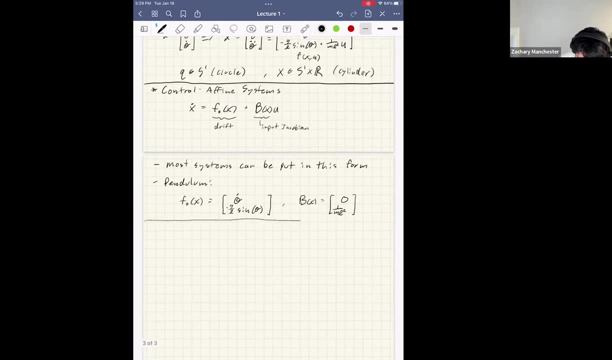 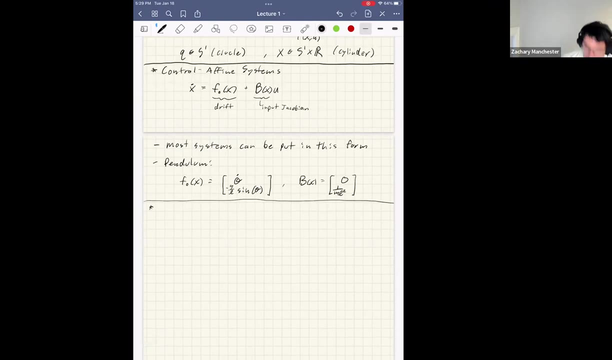 So makes sense to everybody. OK, so that's that. So next up is one that, if you're a robotics person, you've almost certainly seen. If you've taken KDC, I know you've seen it. So this is manipulator dynamics. 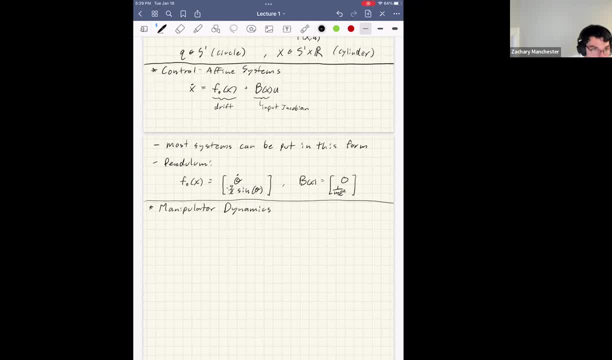 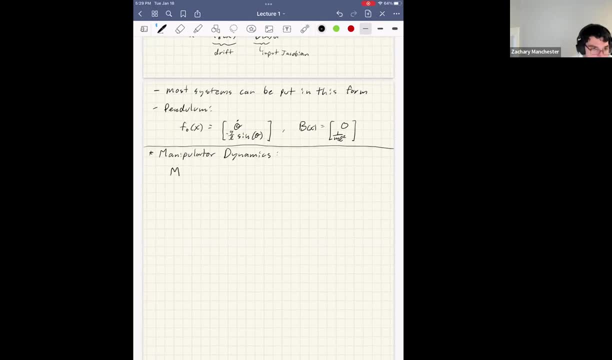 And this looks like the following: There's several flavors of this that you'll see, But we're going to do this a particular way because that's what our dynamics toolbox that we're going to use how it does it. So this is what this looks like. 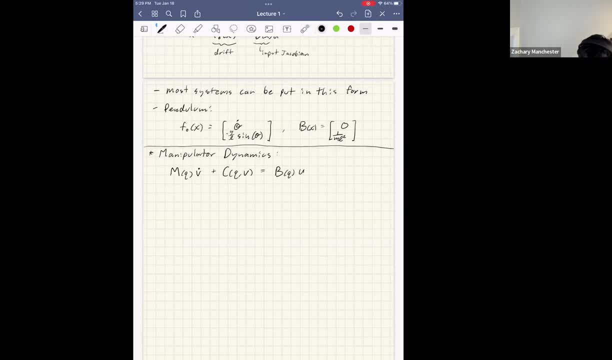 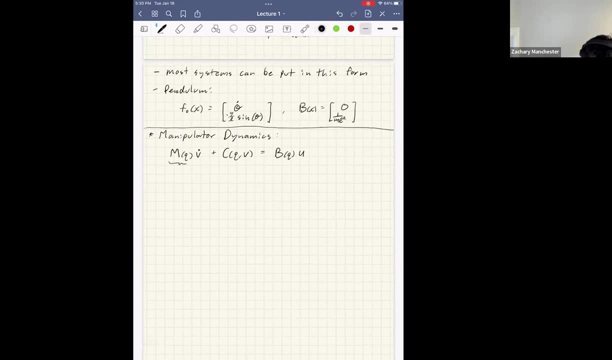 This is maybe bad notation overload. OK, I'm loading on my part, but I don't know It happens and this is what people do, So we'll go with this, OK. so this m guy up here is called the mass matrix. 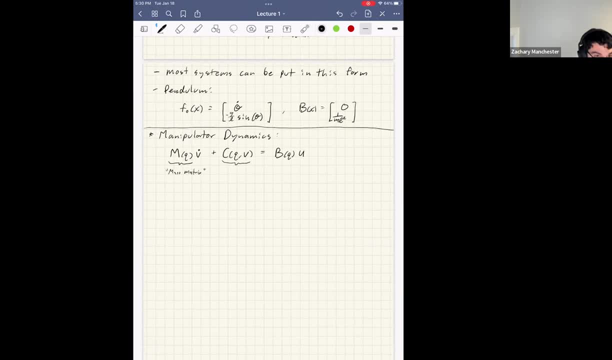 This c guy here is called the dynamics bias, or dynamic bias or just bias, And this includes, like, for example, your Coriolis terms, your gravity terms. People often wrap damping terms in there as well, And there's a few ways to write this, but this is sort of the one. 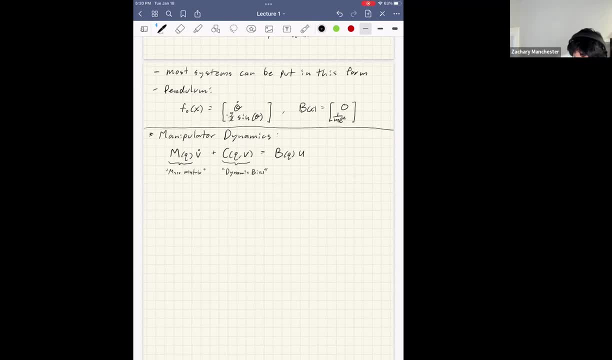 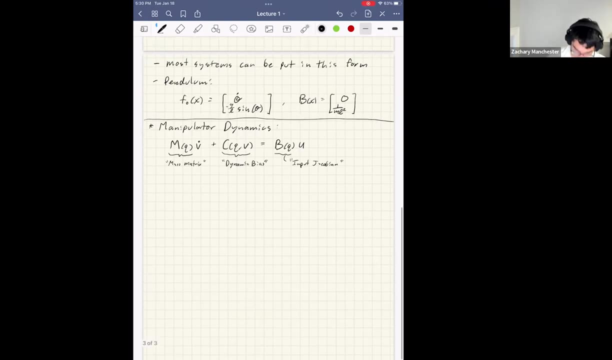 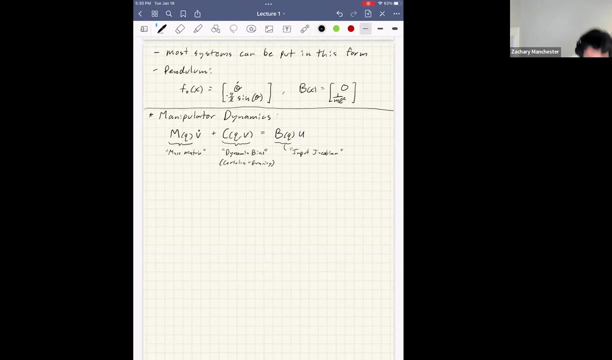 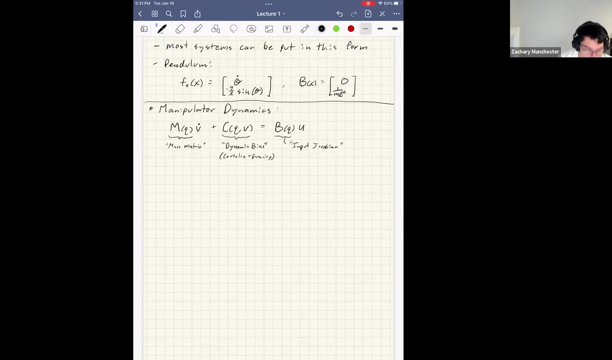 that the toolbox we use in Julia uses. so that's what we're going to do. This thing, once again, is called the input Jacobian And the rest of this stuff. you know what it is. I think It's a little bit of a. 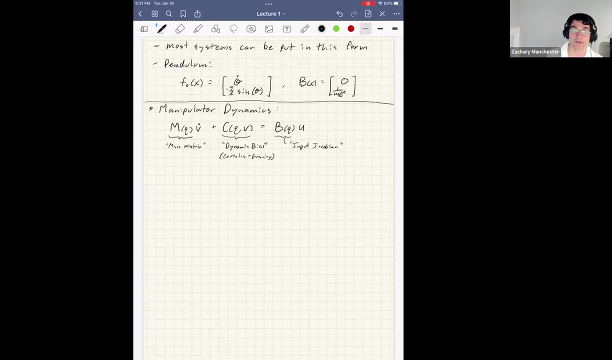 OK, so this is the dynamic stuff, And then often we will also have sort of a second piece of this. So notice this: lets us solve for the accelerations, right, So v dot accelerations. We still need to solve for the q's. 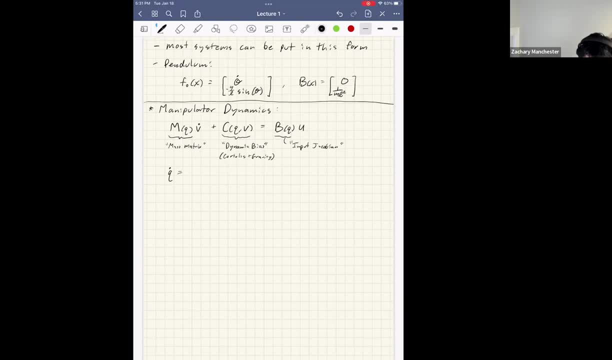 So how we get those? We need a second ODE and that looks like this, and a lot of times we don't talk about this. We will, because I hope it'll show up later- and these we're going to call this the velocity kinematics. 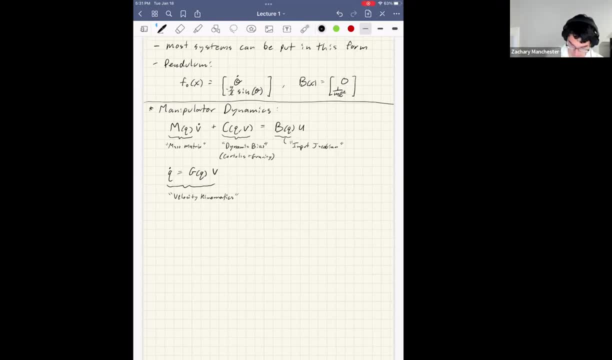 So a lot of times the Jacobian in there, that g of q is the identity. So a lot of times we have, you know, v equals q dot and then this is kind of trivial and often we don't even bother talking about it. but many, many times that's not the case and there's sort of a Jacobian in there and in. 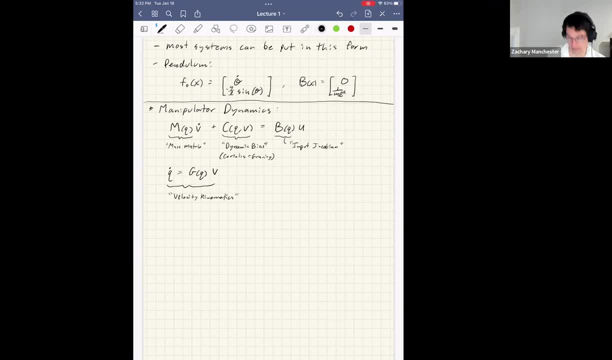 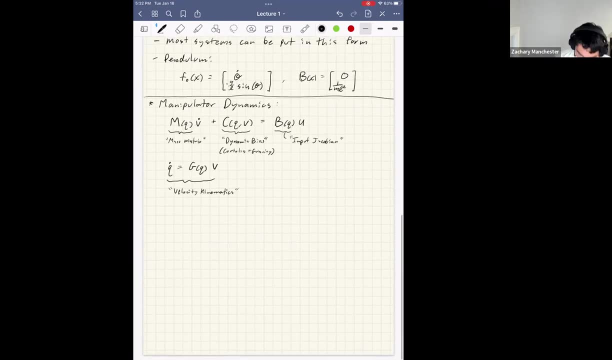 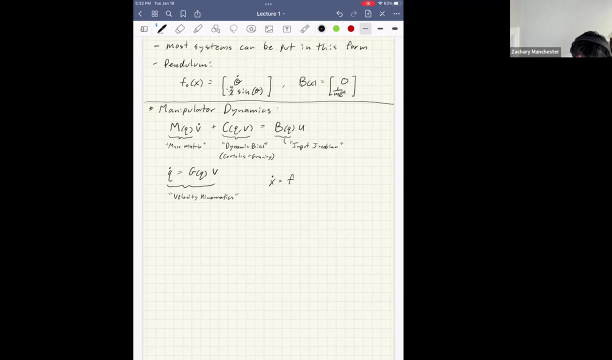 fact a lot of times v and q dot are different dimensions. that happens, but for example we have attitude dynamics going on. Okay. so if we have a system in this form, we can always kind of put it in our kind of more generic form. So the velocity stuff is just g of q times v, right, and then the other stuff. we just take that. 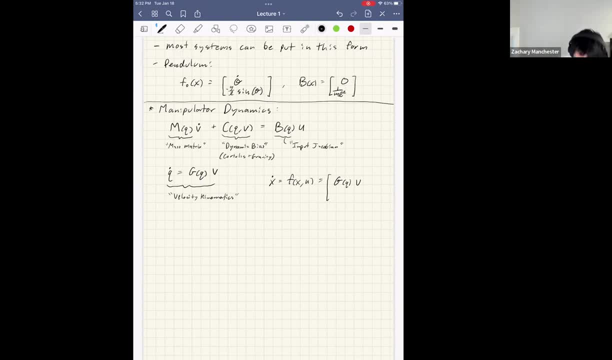 manipulator equation and solve it for v, dot, So that we just kind of move everything over. we're going to get minus m of q, inverse times b of q, u minus c, and I'll leave out the details there, the arguments. Okay, so going back to our pendulum and kind of writing it this way: 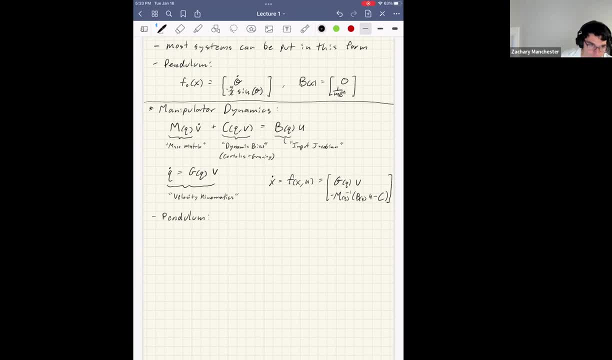 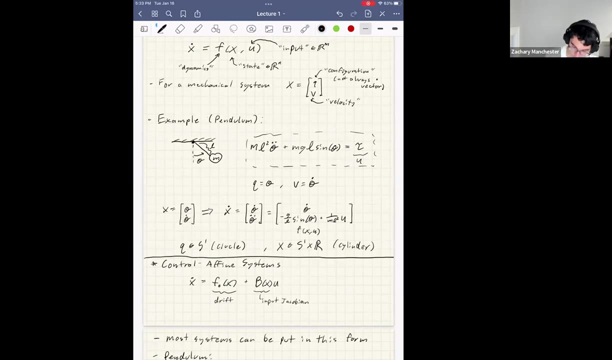 it's pretty. you can kind of sort of squint at the equations up above and kind of see what these terms are. So m of q, here is just m l squared, and you can see this up here right? so it's the thing. multiplying v dot. So our v dot here is theta double dot, so m l squared. 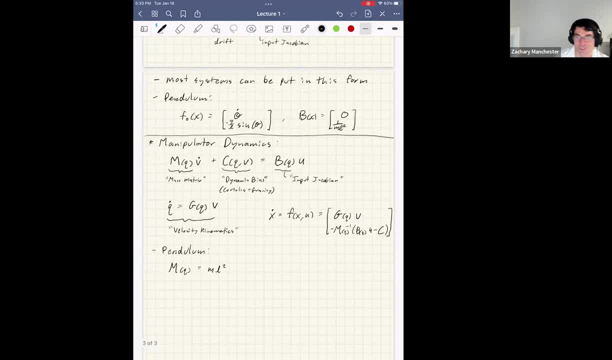 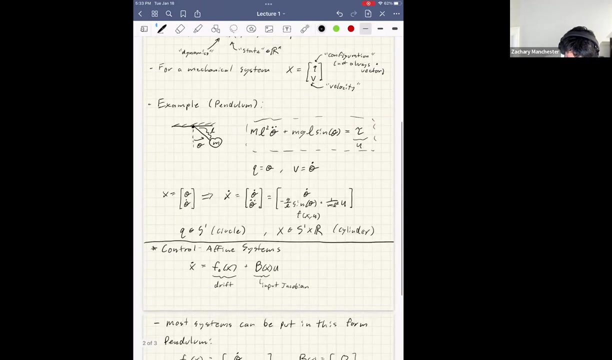 It is the mass matrix, or generalized inertia tensor. if you want to be fancy, The Coriolis term or dynamic bias term, here the c is our, is basically the other term there. so gl sine theta, So the other term from up here, right from this guy, and then 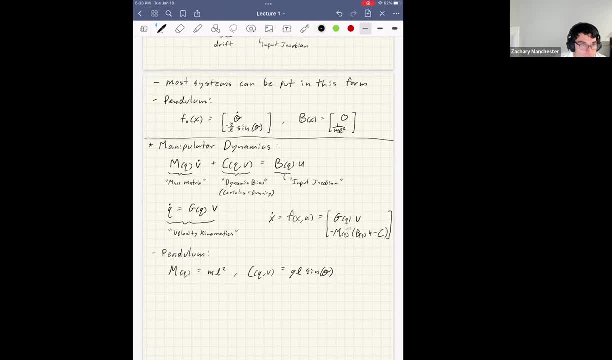 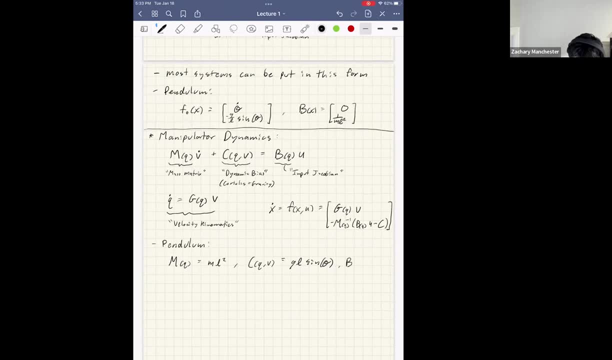 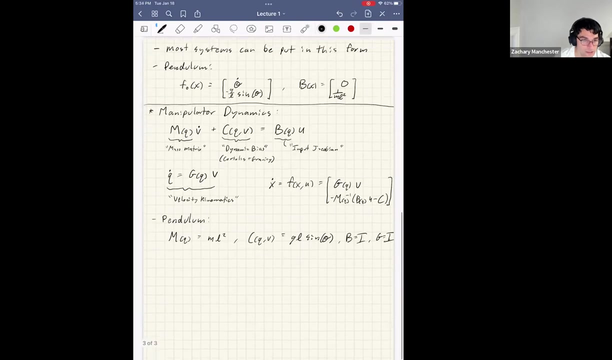 what else we have right, and then the other stuff super easy. So then the b here is the identity, and because q dot equals v, here we're just using theta dot for v. that kinematic Jacobian guy is also the identity, Okay, so any questions about that? 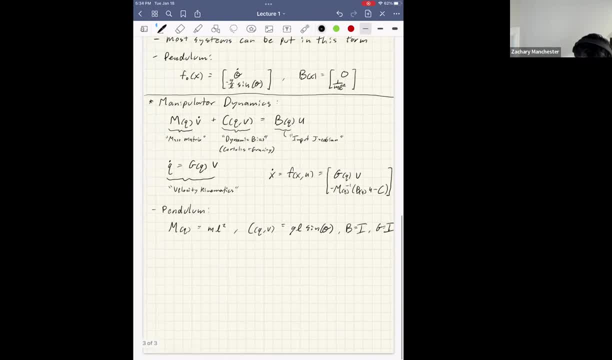 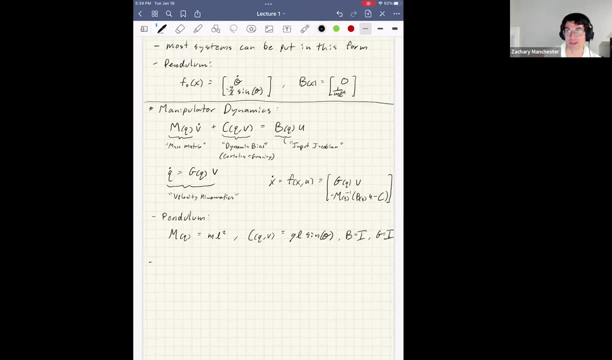 All right. and the last note on this is that all mechanical systems, every mechanical system you'll encounter, pretty much every robot, can be written in this form: manipulator form. So this shows up all the time: super useful. Does anyone know why that's true? 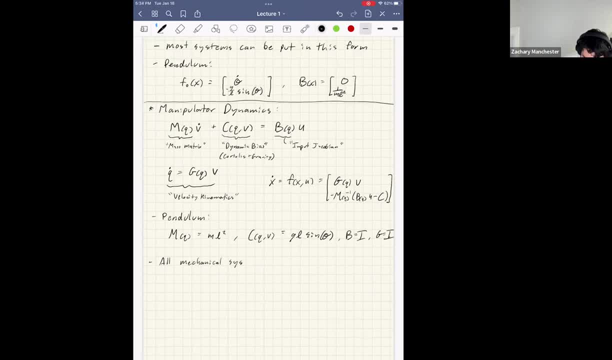 I think. so Take a guess. I don't think you're gonna get a good answer. So I think you're gonna get a good answer. I think you're gonna get a good one. Take a guess. I don't think you're gonna get a good answer. 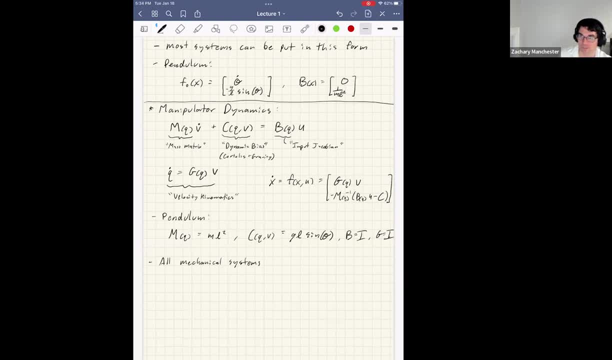 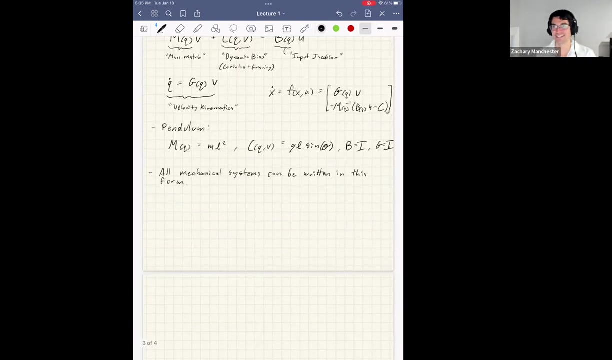 most of you guys have seen this before, so anyone know where this comes from or why this should be true. like, why can I always do this for a robot? Someone, someone make a guess. No one has any thoughts Killing me, All right, so this will be. I'll make this a bonus question. If anyone can like work this out, I'll give you. I'll tell you why, basically, but then if anyone actually wants to work out the detail, 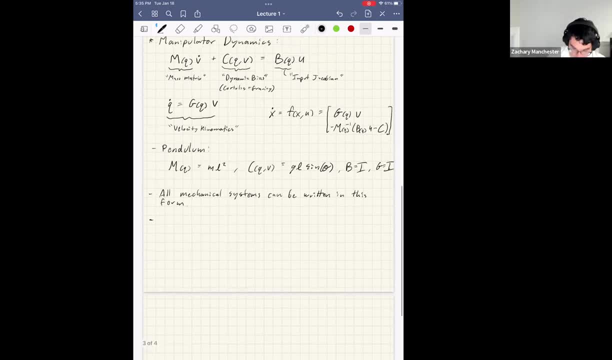 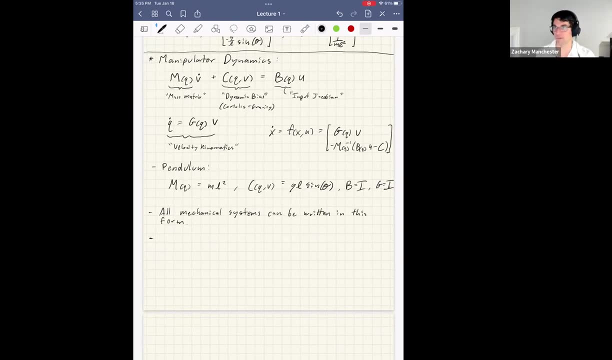 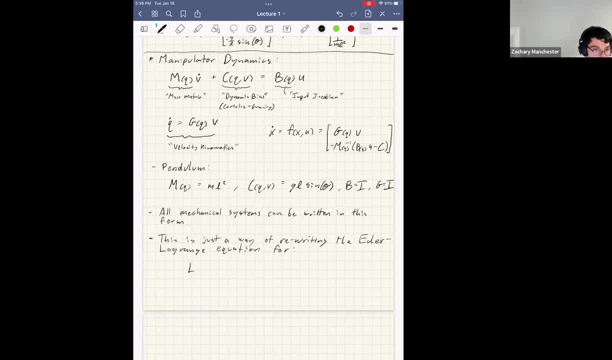 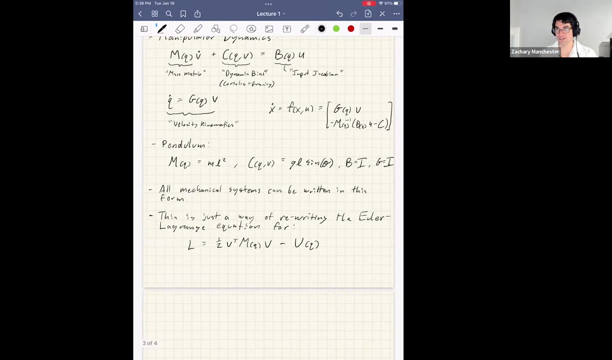 So in particular, if you're Lagrangian, equals one half v. transpose m of q v like the usual m v squared thing minus like a potential. if you turn the crank on that and just plug it into the Euler-Lagrange equation and, you know, simplify it down, you'll get the manipulator equation. So if anyone does that and actually cranks through this, you get bonus points. 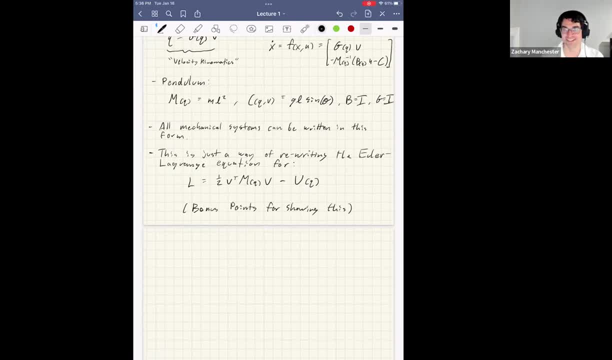 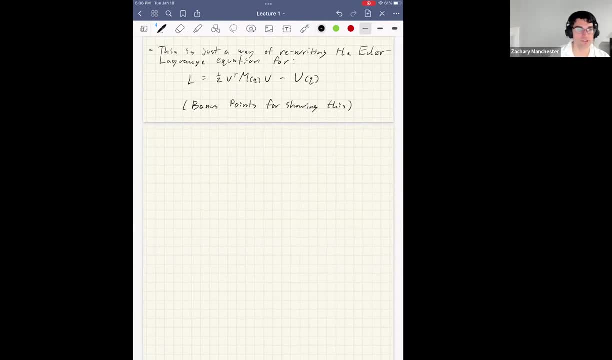 Okay, any questions about anything? All right, so let's see. Now we should talk about linear systems. So we're kind of going from more general to more specific, and this one is basically the bread and butter of control. So there's lots and lots to say about linear systems. 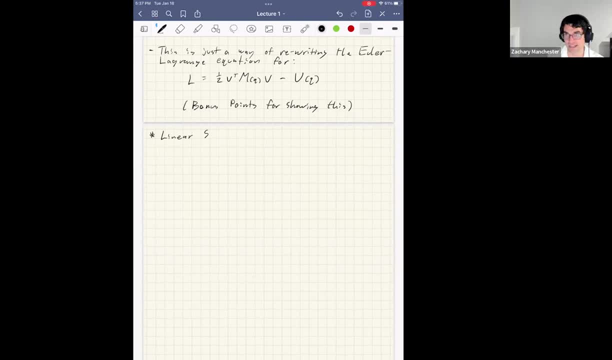 And there's entire courses on linear systems. If you really want to get into this field, I highly highly recommend taking a linear systems theory course at some point. I know there's one in ECE here And you can go through that in depth on these guys, but you should know the basics. So just in case you haven't done a ton of this before, Here's the basics. So a linear system looks like this. 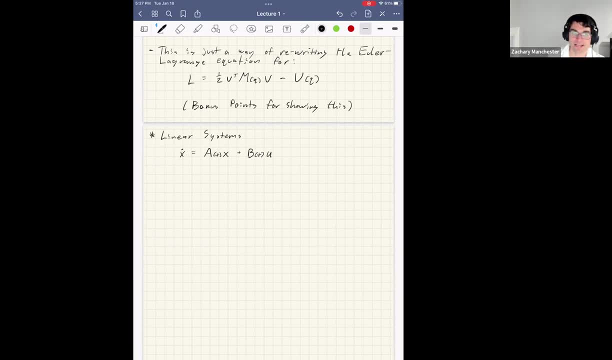 So x dot equals a times x plus b times u, where a and b are matrices. I put time arguments on them because they're allowed to be functions of time. There's a few cases here, So the linear system is called time invariant. 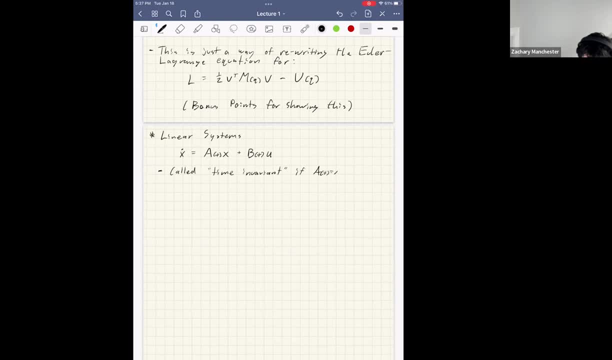 If a of t equals just a, some constant a and b of t equals some constant b for all time, it's called time varying otherwise. So if those things do vary in time, it's sort of obvious. And there's some other interesting cases you can get into as well. 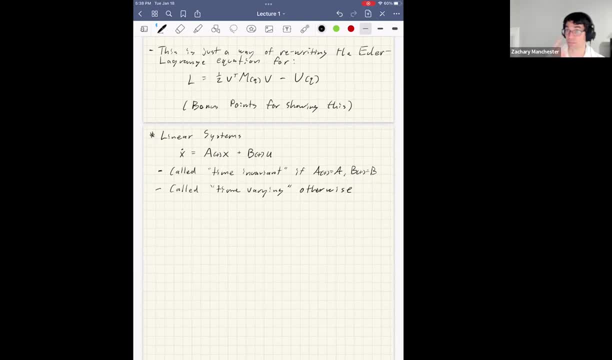 For example, you can have linear periodic systems where, like a and b of t are actually periodic, with some period capital T. That can be interesting. That actually shows up a lot in walk-in systems, for example. So if you're a walking gate, a periodic walking gate, you can end up sort of 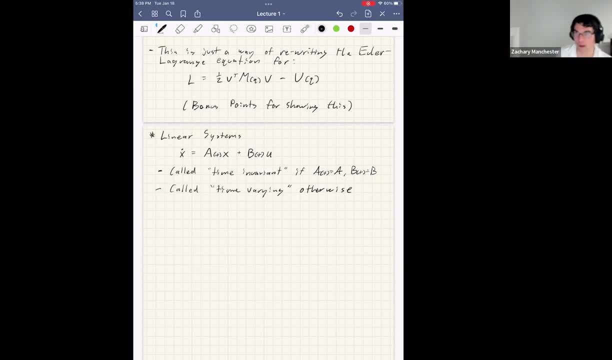 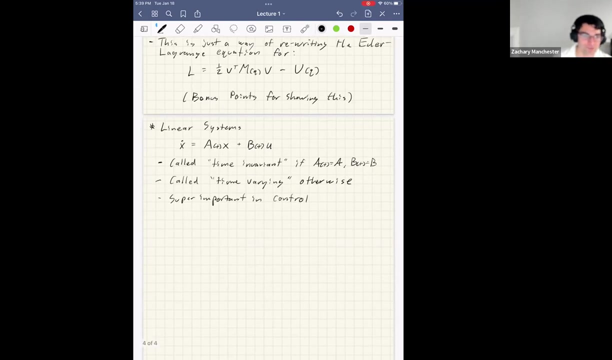 turning that into a linear periodic system and there's special properties there that you can take advantage of. These are kind of like a kind of super, super important in control, in control theory and control design. So they're everywhere And that's for sort of very practical reasons. 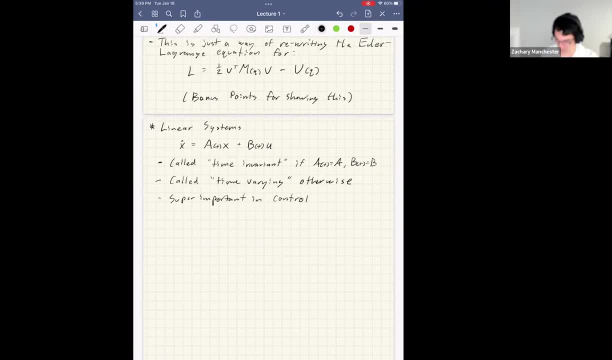 These are the only systems we know how to. we always can solve right. We can always solve linear systems, And that's not true of most other things. And yeah, that's sort of why that's the case. And so, because of that, because there's like 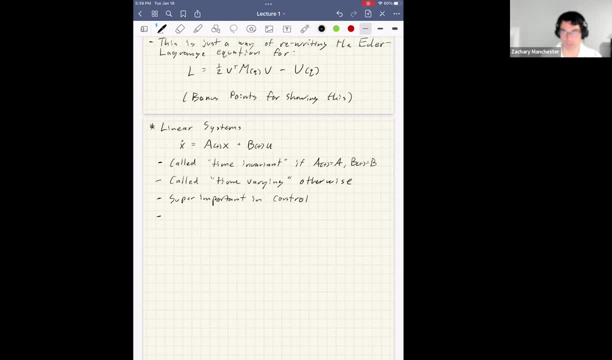 a whole well-developed theory for these things. we essentially can know everything there is to know about any linear system, right? So we often approximate non-linear systems with linear ones as follows: So if you've got the generic nonlinear system, x dot equals f? u, you can linearize this and do: a is partial f, partial x, right? Take the Jacobian. 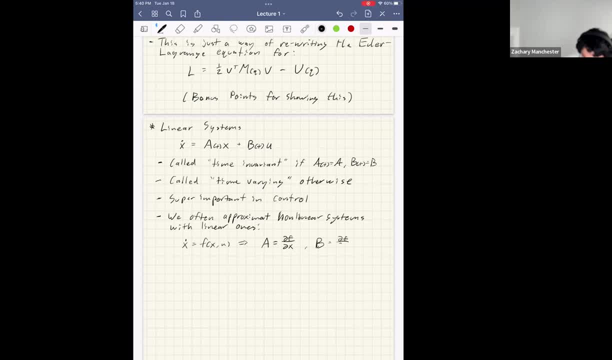 And b is letter a, A, partial f, partial u, and you can do all kinds of fancy things. obviously you need to evaluate those derivatives somewhere right so you can do this whole bunch of ways. there's all kinds of tricks, but if you can play this game, then you can take advantage of all the standard control results for 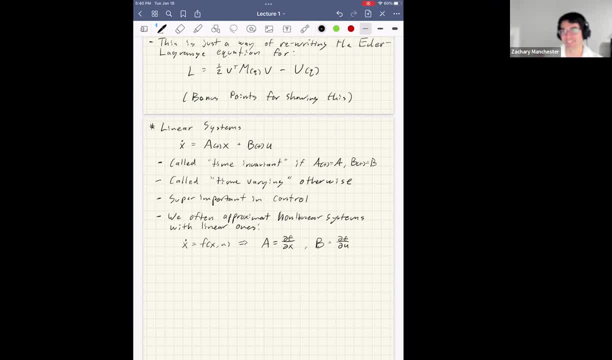 linear systems and apply them to non-linear systems, and that is really kind of the name of the game most of the time is to is to somehow take your crazy system and smoosh it into the form of a linear system where we know how to do things. yeah, one of the sort of founding fathers. 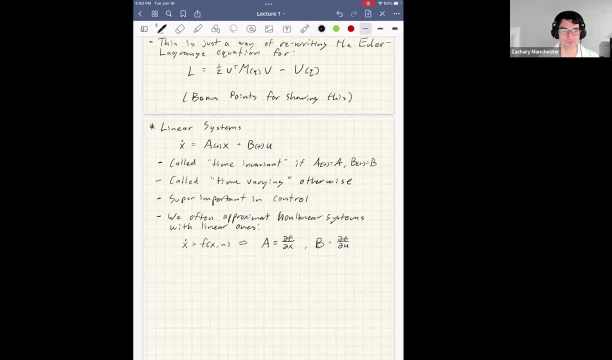 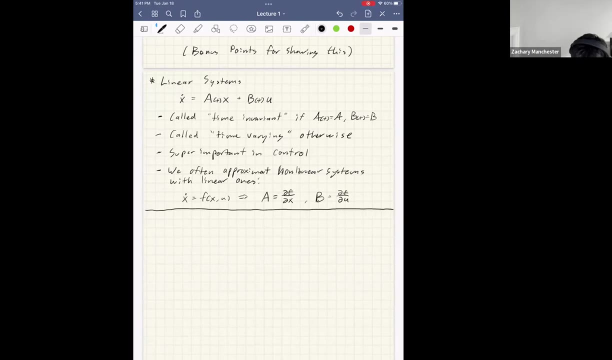 of control, Bryson. Art Bryson, who you will, you will, whose name will come up again- had a quote that was like one of his books, somewhere or something called that was: be wise, linearize, okay, cool. so that's that's sort of, I think, roughly all we'll need for dynamical systems: continuous time dynamical. 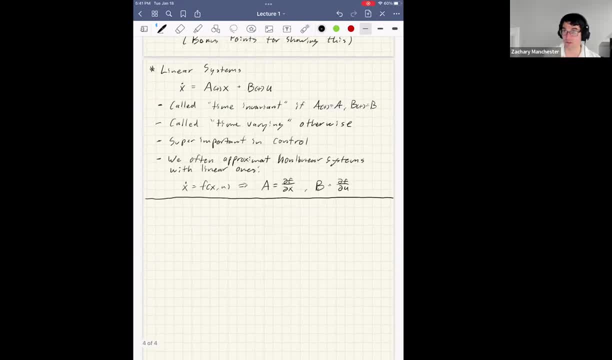 systems. there's a little bit more to talk about. we're going to dig in a little more now to some other stuff, but this is sort of the kinds of systems we'll generally talk about that you'll need to be aware of, and I can post some references on this stuff after. okay questions, speak up anytime. 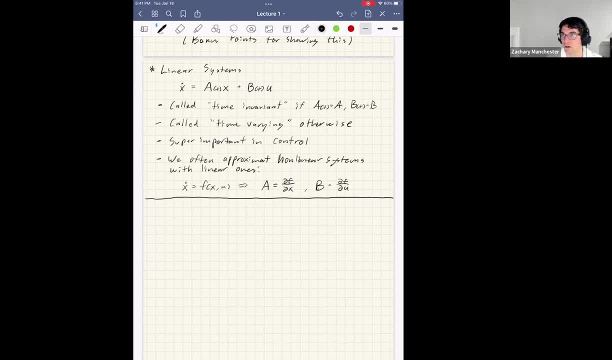 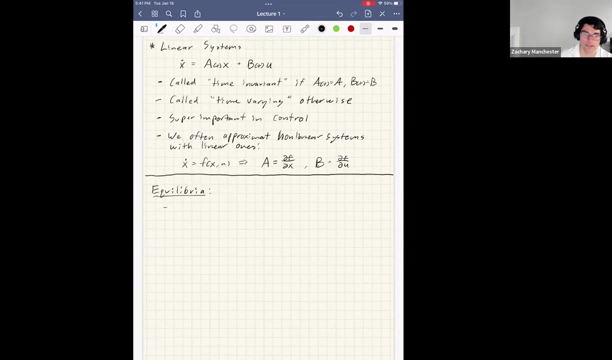 okay, so what we're going to talk about now are equilibria, so this is a, again, a pretty core concept in control, and so the the intuition for what this is. it's a point where a system will sort of remain at rest, and can anyone tell me what that looks like in terms of the dynamics, in terms of f of x, u? 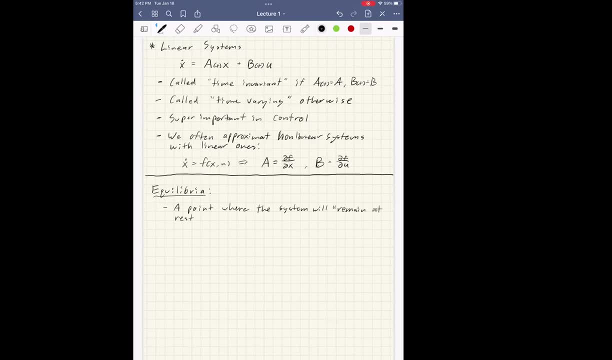 come on a geometrical function when it equals zero. yeah, thanks, okay, so that's right. so you know, remain at rest, not move. so you know, intuitively, then the derivative here needs to be zero. that's the definition of an equilibrium point. so algebraically we can kind of just look at this as a. 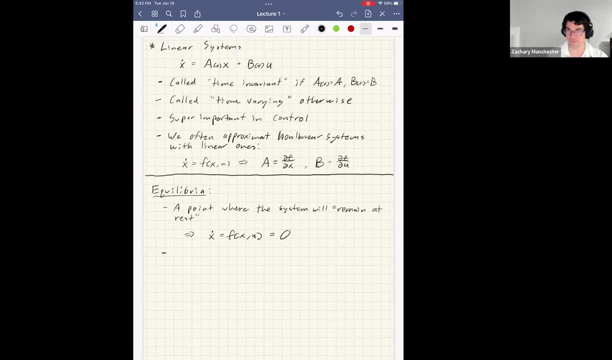 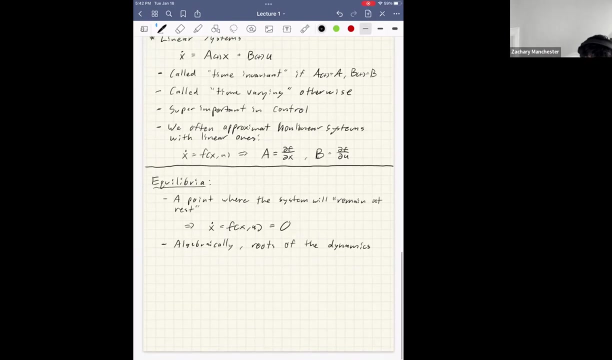 root finding problem. I just need to solve f of x, u for zero, and if I can do that, if I can find a zero of that function, here we go. I've got an equilibrium point, All right, So let's go back to our pendulum again. 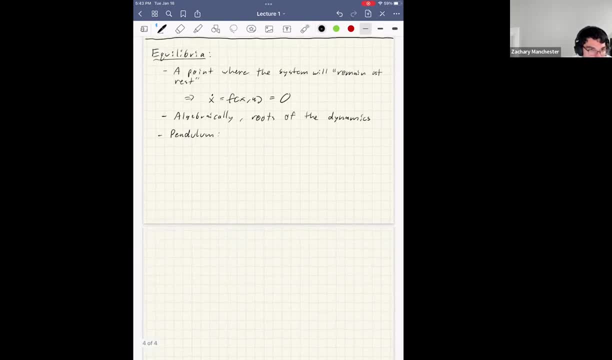 So if we write those dynamics down one more time, We've got theta dot, then minus g over L, sine theta. So this will just deal with the uncontrolled dynamics for now. And we want to set this all equal to zero, So the top part's easy. 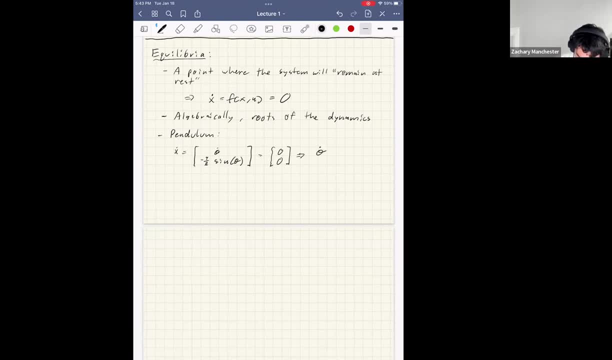 Theta dot equals zero, velocity zero. That's sort of a no-brainer. How about theta? What does theta need to be here for this to be have an equilibrium point? This is pretty intuitive. also, Pi over two. So it depends how you define your angles, right? 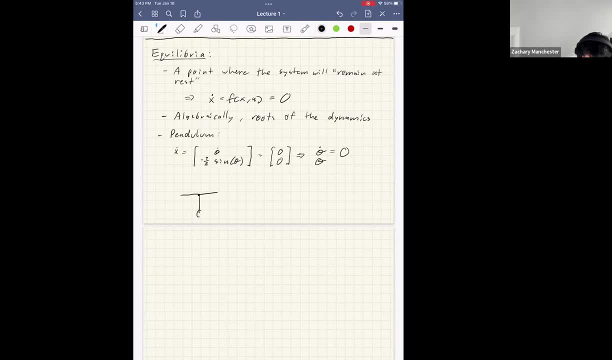 So the way I defined them before in the picture, this is this: is theta equals zero Right? So sine theta, sine sine theta, you know, sine of zero, zero right, And there's one more. So where else does sine theta equals zero? 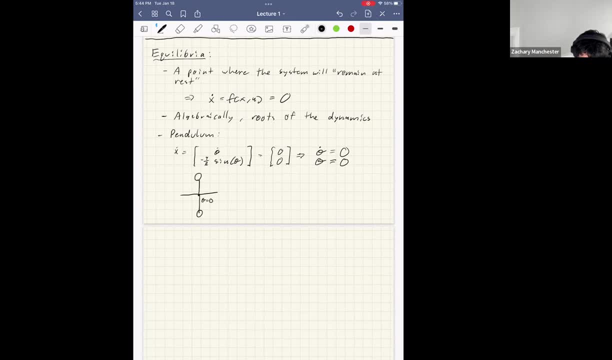 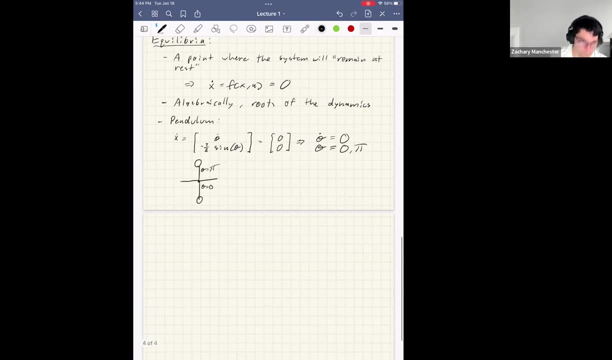 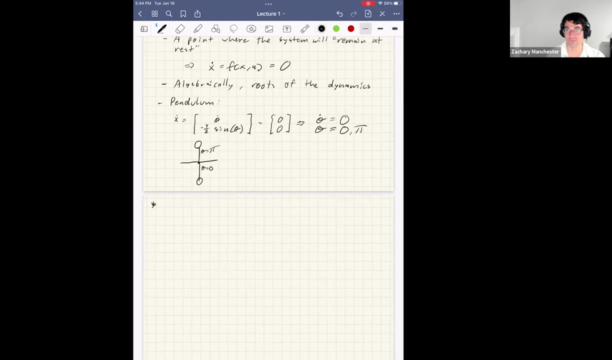 So right up, right pi. So we've got zero and pi. So there's kind of two equilibria here, Okay, So now we're going to do our first control problem. So now I'm going to look at this with the. 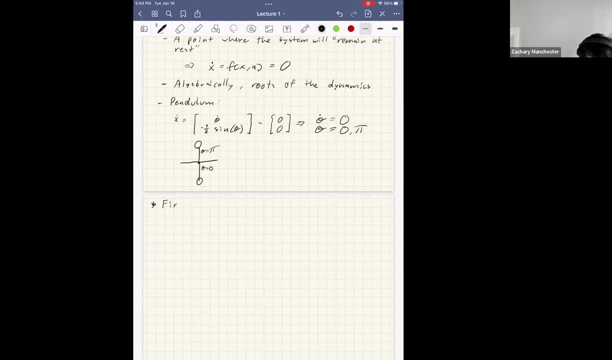 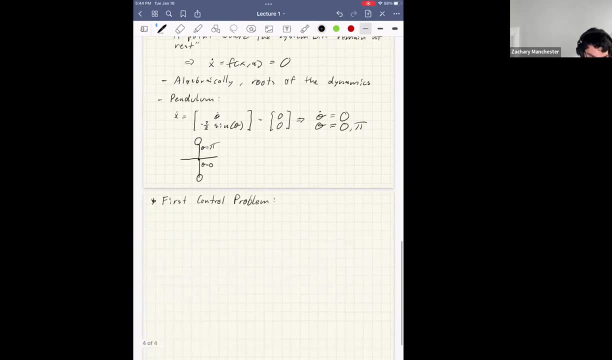 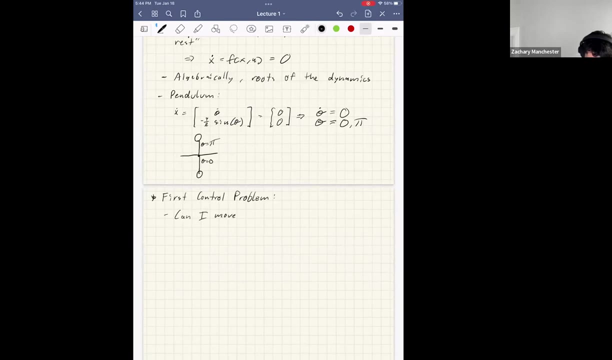 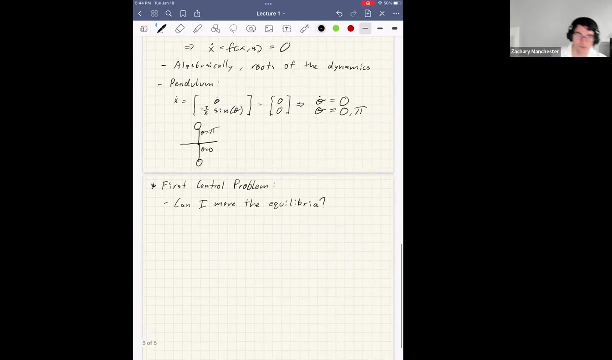 with the control torque in there, Okay. So question: can I move the equilibrium points? So what do you think? Can I? so here's: yeah, We can by applying some input. Yeah, that's exactly right. So what I'm going to ask now is: let's try to put it at. 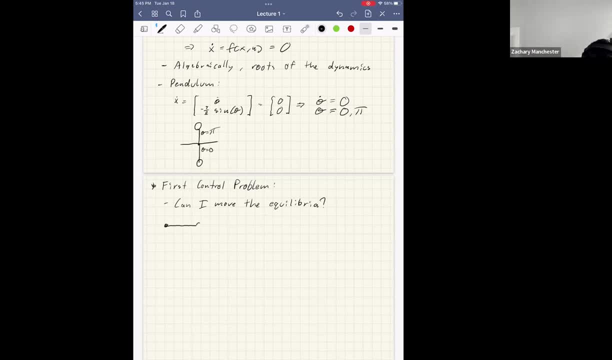 say pi over two. Let's try to put it straight out here. So now I'm going to write the dynamics with the torque input And I'll take a look. So here we've got a theta dot which we want to be zero. 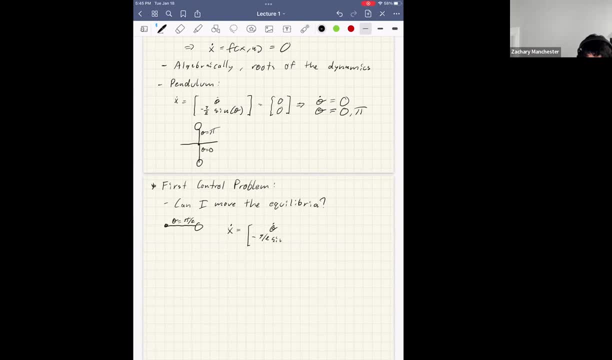 And we've got minus G over L sine, So we'll put pi over two in here. And then we've got the input torque, So we need the this whole thing to be zero, right? So velocity is easy, but I need to solve that second equation now. 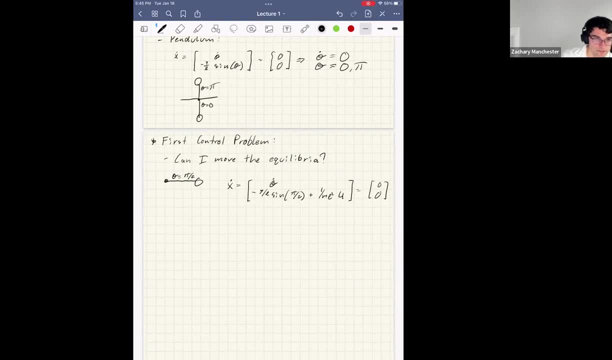 For zero right. So if I kind of just go ahead and do that, I get. I get one over ML. squared. U equals G over L sine pi over two. Pi over two is obviously sine, pi over two is one. So this tells me that U equals. 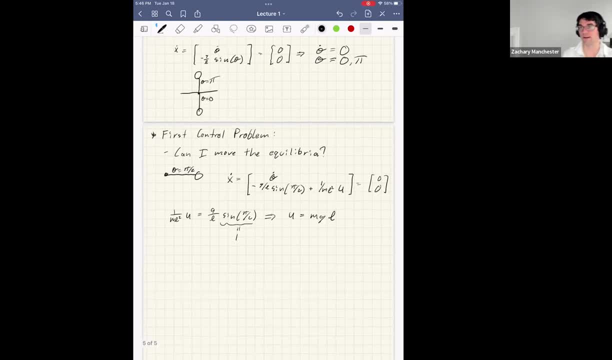 MGL. And so I mean this is super intuitive right? I'm basically applying a torque that's going to cancel out gravity at that position, right, I could make this wherever I want, right? So with this trick, I can plug in any theta I want. 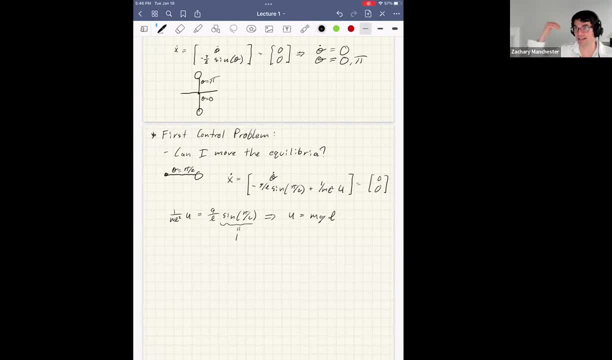 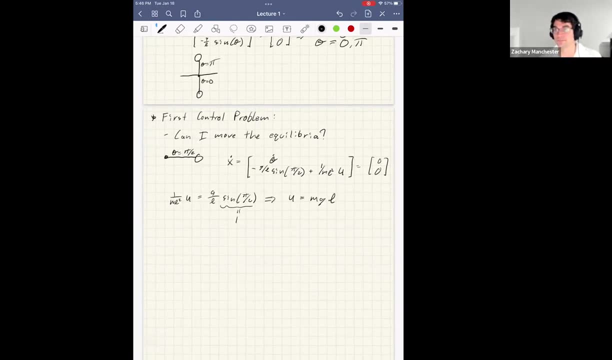 solve that equation for U and get an equilibrium and move it anywhere. I feel like right. I have a quick question. Yeah, So in this case, what this? the interpretation of this would be that like if, let's say, the pendulum was at theta equals pi over two already. 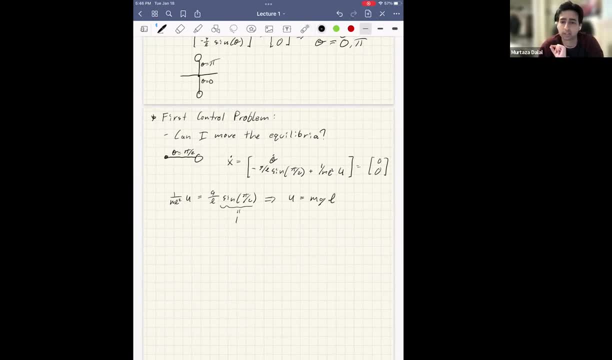 and then you want it to hold it there, then you'd have to apply this U, but it wouldn't necessarily get you to that equilibrium position. That's right. So what this is saying is: if I want this other point to be in equilibrium, 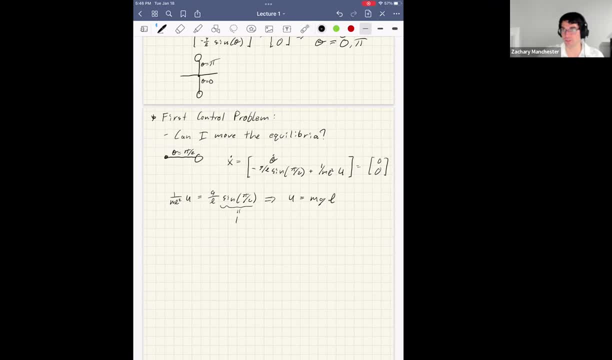 to be a place where the system will hang out if it starts there. this is what I need to do, right? It doesn't say anything about how you get it from some arbitrary point to there. That's sort of: yeah, we're going to talk about that for sure. 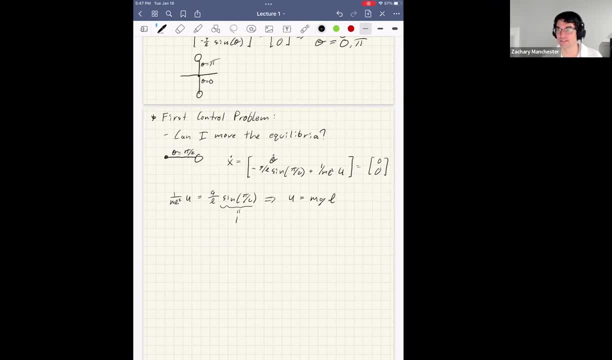 But yeah, this is kind of one of the core core ideas. So it's like if I want to drive a system to a set point right, First I need to know what the set point is, and I may need to do some weird stuff. 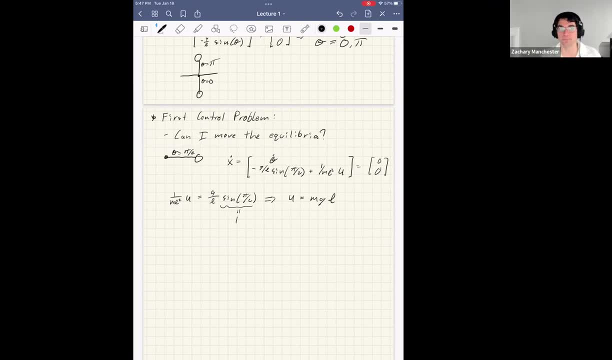 to create a set point that I like to drive it to right. Cool. So in general, right, we can just solve a root finding problem here in U. So so, given some you know, X star, that I want to be an equilibrium. 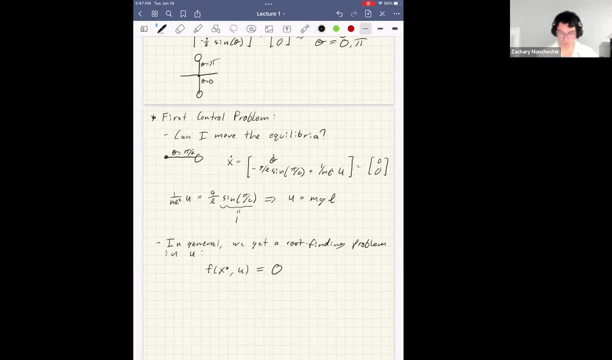 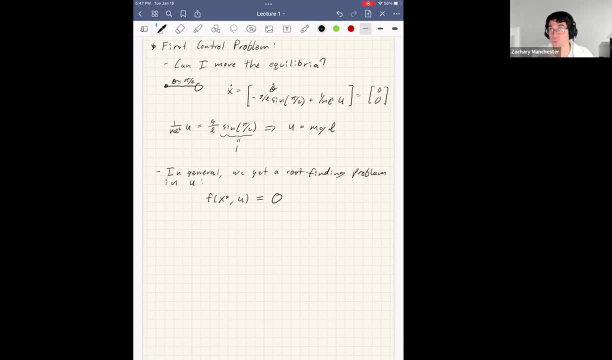 I can plug that in to the dynamics, set that equal to zero and just solve for for the U that makes that happen. I can't always do that. It depends on the dynamics of the system. For the pendulum, I can always do it. 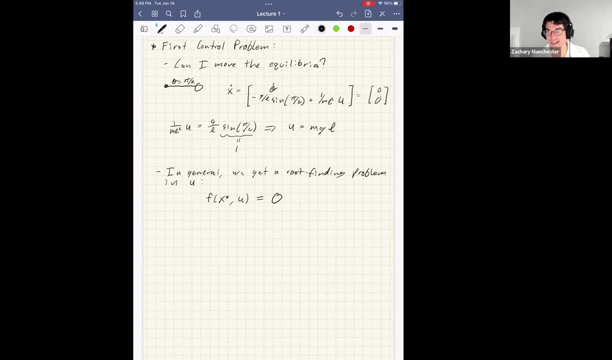 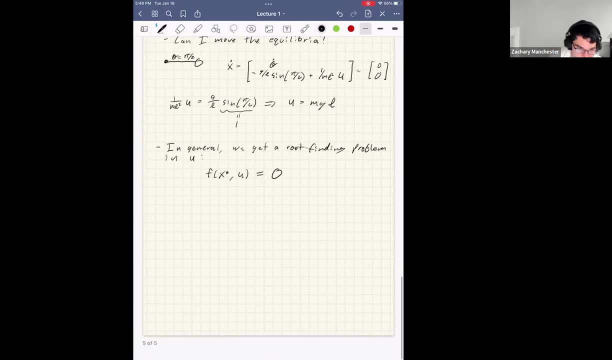 In general, if the system's fully actuated- ie I have as many control inputs as I have degrees of freedom- I can do this pretty much. It gets more complicated for underactuated systems. Okay, so that's equilibrium point. 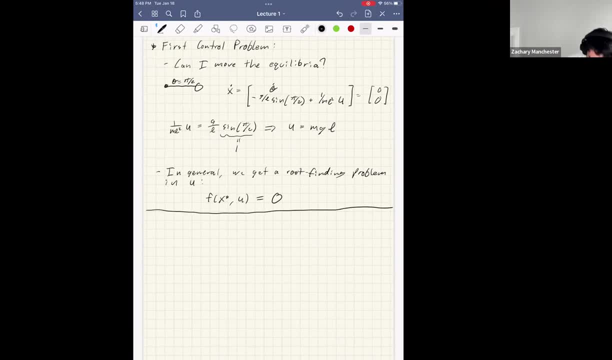 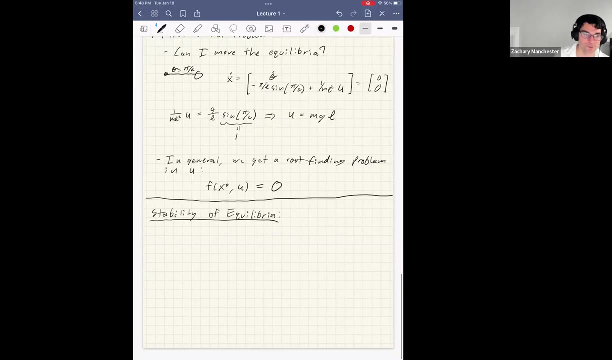 or equilibria as the plural. So the next thing to talk about is stability of equilibria, And this is kind of starting to follow up on the question that was just asked about, like how do you get there, et cetera. 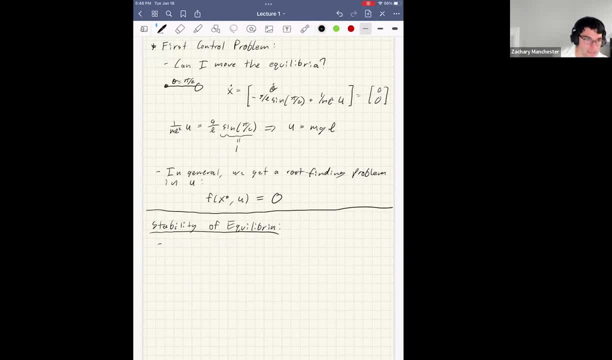 Okay. So the idea we want to get at here is: if we start out near an equilibrium point, will we stay near it under, say, small perturbations? So that's kind of the question: When will we stay fuzzy near an equilibrium point, say under like small perturbations? 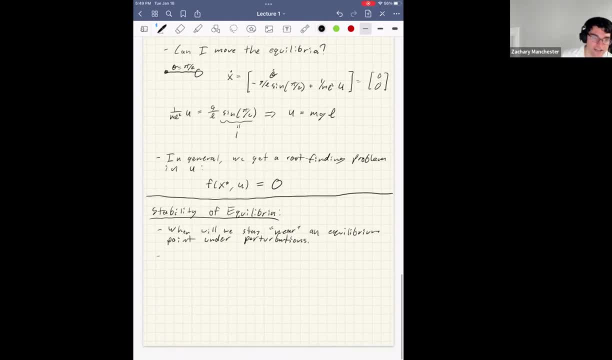 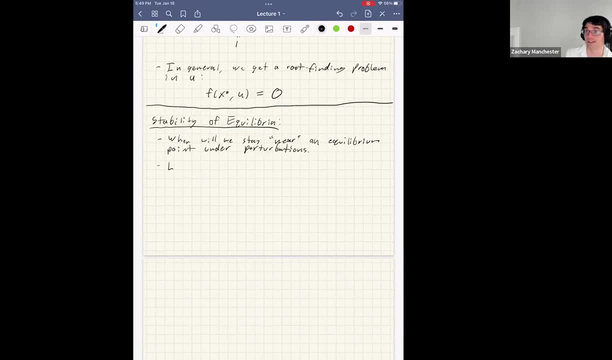 And to get at this, we're going to look at a super simple way to do this. It's a 1D dynamical system. It will be a nonlinear system, but a 1D system, And here I mean 1D. the state space is 1D. 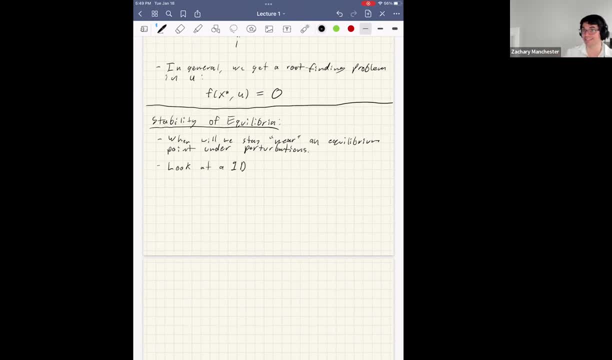 So the pendulum, it has one degree of freedom. the configuration space is 1D, but the state space there is actually 2D, right, because the state has theta and theta dot Here. I mean the state is 1D. 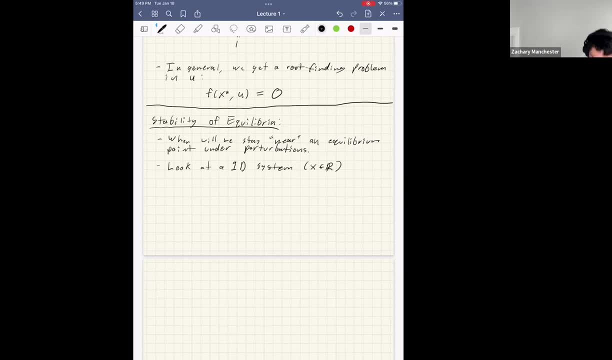 So these are kind of interesting In that we can basically understand everything there is to understand about 1D nonlinear systems, which is kind of cool. So here's a- I'm going to draw a 1D nonlinear system where the x-axis is going to be x. 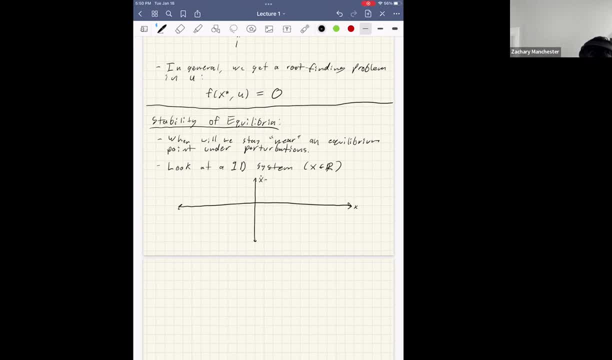 and the sort of vertical axis here is going to be x dot, which is our dynamics right f of x, And here there's no control, It's just an autonomous system And I'm going to draw sort of the dynamics function. 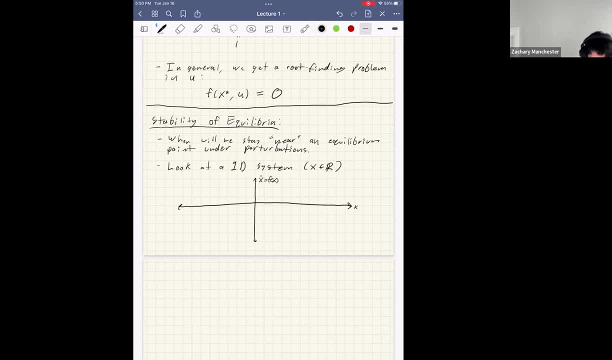 Let's say it looks sort of like a cubic, maybe It looks like this. So let's say that's our dynamics function And you can think of this like some weirdo. you know cubic polynomial or something like that. So first question is: where are the equilibrium points? 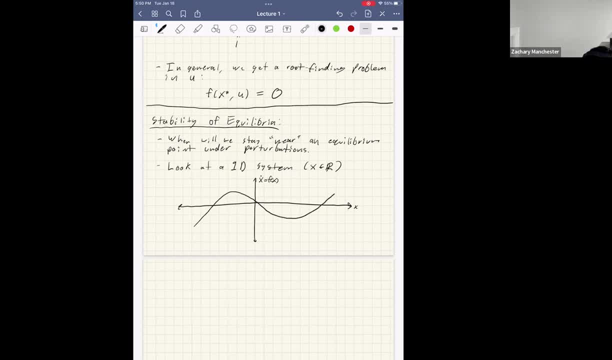 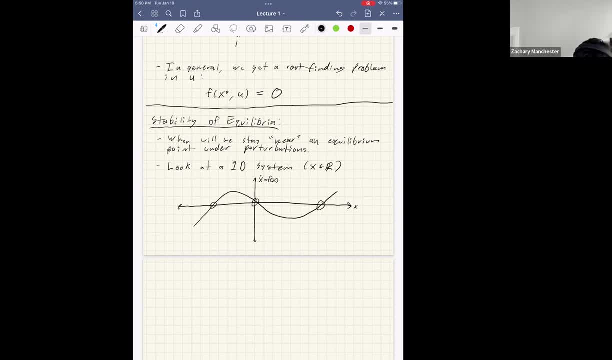 Exactly. So we got three equilibrium points at these zero crossings. So next question, let's look at the one at the origin here. So and keep in mind, right like x, dot is the vertical sort of axis. So if I get pushed a little tiny bit to the right in this picture, x dot is negative. 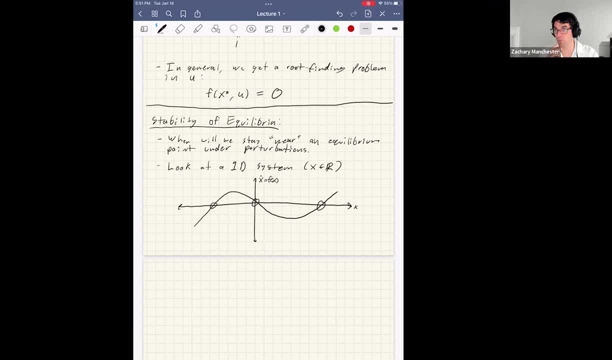 That means I'm going to sort of drift back towards the equilibrium point, right, So I'll draw this. So if I get pushed a little bit to the right, Yeah, right, I'm going to end up getting. the dynamics are going to naturally nudge me back to the left. 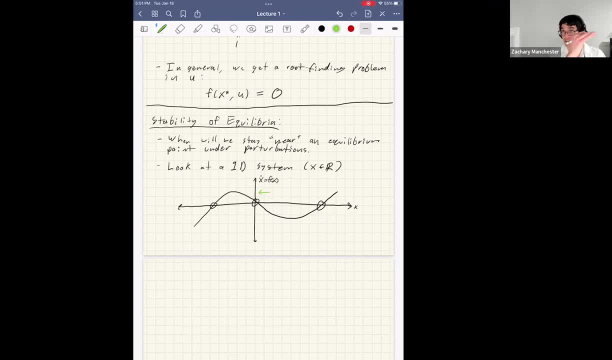 and vice versa. if I get pushed a little bit to the right, x dot's positive and I'm going to get pushed back. if I get pushed to the left, if I get perturbed towards the left, the dynamics will naturally push me back to the right. so I'm going to sort of naturally stay in the neighborhood. 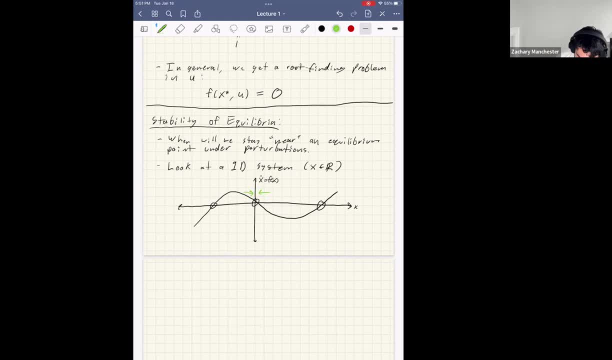 of this equilibrium point. so let's go look at one of the other ones now. so let's take the right one, for example. so in this case, if I get pushed to the left, x dot is negative. that means I'm going to go further to the left. vice versa, if I get pushed to the right, x dot's positive, I'm going. 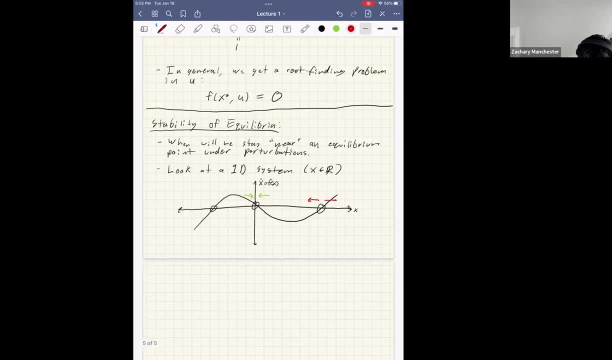 to go go further to the right. the dynamics are going to carry me sort of farther away. and then same thing on the left one: if I get pushed left, I'm going left, if I get pushed right, I'm going right. so, looking at this very intuitively, we say: 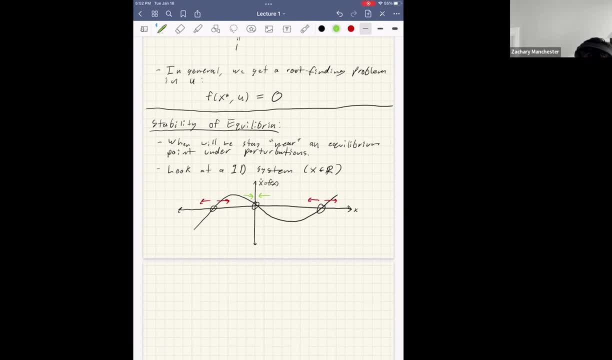 um, the middle one. here we say, this guy is stable, because under small perturbations the dynamics will sort of naturally kind of restore me towards the equilibrium point. and then the other two we say are unstable, because if I get nudged a tiny bit away from the equilibrium point, 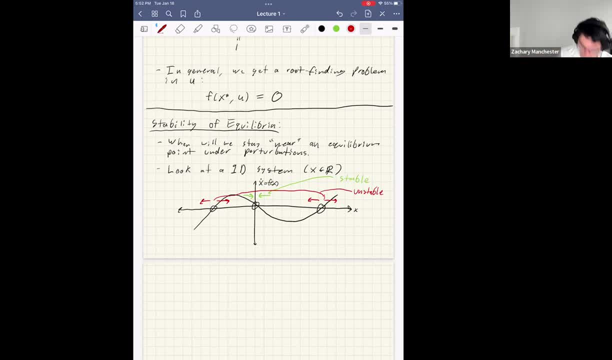 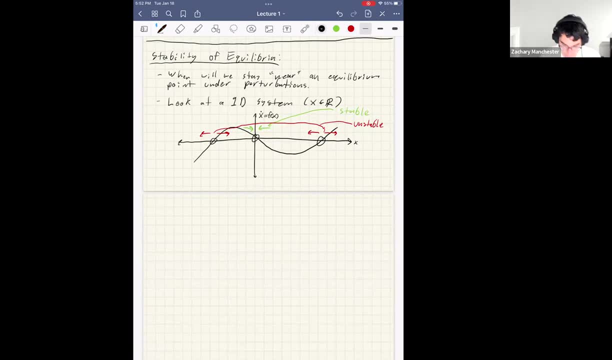 uh, that's it going um. okay, so any questions about that? does that make sense to everybody? cool? so, uh, we're going to now sort of like, take this really intuitive picture, um, and we're going to kind of generalize it to n dimensions almost trivially. so what we're? 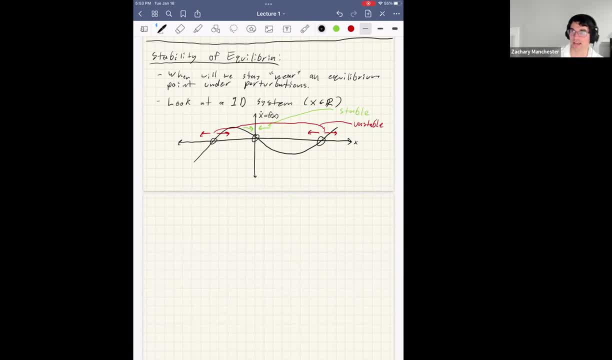 going to do is look at the slope of f of x, right? so what we kind of did here is we reason about um. is x dot positive or negative on either side? and we found you know how this works. so if we look now of f of x in the neighborhood of the equilibrium point, you'll notice in the stable. 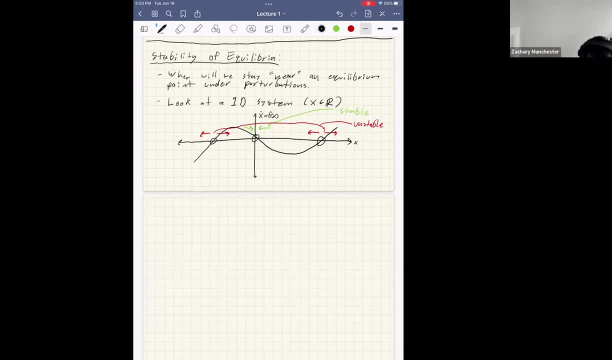 case the slope is negative. so partial f, partial x, negative implies that the equilibrium point is stable. and conversely, if you look at the unstable cases, the slope at the equilibrium point is positive, and that that implies that, uh, if you have partial f, partial x positive, you're going to be unstable, your equilibrium is going to be unstable. 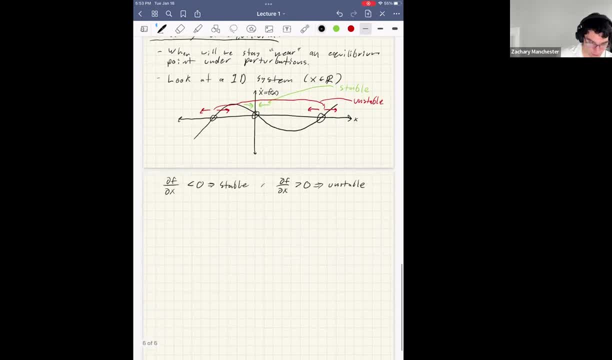 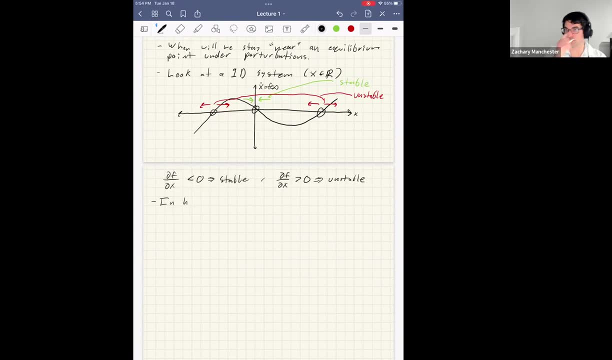 so that's coming just right from this picture that we just did. in higher dimensions. uh, we can still take these derivatives, but they're no longer scalars, they're just Jacobian matrices, right? so what do you think happens in higher dimensions? uh, so we get partial f, partial. 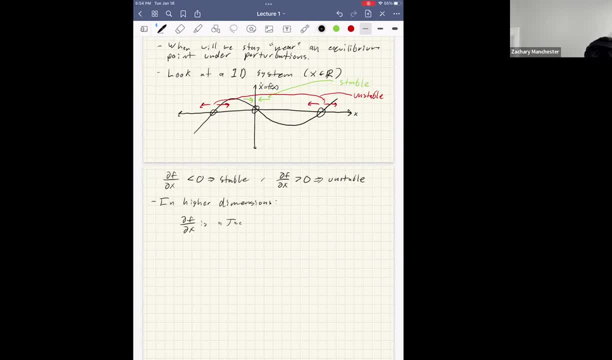 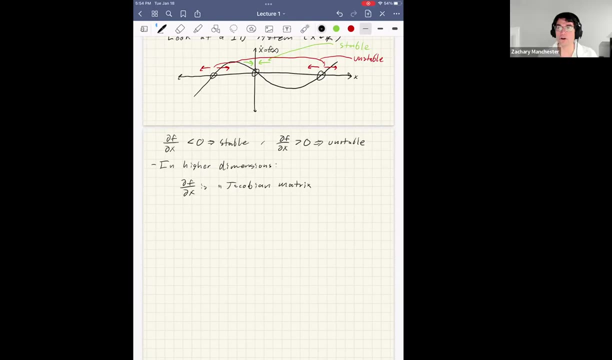 x. this is a Jacobian matrix, and so it's n by n. uh, where n is the state dimension. so it's a square matrix, and does it depend on the semi-definite definiteness? no, so, so that sort of property, that's um for a quadratic form, right, so that's a symmetric matrix we can, we can talk about. 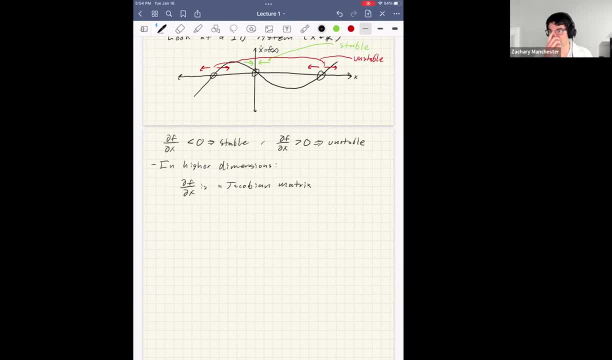 definiteness. this is not necessarily a symmetric matrix. um, this is just the- uh, the Jacobian matrix of some random dynamics function. so this, uh, we can't really say anything about the definiteness of this matrix and it's not a quadratic form, so that's sort of not the. 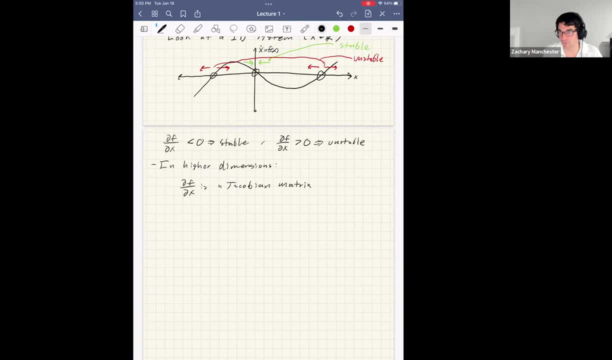 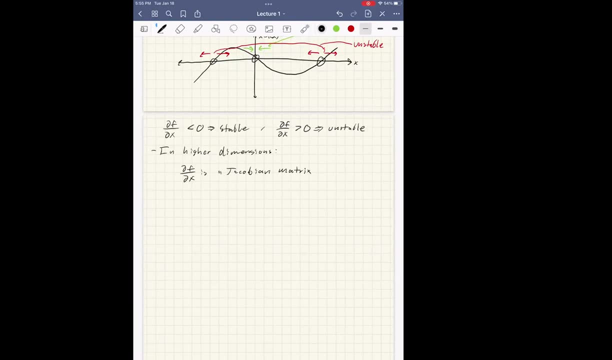 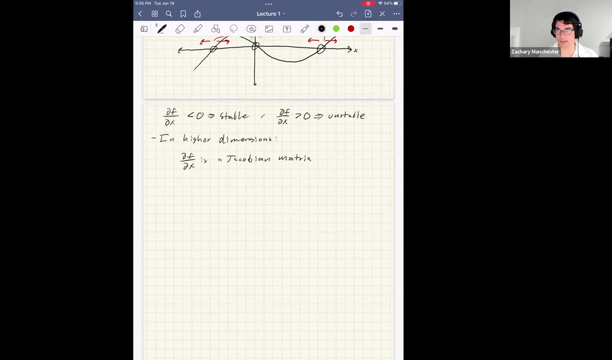 right thing to talk about. um, it's a linear, linear map, a linear function, um. so what we're actually going to do is we're going to take the square matrix and we can do an eigen decomposition of it, right, and what that's really doing, uh, is decoupling this, uh, this system, into n one-dimensional systems. 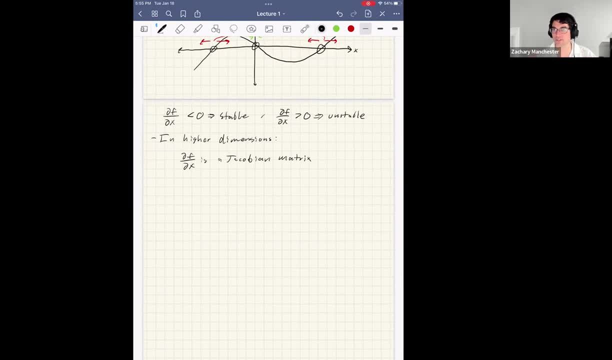 right. so if you think about an eigen decomposition, sort of geometrically, what it's doing is finding you a coordinate transformation such that that matrix is diagonal, and in this context, what that means is we're finding some funky coordinate transformations such that I've decoupled all 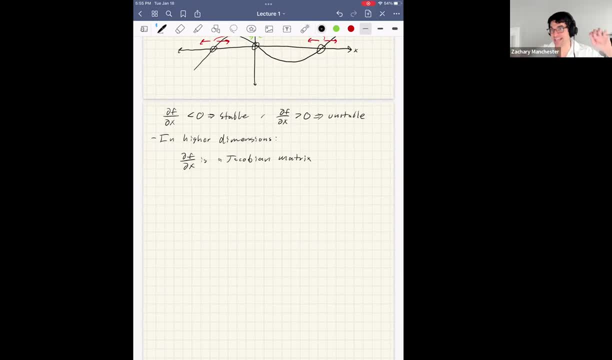 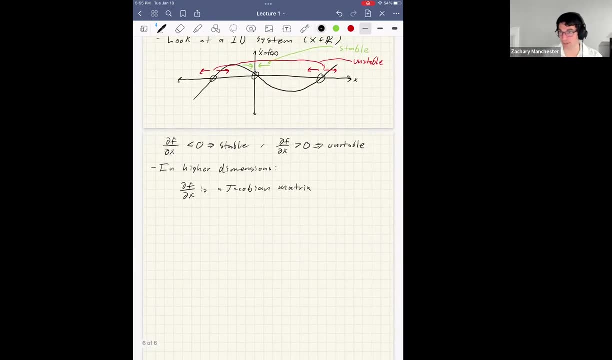 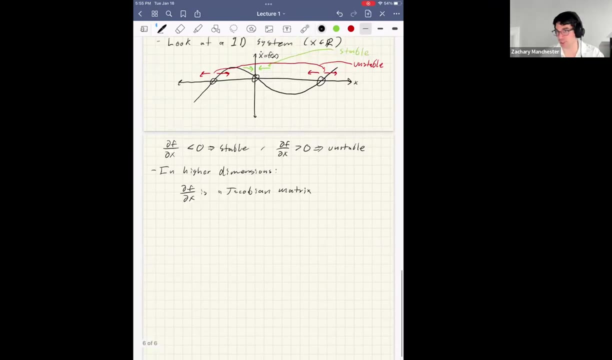 of the degrees of freedom of this system, and I basically just have n one-dimensional systems, and once I do that, I mean exactly this place again, uh, that I just drew the picture for. so the eigen decomposition is basically a trick for finding a clever coordinate transformation that puts us back in this 1d picture, and then we can apply the 1d result. so 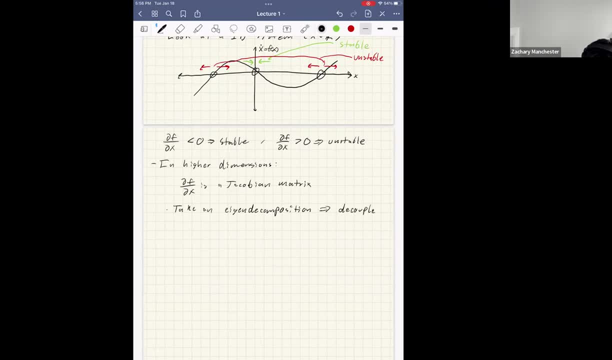 this sort of decouples us into n? 1d systems and then we um the n1d systems, right, the eigen values, are that the diagonal elements of that, uh, that matrix, and those are kind of telling us what each 1d system is doing and we can look at the real parts of 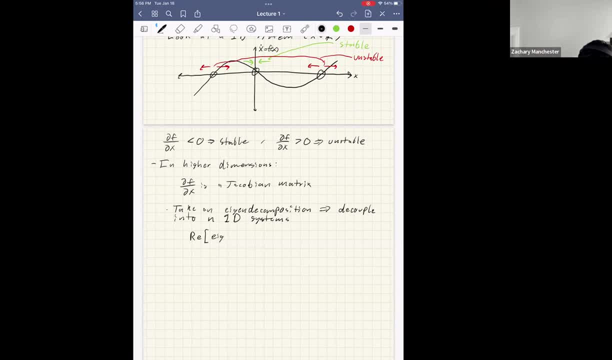 those eigen values it turns out. so we'll write it like this. so I take this eigen decomposition of my Jacobian, I look at the real parts of the eigen values. if they're all negative, this is saying like all n of those little decoupled 1b systems is stable. So then we can say that the whole system 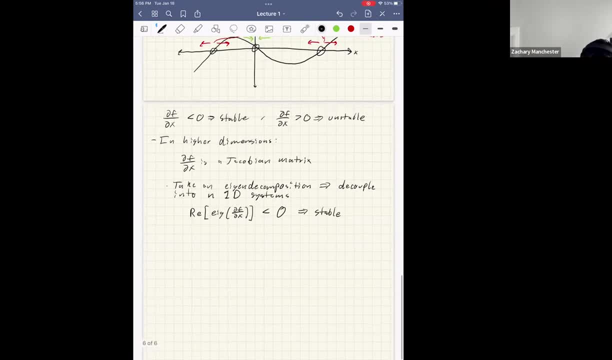 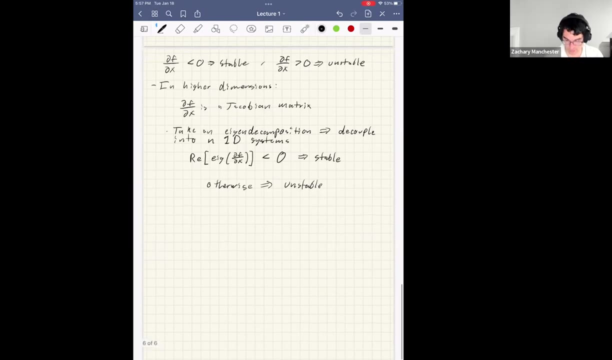 is stable and otherwise it's unstable. There's some subtlety in here, but practically speaking, that's sort of what you want to look out for Any questions about that. I know I did that kind of quick. I expect that most of you have seen this before. If you haven't seen this before, 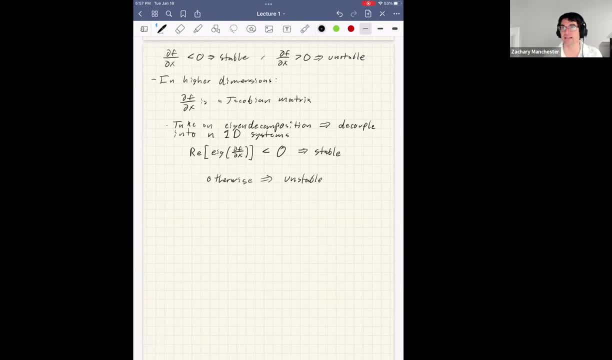 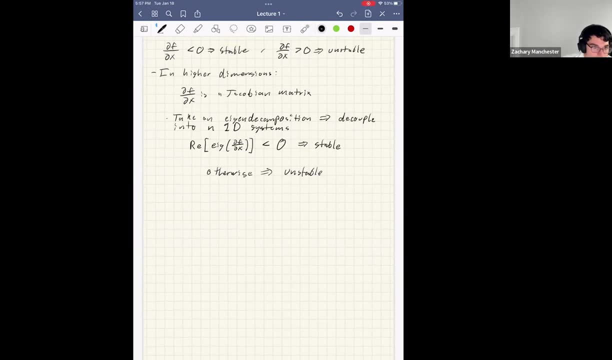 just send me a ping and I can shoot you some stuff to read, or we can talk more about it in office hours, But if there's any questions, though, don't hesitate to speak up. Okay, so now we're going to do this for the pendulum, And the result should not be surprising, So we 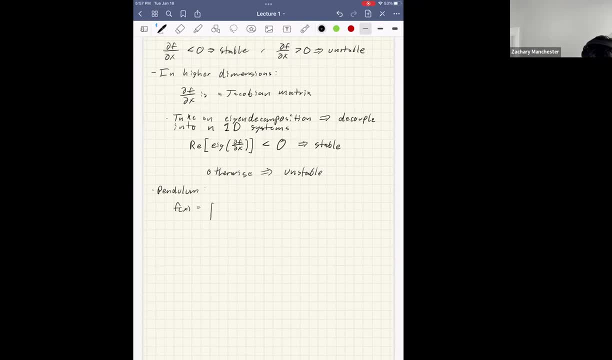 got our f of x theta dot minus g over L sine Theta. I can take the Jacobian of this partial f, partial x. This is going to be a 2 by 2 matrix, right, And that matrix. I'm just going to do this real quick by hand, So I do the first row. 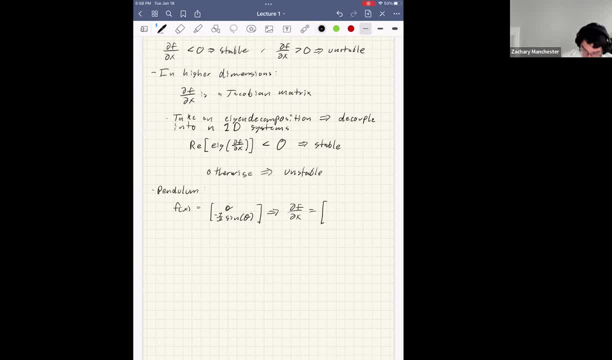 I take partial to the first row with respect to theta 0.. Partial to the first row with respect to theta dot 1.. Then we do the bottom row, partial with respect to theta. Is derivative of sine, is cosine, So it's minus g over L cos theta, And then partial to the bottom. 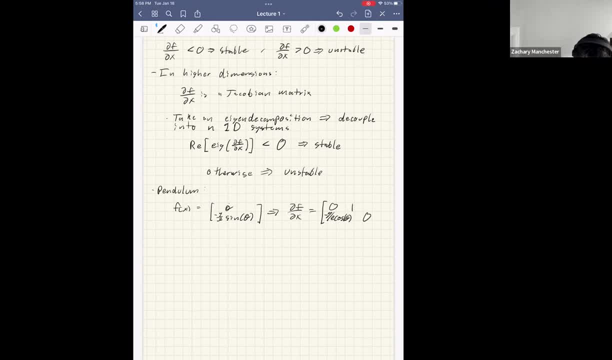 row with respect to theta dot is 0.. So I get this And yeah, just kind of following up on the previous question about positive definiteness, this is definitely not symmetric right? So they're sort of not sort of weird to talk about definiteness in that way for something like this. Okay, so now we've 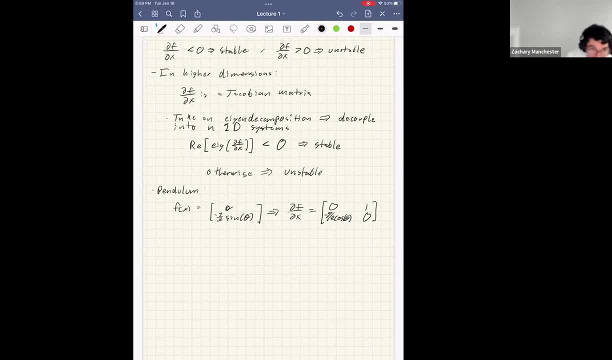 got our Jacobian and all we have to do is evaluate it at the equilibrium points that we want to check out. So let's look at the top one first. So we do, partial f, partial x, evaluated at theta, equals pi. If we plug that in, we get 0,, 1, g over L 0.. I can take the eigenvalues of this guy. 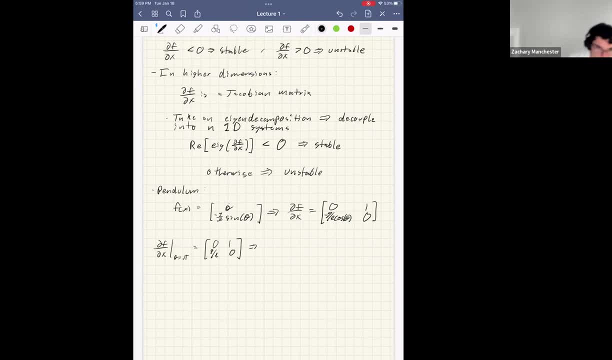 And for 2 by 2, it's pretty easy to do by hand or with a calculator. I'll spare you that. In this case it turns out this is plus or minus root g over L, And we check the signs on these guys right? So obviously this guy has a single positive. 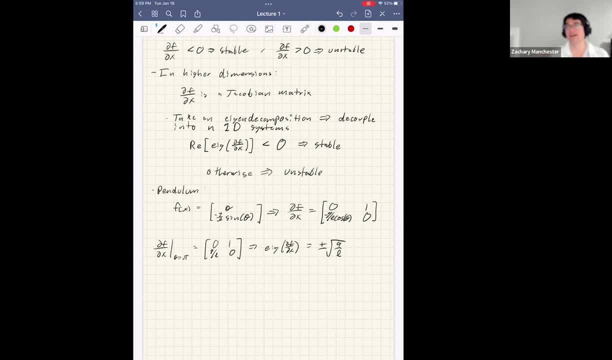 eigenvalue and a single negative eigenvalue And because of that, the positive eigenvalue means that we're unstable. So if we do the same thing for the other case, we're going to get a minus sign down here. And if I take the eigenvalues of this guy, 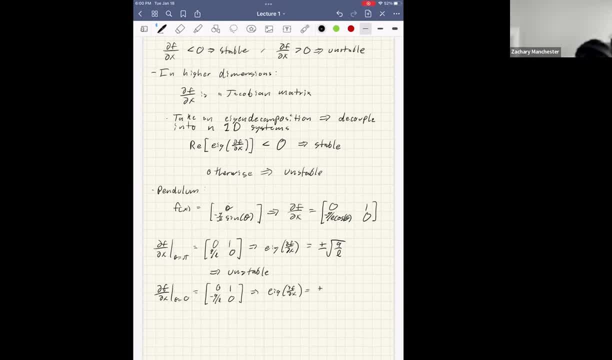 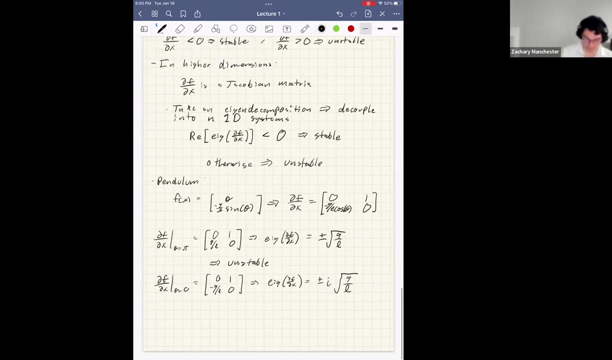 it turns out what I'm going to get is plus or minus i or j, depending on your persuasion. root g over L, And so this is pure imaginary, no real part. This is a bit of a weird case that we didn't talk about. 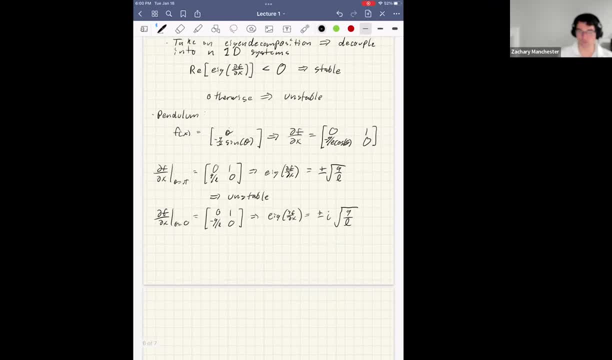 but now we're going to talk about it. So in the theory of linear systems we call this pure imaginary case marginally stable. Does anyone know what this means? like physically for the pendulum? No friction, It just keeps going back and forth. 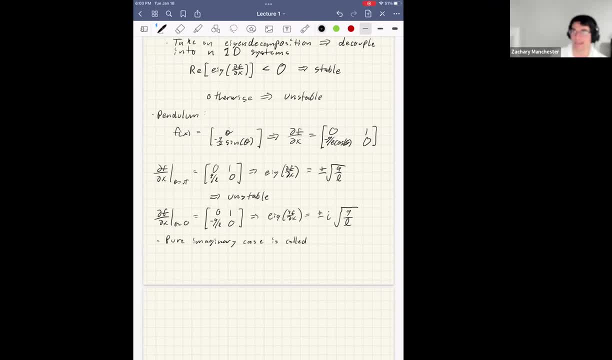 Yeah, it means that there's no damping in the system and that essentially pure imaginary eigenvalues correspond to oscillations, right? So this kind of means you basically have undamped oscillations and that things are just going to oscillate forever. 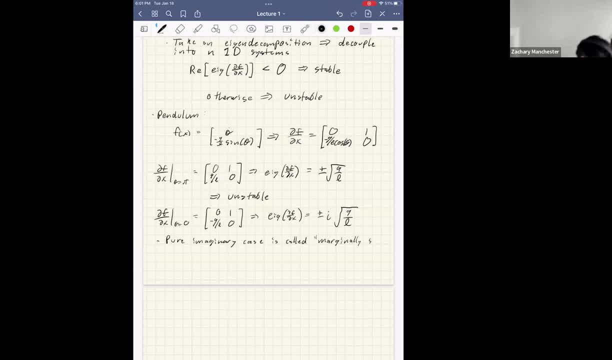 But there's a catch to this. So this is true in the linear case, in the linear systems case, But if we're doing this, if we're applying this linear analysis to a nonlinear system, what this means is that there's going to be higher order terms in the Taylor expansion that we're ignoring right here. 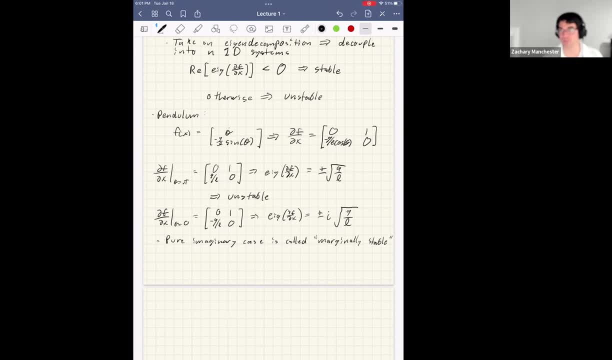 And if you've got, you know, if the first derivatives here, these eigenvalues, if these have zero real part, you can have these oscillations. But you've got nonlinear terms in there too And kind of all of a sudden you're going to have a nonlinear system. So you're going. 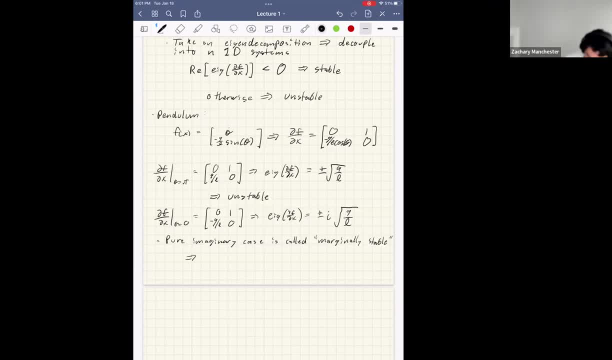 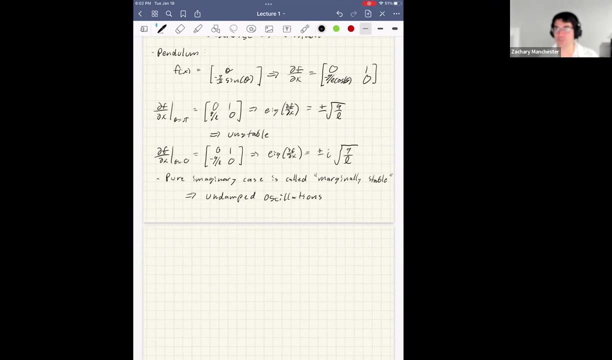 to have. all bets are off on those. So for a linear system you have this sort of marginally stable, undamped oscillations kind of thing. But if you're doing this on a nonlinear system, this is sketchy and you can't really trust it. It turns out for the pendulum here.